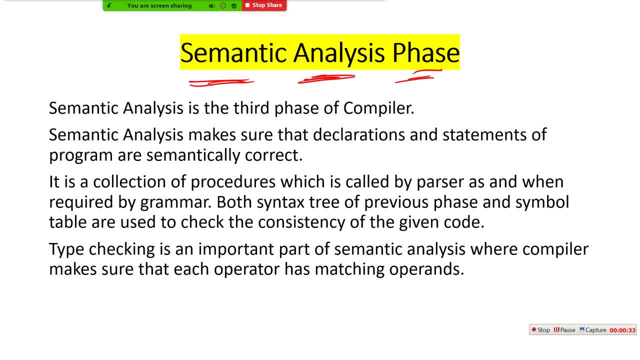 So semantic analysis phase. If I talk about semantic analysis phase, the very first point is: semantic analysis is third phase of compiler And I know that you all know about it, Right? So you can now assume that we have discussed lexical analysis phase and syntax analysis phase. Basically, these two consist of more than 70% part of GATE syllabus Right, More than 70, or you can say that at least 75% part of GATE syllabus Right. 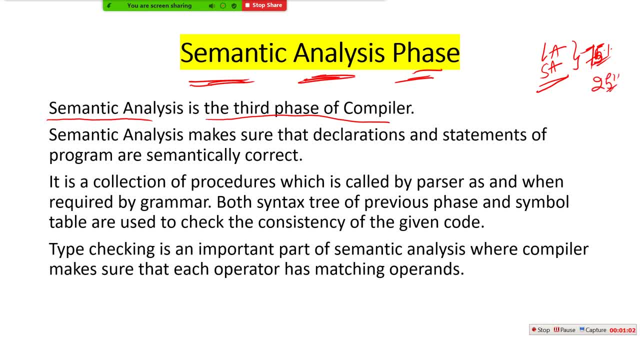 Right Left with only 25% part And in many times they may ask 100% from these two phases as well. But for the perspective of newly added syllabus and remaining topics, because in remaining topics theoretical points are more- You just need to focus on GATE perspective points, Right. You do not need to concentrate on subjective points, Right, Because there are more subjective theory in that, So we will just focus that what is important, Right? 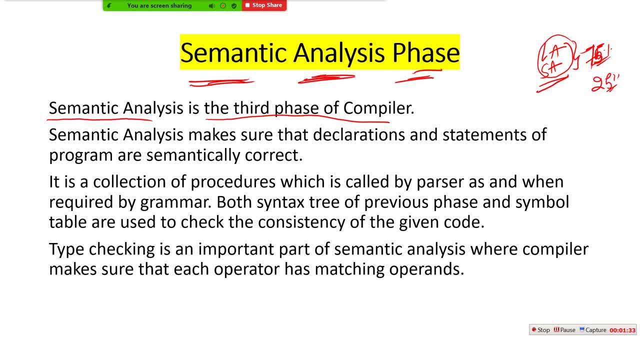 For us is of GATE syllabus Right. So it is a third phase of compiler and the semantic analysis make sure that declarations and statements of program are semantically correct. So what it makes sure, So semantic analysis phase will make sure that declarations and statements of program are semantically correct. The next important point is it is a collection of procedures which is called by parser, is and, when required, by grammar. 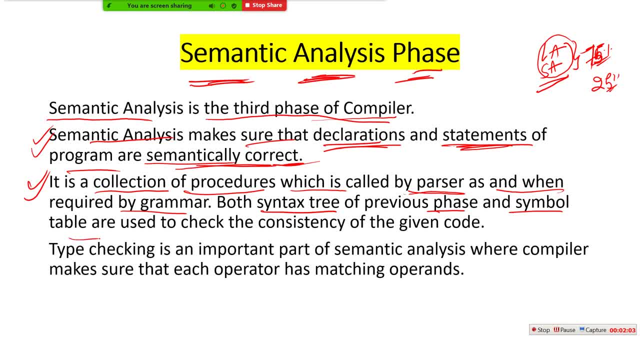 Both syntax tree of previous phase and symbol tables are used to check the consistency of given code Right. So both syntax tree and previous phase of symbols that is generated from lexical analysis and syntax analysis phase are used here to check the consistency of the given code. The next important point is type checking is an important part of semantic analysis where compiler make sure that each operator has matching operands or not, Right. But as of cylinder, each operator has matching operands or not Right. 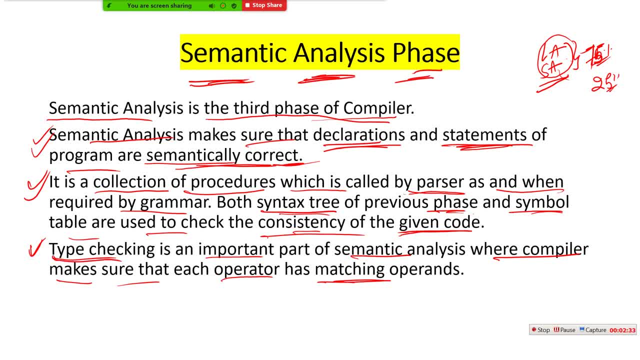 As of gale, each of them have matching operands. However, the gate is not asking much question on type checking Right. They is only asking questions on basics of semantic analysis. So we will only discuss the topic of semantic analysis as of here. 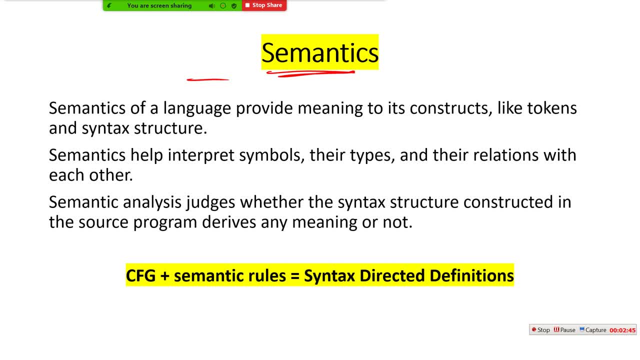 Now, if you talk about the terminology of semantics, that what is semantics? right? That if you generally talk in terms of definition or the terminology semantics, then semantics of a language. semantics of a language provides meaning to its constructors, like tokens and syntax structures, right? so whatever token you have taken from previous, 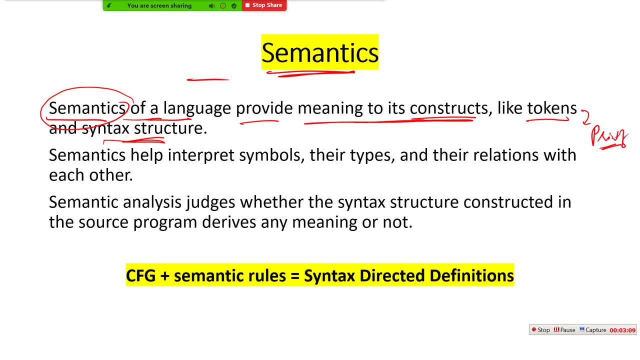 phase. suppose you have taken printf. suppose you have taken printf as a token from previous phase, so it will provide meaning to constructors that whether it is valid or not or like that, like tokens and syntax structures. suppose you have taken markup tags in your diary, so is it valid or not? suppose you have taken structures like that. so this kind of meaningful 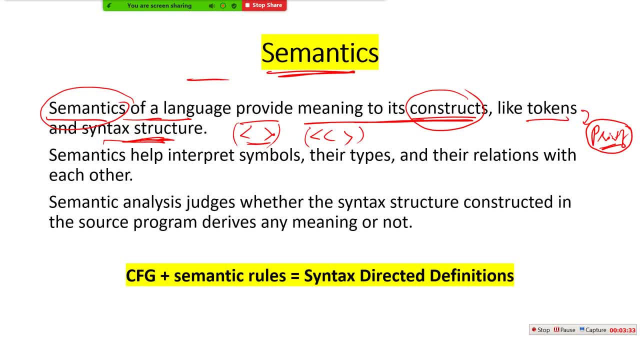 constructors would be check under that right and semantics basically help interpret. it will help in interpret symbols like, at the rate, hash dollar and their type and their relation with each other- that what is relation of this symbols with each other. it is the part of semantic analysis. we will discuss it with practical example so that you can. 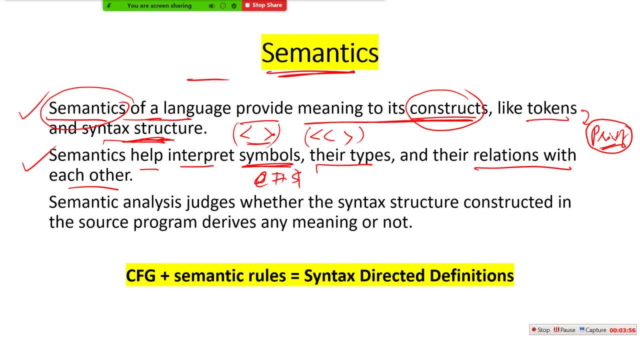 understand it very well. right here we are only discussing theoretical points. when we will come up with the real exam question of game, You will understand each and every theoretical points there. that what does it means right? and here our target is only to cover important theoretical points that may ask directly in. 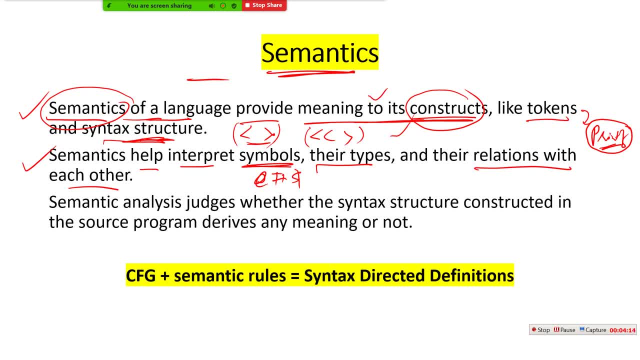 any of any of CS exam, because it is a very important part to discuss the theory. until unless we don't have knowledge of this simple terminology, we can forward proceed. so we are discussing that now. so next one is semantic analysis. so basically, semantic analysis judges that whether the syntax structure is valid or not, 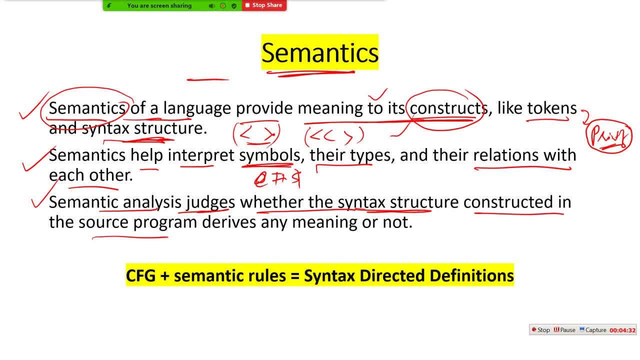 So we are going to talk about semantic analysis and that is where we are going to discuss the whether the syntax structures constructed in the source program derives any meaning or not. right suppose you have discussed if and forgot to close the rightmost braces. so it will judge that whether the syntax structures are meaningful or not. now, if we talk about simplest terminology of semantic analysis phase or the SDT, that is, syntax, directed translation, you can say it is the combination of CFG plus semantic rules, means 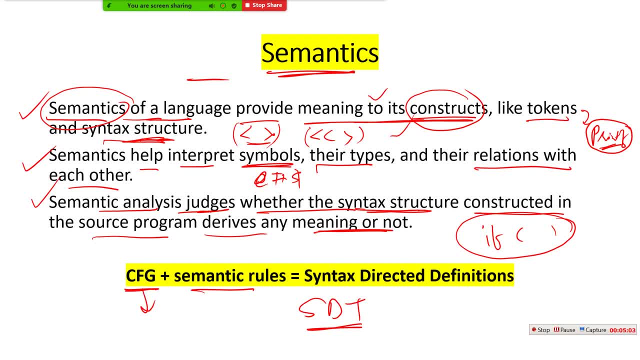 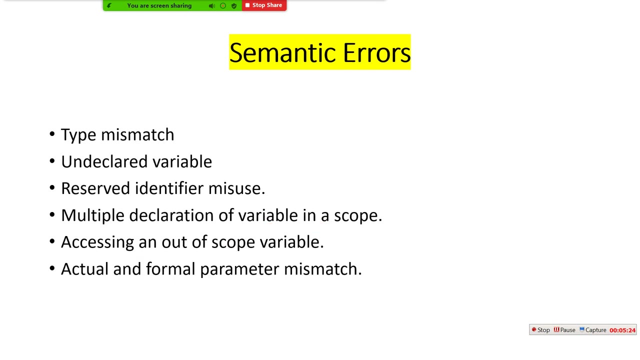 context, free grammar would be there and after each transition in the right hand side you will get some semantic rules. on the basis of the semantic rules we will apply the semantic rules on grammar and combination of CFG plus semantic rules are: say, are can be said as a syntax directed definition, as SDT. now there are some important, important types of semantic errors. you just need to know. 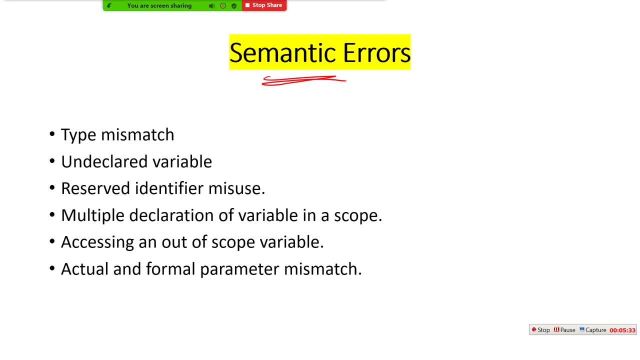 it only is of perspective, of knowledge. GK right, no using gate, but just need to know. it is a knowledge perspective that what are semantic errors? type mismatch is one of a semantic error. undeclared variable is a semantic error. so suppose you have discussed int i, j and k and suppose later you are using terminologies f, that is, f equals to 10, but you didn't declared f in earliest of program. so such kind of 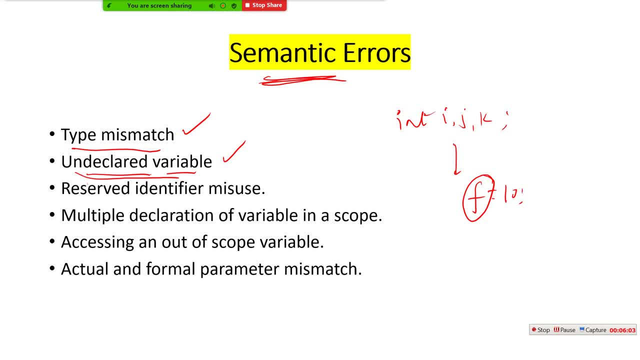 undeclared variable is a part of cement semantic errors and the next one is reserved identifier misuse is also part of semantic error. if you are misusing any identifier on unnecessary places, it will be detected under semantic errors. and if we talk about multiple declaration of variable in a scope, if you will declare multiple declaration of variable in a scope, right. if you are declaring int i, again you are declaring int i. or suppose you are providing? 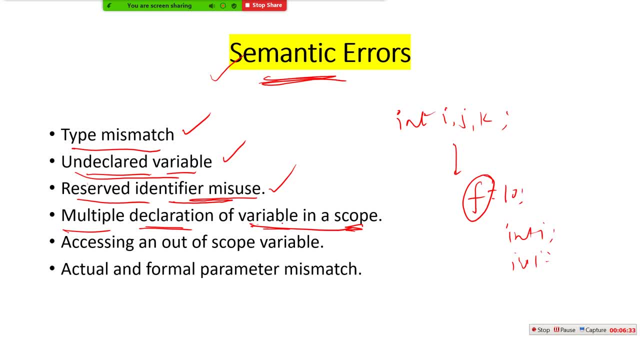 values to it. so if you will multiple declare, declare our variable in a same scope. it is also part of semantic errors. and next one is accessing an out of scope variable. suppose, in our scope we are only able to get i or j, but we are trying here to accessing some other variable, like k, which is not a part of this scope. then it is. this kind of errors is also termed under semantic errors. and next one is actual and formal parameters. so i hope you have learned. 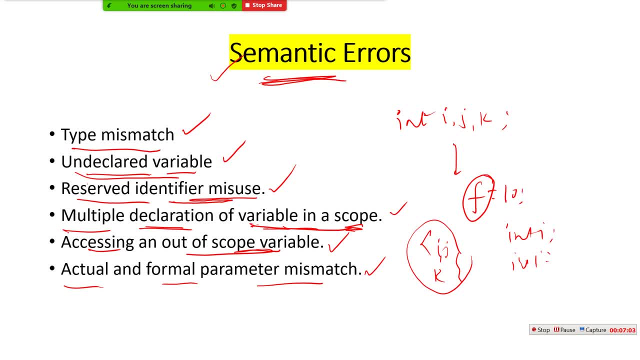 what is actual and formal parameter in call by reference and call by value in part of basics of c programming. so this is also placed under semantic errors. so this is the general knowledge point of semantic errors, right, you just need to know it as a point of g, k, right? no, using get example, but at least you need to know it so that whenever we talk about this terminologies later, you will get it now, let it, let it take. 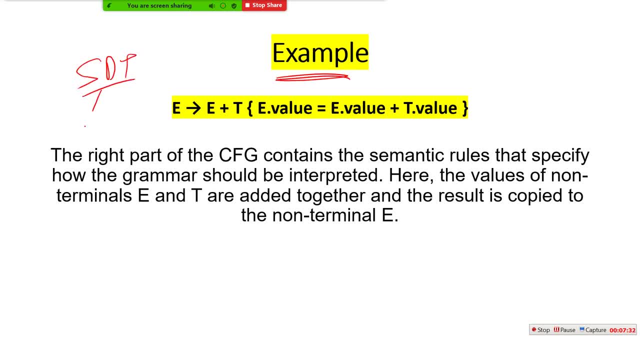 example? so it is an example of SDT. what is SDT? it is a combination of CFG that is a grammar, is there? it is a CFG, context-free grammar plus semantic rules, plus semantic rules. so this is the semantic rules. now, what semantic rules is telling us? focus here the right part of CFG, that is, this part, this. 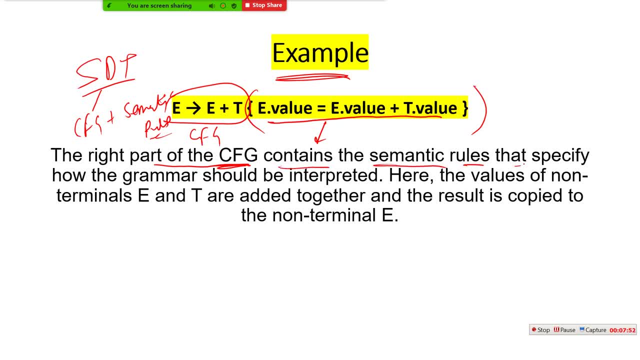 is the right part. it contains the semantic rules that specify how the grammar should be interpreted. how the grammar should be interpreted means this grammar, this grammar, should be interpreted with this rule. okay, here the values of non-terminals E and T: here the values of non-terminals E and T are added together. are added together in. the result is copied to: here the values: 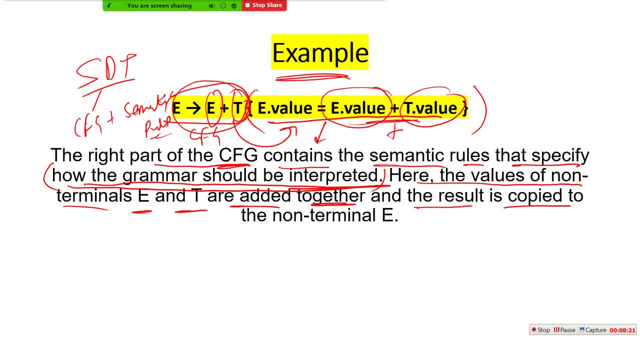 of these non terminals are added together and result will be get copied to non terminally. result will we get get added to this non-terminal e, non-terminal e, right? so this is the basic, first example of our sdt, that is, syntax directed translation. now, guys, i am presenting a very, very important question in 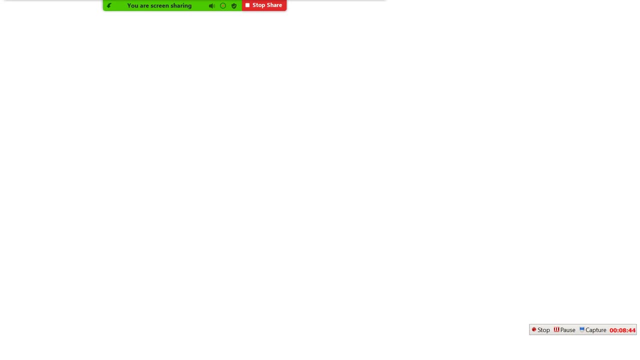 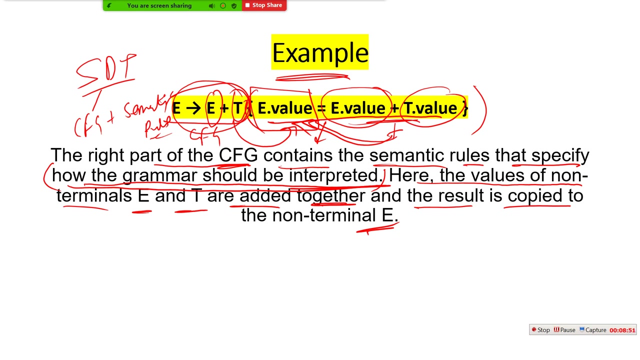 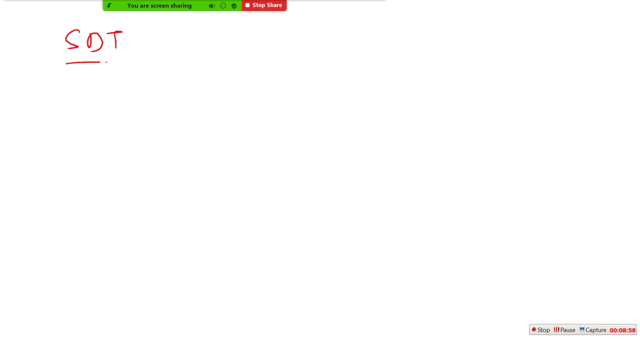 front of you. first we will see. first we will see that how sdt can be created, and later i will give you examples in real get scenario and you will solve that right. so if, uh, initially i am writing one sdt here, one sdt here, and my sdt is e derives e plus t, this is my cfg. this is my cfg. now i need. 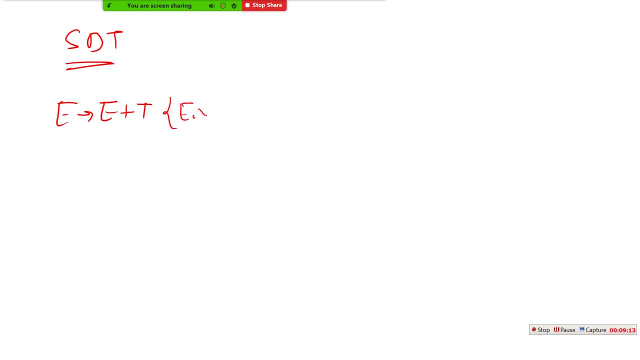 to write semantic rules. semantic rules are: e dot value equals to e dot value plus t dot value. so this semantic rules is telling me that here, in this grammar, i need to add. i need to add the value of this e with this t. i need to add the value of this e with this t. 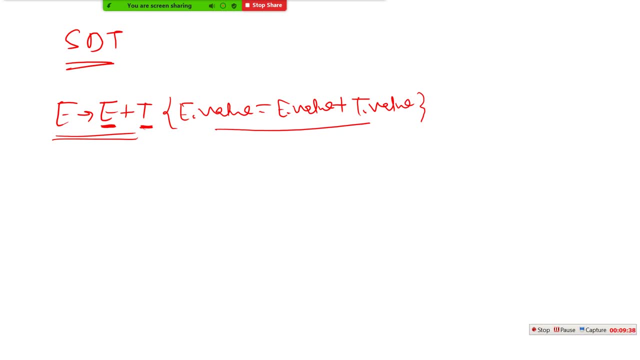 this is my semantic rule, is telling me. so this is a one sdt transition. one more sdt transition is e, also deriving non-terminal t, and here we can simply say that e, the value of e, that is, e value is t value, e value is t value. okay, this is the simplest transition. the next: 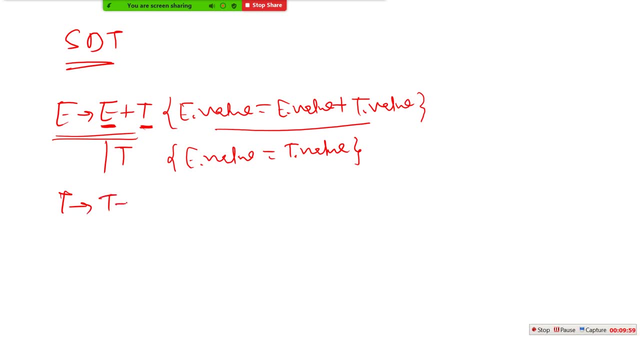 transition is: t derives d derives t star f, and what i need to do here is that this t value, this t value, is equal to t value. that is, this t value multiply with this f value, multiplied with this f. so basically, semantic rules are telling me that what i need to do, semantic rules helping me to do. 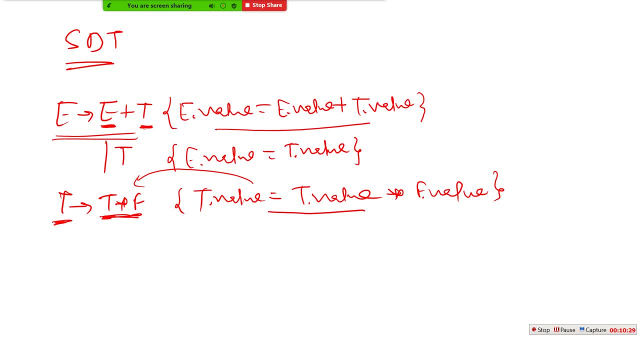 whatever written in the grammar, so it is a part of sdt. that is why whatever we need to do in cfg, whatever we need to do in cfg are- i am getting from help of semantic rules- okay, and t is deriving one more transition. that is small, that is a non-terminal f, and in that i will write that t value. 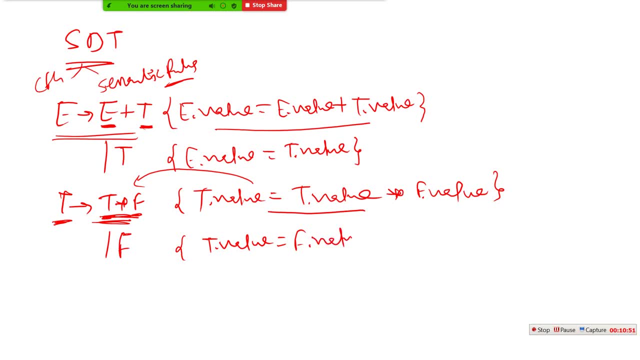 equals to f value. t value equals to f value, and at last i am getting f derives num, that is, a numerical part, num that is. so it telling me that the value of f, f value, equals to num, dot l value. l value means whatever the exact value of num. we will replace this f with that num value, right so? 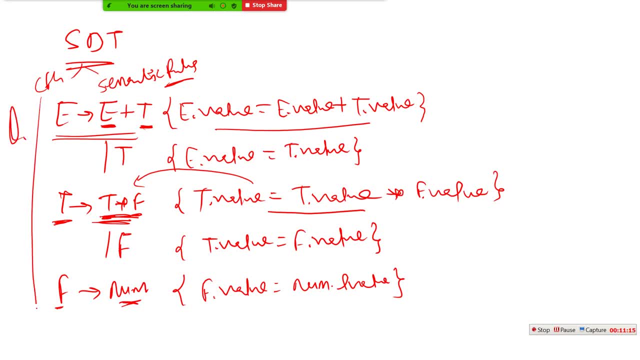 this is sdt. this is a question that this is sdt given to us. suppose this is the sdt given to us, okay, and what we need to do? suppose we need to apply. we need to apply our concepts on this, our concepts on this, and we will. we need to parse it so sdt can be parsed from bottom to up. 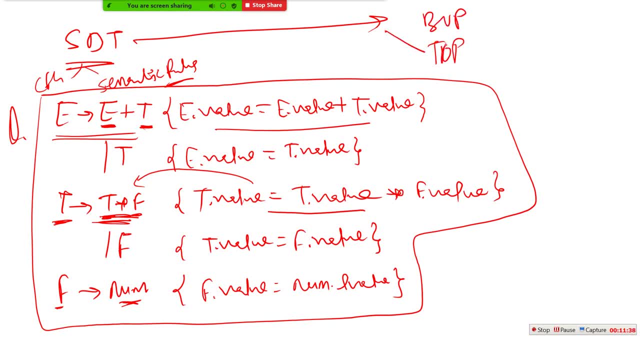 and it can also part top down right, so it can also. it can also be parsed using bottom of parsing technique and it can also be parsed using top down parsing. it generally parses from bottom to right, according to the question. so suppose my question is if i need to. 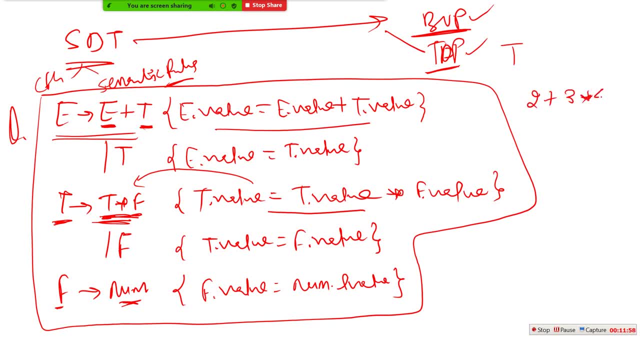 i need to traverse. suppose my string is suppose 2 plus 3 into 4, 2 plus 3 into 4, it is my string. it is my string 2 plus 3 into 4 and i need to parse it. i need to parse it using using top down parsing. 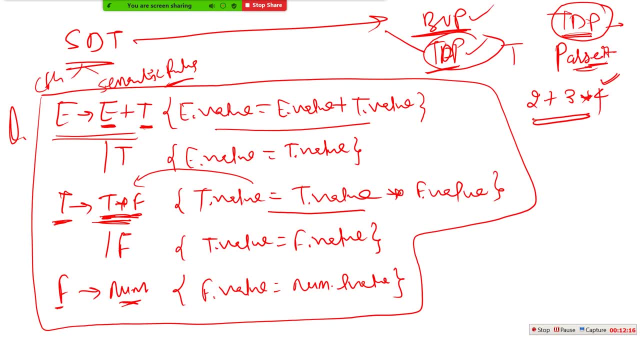 using top down parsing that is from left to right. you know that top down parsing is left to right and bottom parsing is from right to left in reverse manner. it is rightmost to derivation. bottom of parsing is right to rightmost derivation in reverse manner and top down parsing is leftmost derivation. 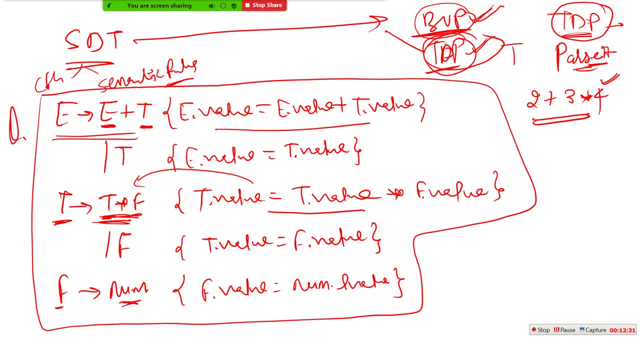 we have already discussed it in our previous sessions. right now, what my target is. my target is to draw some semantic, the syntax and semantic tree for this. so i will follow my target. 2 plus 3 into 4 guys. it is my target. so here i will start my target and i will start my target, so i will start. 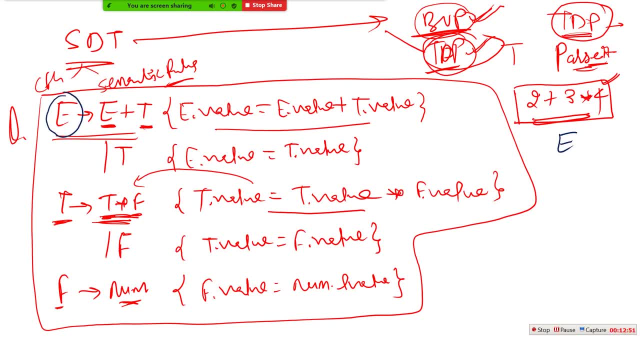 start from E, because E is my starting symbol. I will start it from E, right, what my target is. my target is to follow. this input means my syntax tree, my semantic tree. my semantic tree should generate the value of 2 plus 3 into 4. so, firstly, what do I do? have 2 plus? 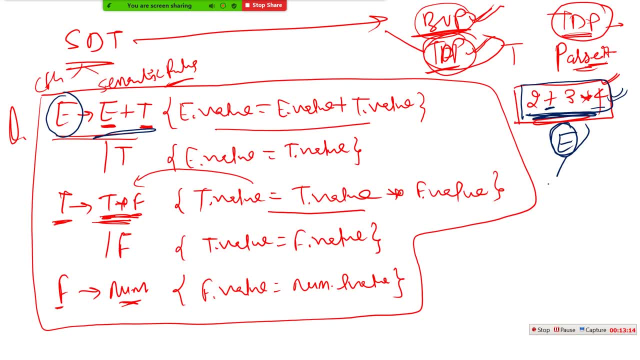 3, so I will. I will generate this transition, that is, e derives e plus t. okay, now, after that, I need to take two value here for e. so what I will do? I will derive this t from this e, so I will write t, and this t will derive f, and from f I will take the value of this. 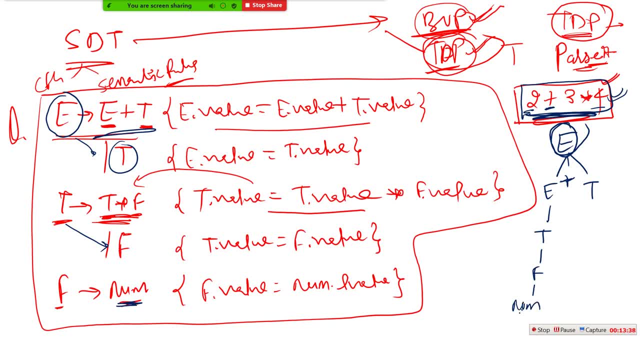 num. so if this f will take num- value of num. and what is my num value exactly? here is 2, the value of my num value is 3, so I will take the value of num, value of num, value of num. my num is 2 here. now I need to add this 2 with 3 into 4. so for this transition, t will 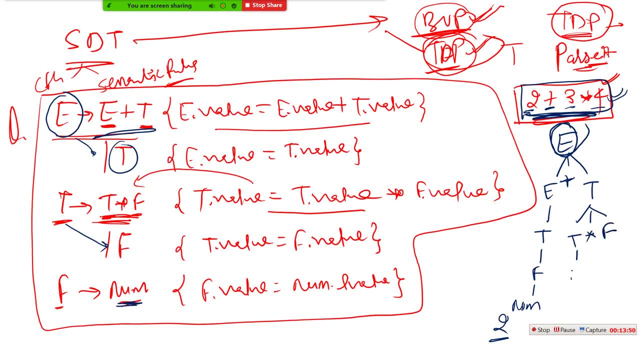 further derive t into f and t will further take value of f and f will generate num value. and this f is will always, always, always generate num value. the num value of this is 3, because I took this 3 here and this is 4, so now my semantic tree is in front of me: 2 plus 3 into 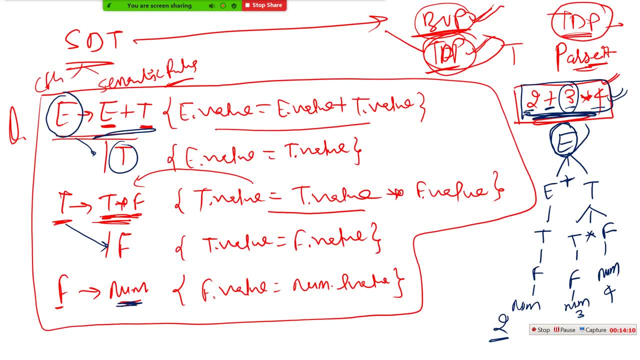 4: right, it is my semantic tree. how I will parse it. focus it now. how I will parse it. how I will gonna parse it now. focus here I am going to parse this tree. so, guys, I will start from the initial symbol e. I will start parsing from initial. 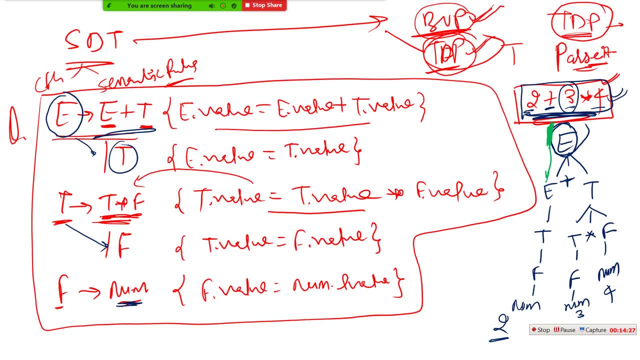 symbol e. I reached at this e, but I didn't get anything here. I didn't get anything here, so I will parse some more bottom level. I don't get anything here. I parse to f and this f has generated value of n, so here here f is replaced with num value of t, so I will parse. 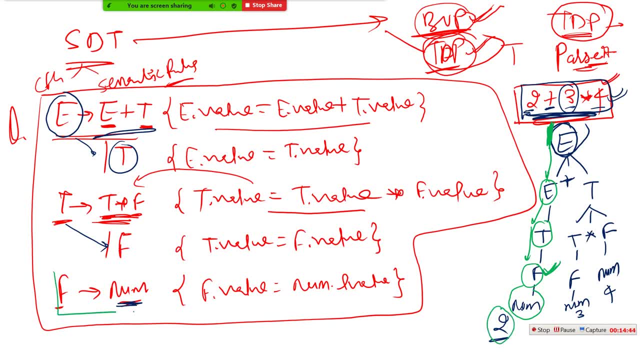 value of 2, because this num consists value of 2. and using third, this transition: using f derives num. using f derives num. I can replace this f with 2. I can replace this f with 2. I can replace this f with 2. now this f dot value will be parsed to t dot value. this f: 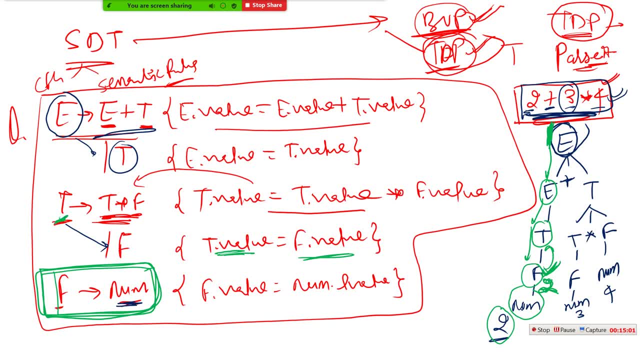 dot value will be parsed to t dot value according to this transition. so this 2 value will be parsed to here. this 2 value will be parsed to here again, if you will see, this t value will be parsed to 2e here. so I am going to parse this. f dot value will be parsed to 2e. 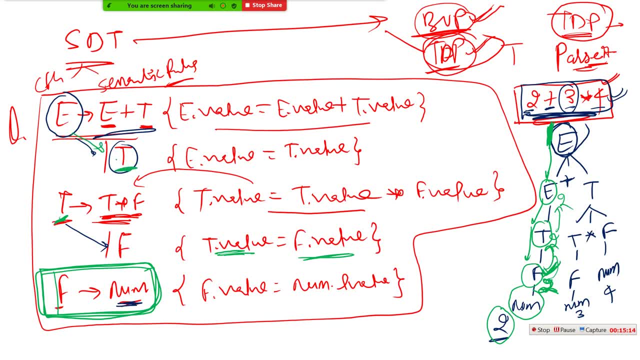 here. using this transition. using this transition, this t value will be parsed. this t value will be parsed to e here now. this e consists to: this e consists to 2. this e consists to 2. now I have addition. I need to add this 2, but to whom I will add it? to whom I will add it? 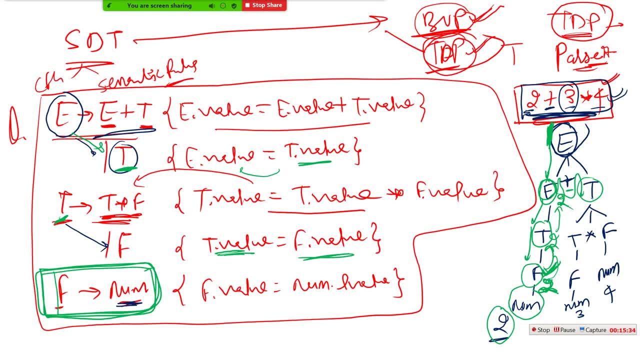 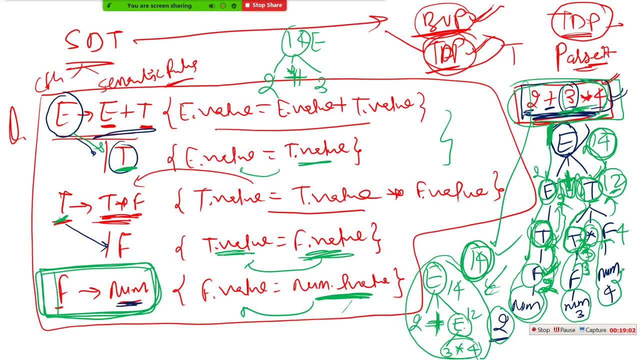 Don't write these non-terminals. Non-terminals are not a part of syntax tree. So on the place of this, it 12 would be there, and on the place of this, it 14 would be. result: Right, guys? 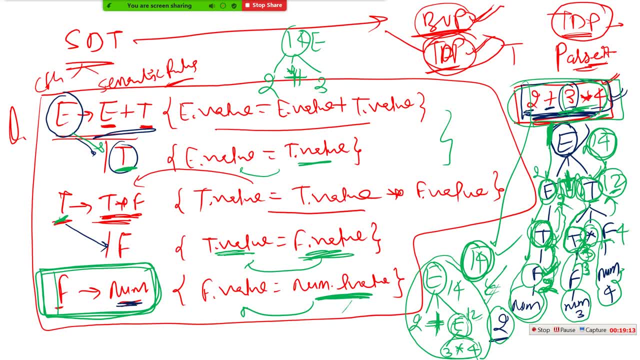 Soumya. sir, I can understand the traversal. You can't understand Soumya. is it clear to you or not? Soumya, is it clear to you or not? Please answer me That how I did this example. 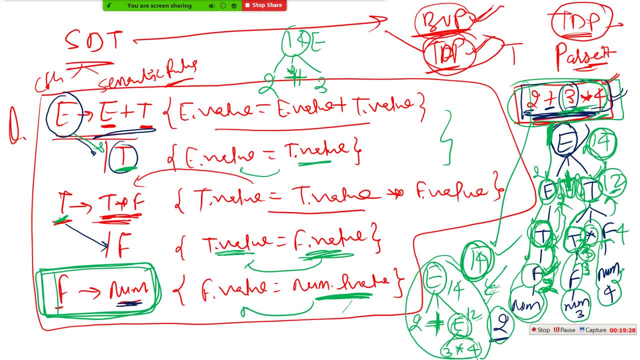 Is it clear to you or not? It is not clear to Soumya. Is it clear to you or not? guys, Please tell me, Because many candidates have answered. it is clear to them. Okay, Soumya, if you don't get this answer. 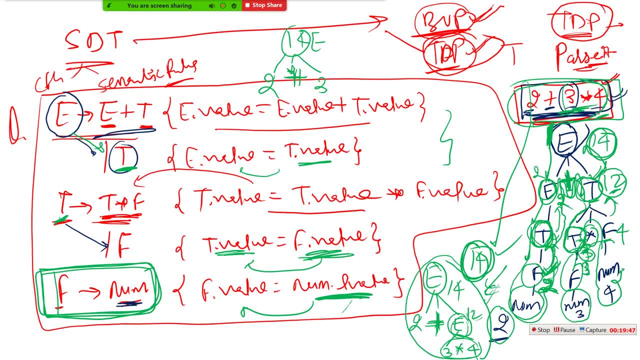 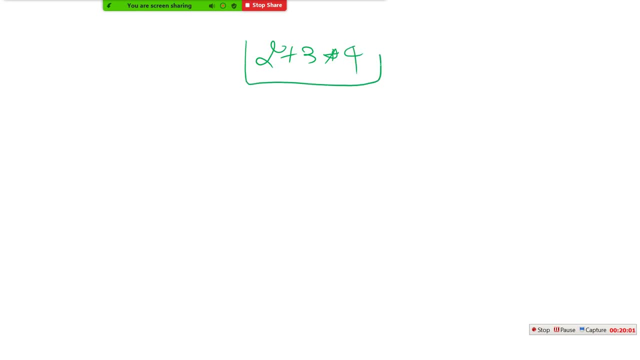 you just focus here once again. Right, sir, the traversal. I can't understand Actually, Soumya, we need to traverse. Actually, my basic target here is, you can focus here- 2 plus 3 into 4.. It was my input string. 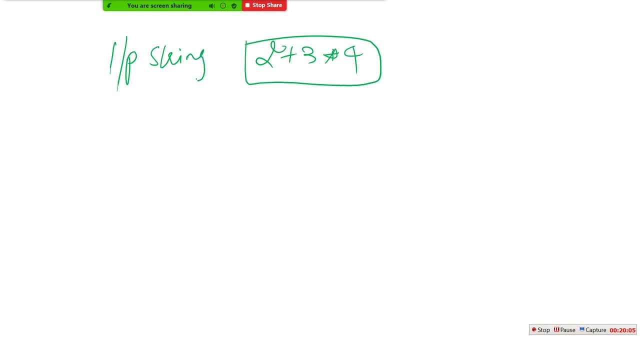 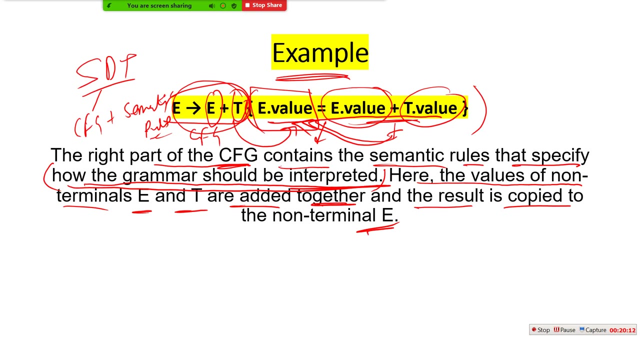 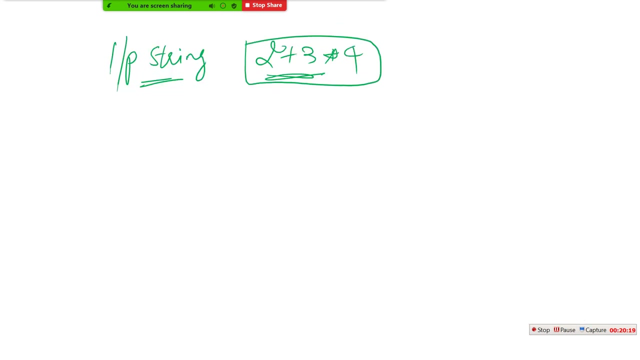 It was my input string. Okay, it was my input string and on the basis of this input string, I need to generate semantic tree. I need to generate semantic tree using this grammar. Now, it is upon us. It is upon us. 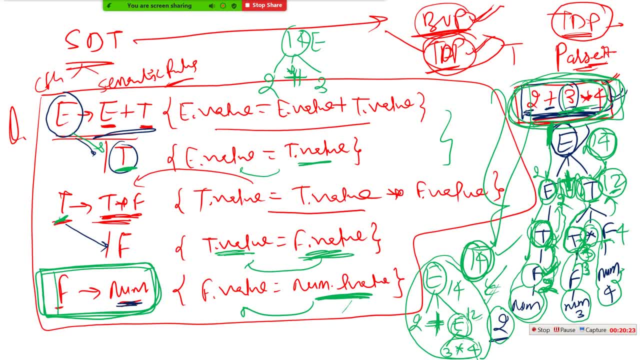 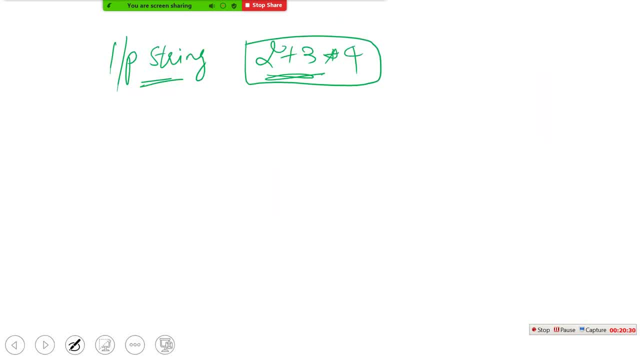 We need to apply our concepts, We need to apply our aptitude In order to create semantic tree so that it can generate a string 2 plus 3 into 4.. So that it can generate a string 2 plus 3 into 4.. 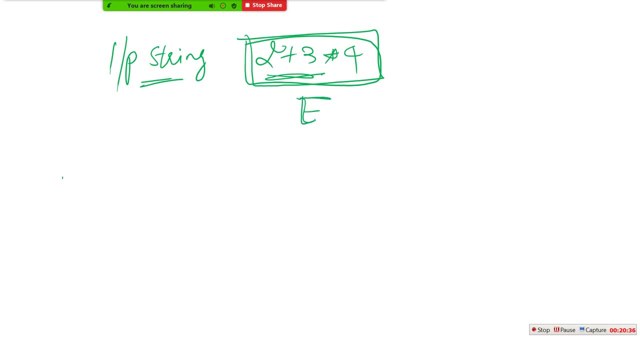 Now we always need to start it from E. We always need to start from the initial symbol. that is the starting symbol. that is E here. Now E will generate. First statement should be E plus T. Why E plus T? Because I am getting addition operator here. 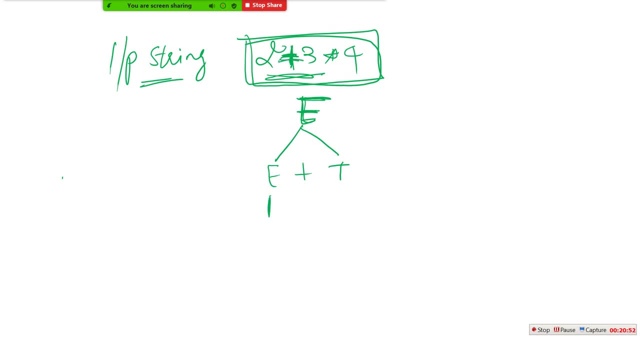 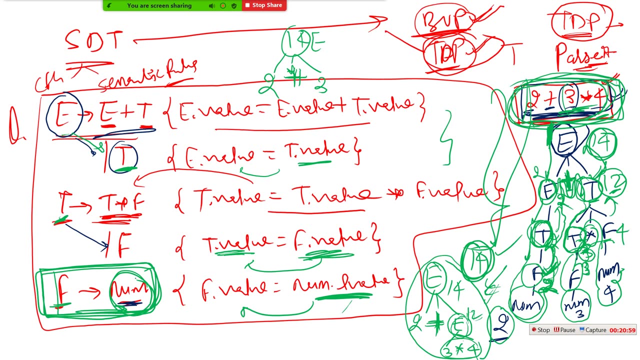 So I initially take the. I should generate E plus T, But E can't generate my num value. E can't generate Only F can generate num value. Only F can generate num value. So in order to get this num value to this E, 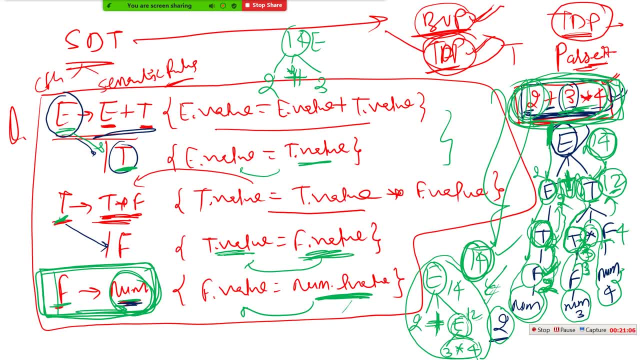 in order to give this 2,. in order to give this 2,, that is, this num value. in order to pass this num value to this E, what I need to do, I need to further make a transition from this E to T. 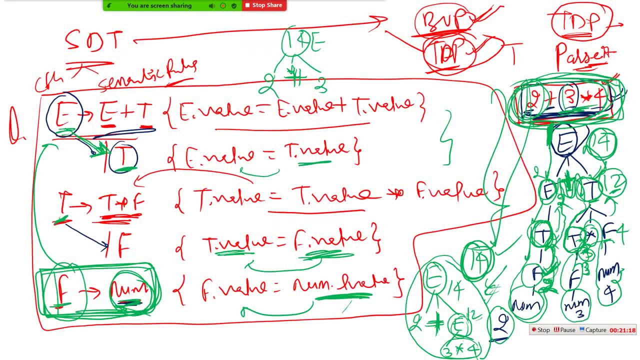 So I will transit E to T. I didn't get num value yet. Why? Because this T don't have any num value. Num value is only here. So this F only consists of num value. So this T will further generate F. 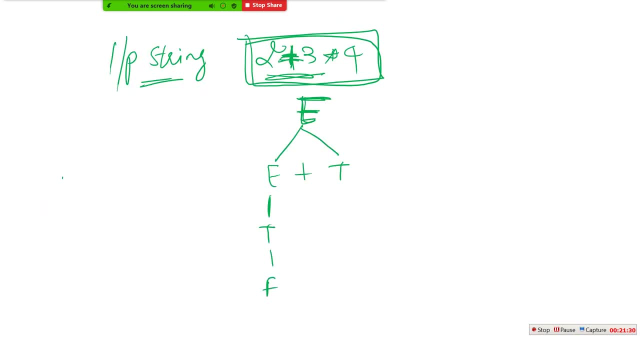 So this T further generates F, This T further generates F. Now this F now have num value. So I traverse here And this num now will give me 2.. Because only this F have num value And I need this 2 value here. 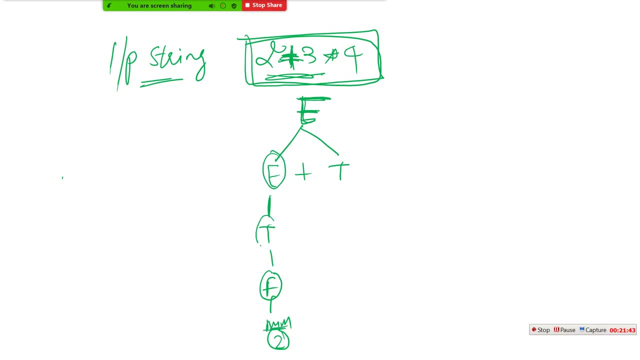 So, in order to get this num value here, I generated T From this transition. From this transition, I have generated T. From this transition, T derives F. I generated this level And from this transition, T derives F And finally I got my num value. 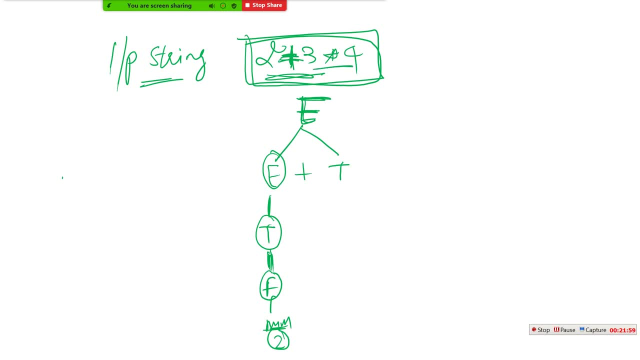 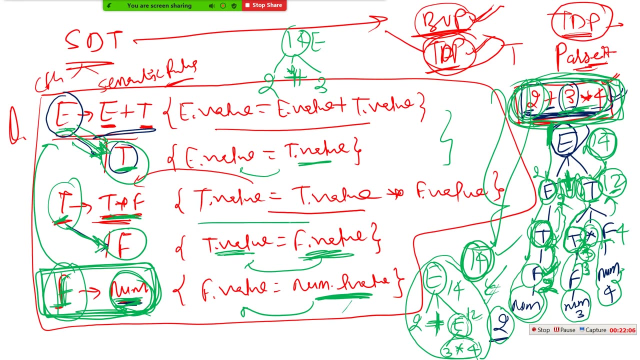 But I only got 2.. Now I need to 3 into 4 as well, But I need to multiply here. So you can simply check here that E dot F, T dot F is here. T value equals to. 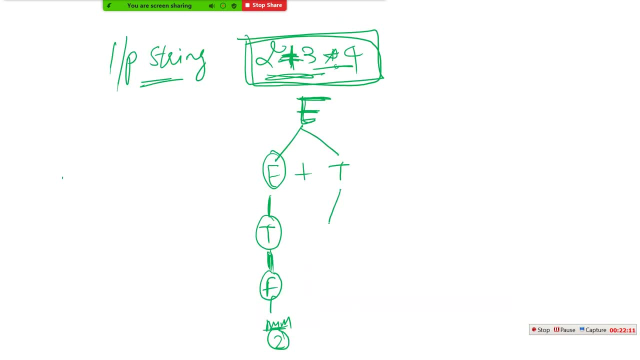 T value dot F value is existed here, So I will just write it here. T multiply with F And I need to pass F value to here. But I don't have any F value, So I will generate F value by deriving F from T. By deriving F. 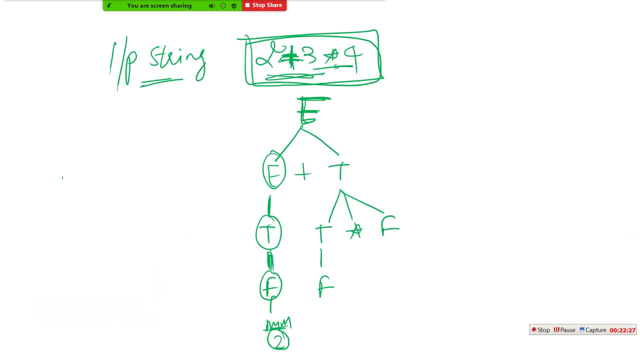 By deriving F from T Using this transition, And I will generate num value. then And now this have 3.. And F will generate num value And this num value now have 4.. Okay, So this is my semantic tree. 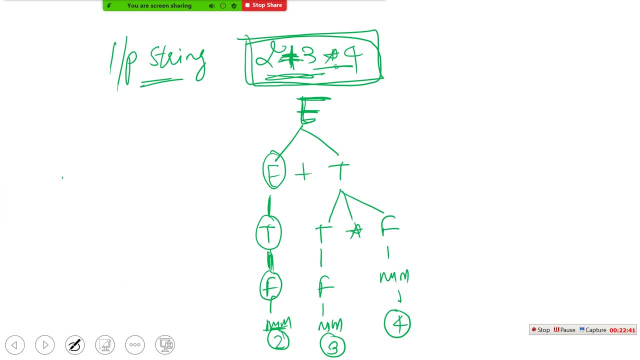 Now you need to understand traversing, So we will start from here. We reach to here, But we don't have any num value to this. E. So we traverse on the bottom most side T. So we traverse on the bottom most side T. 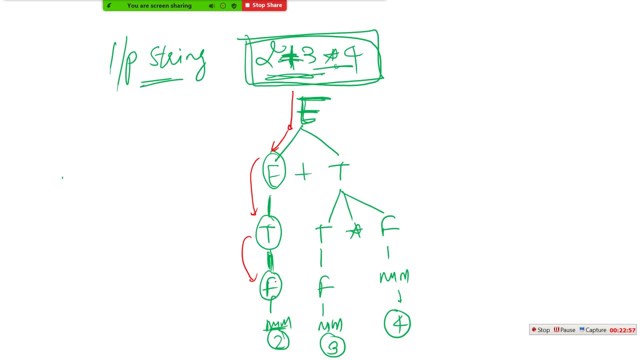 No value to this T, So I again traverse to this F. I don't have any value to this, But this F further have num value, That is, 2.. So this F now consist value 2.. Now this F will pass this value 2. 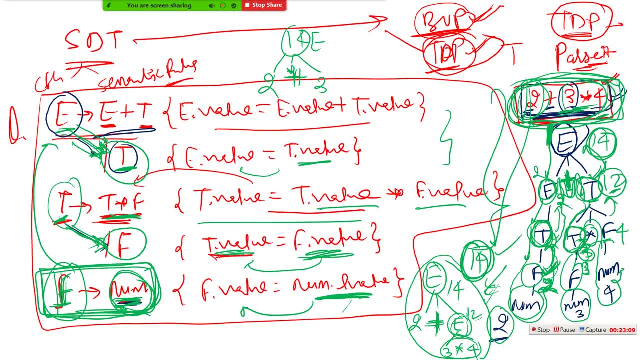 to this T How? Because my semantic rule is saying that T value equals to F value. So whatever value F have, it will pass this value to T value. In transition, T derives F. So in the transition, T derives F. 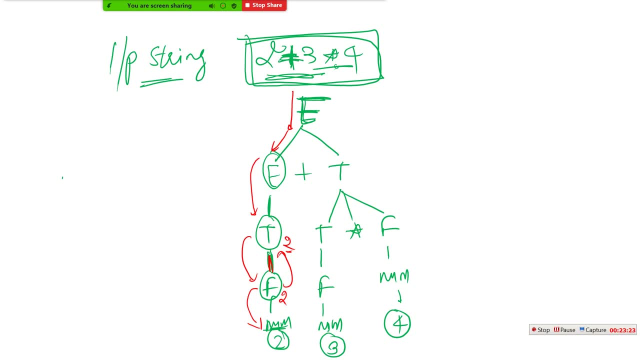 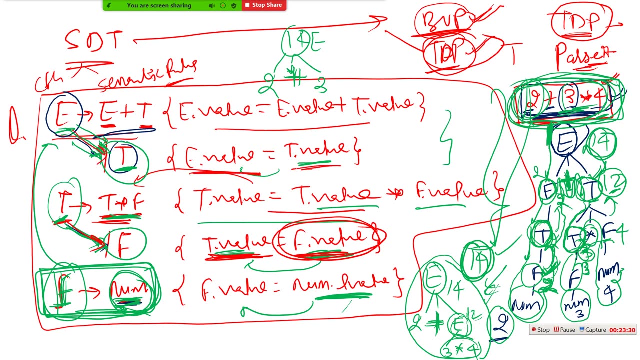 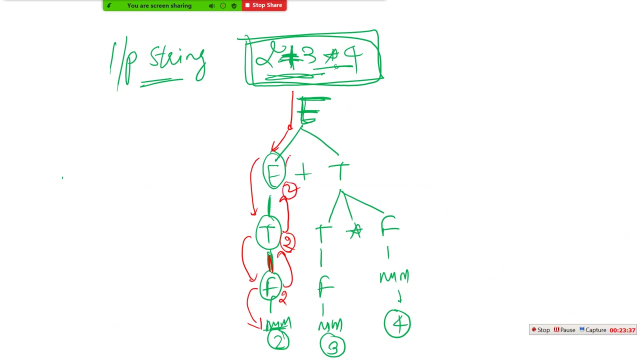 In transition T derives F. This value is passed to here. two value will be passed to here by using: by using transition e derives t. that is, e value equals to t value. this transition has. this transition has passed this value 2 to here. now i need to add 2. i need to add 2 with t, but i don't have any value of t as of now, so i will. 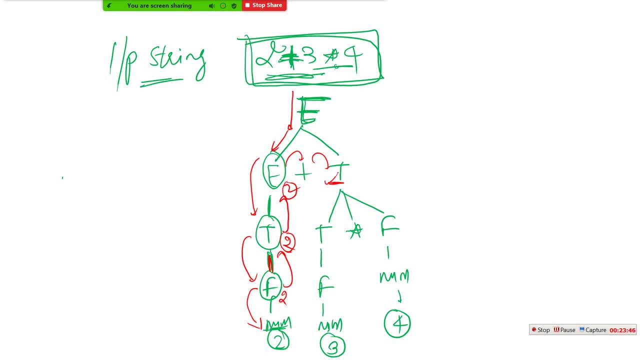 wait. now i will wait and i will generate this, the value of this t. in order to generate value of t, i will further traverse to this t. i don't have any value of t. now i will go to f. i don't have any value. this f have num value 3, so i got f. this 3 is a num value of this t, because this 3 is passed. 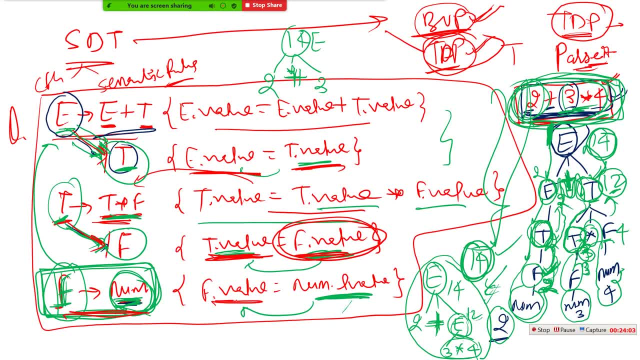 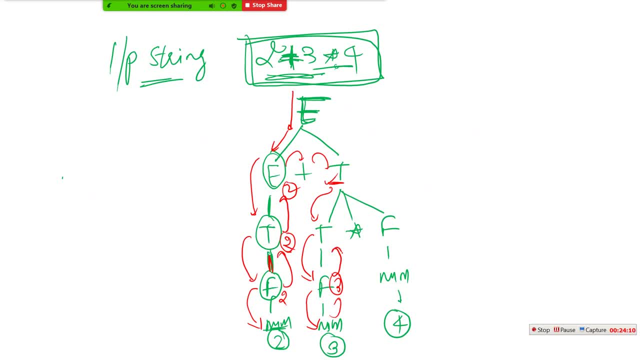 to this f. using f is deriving num, that is, f value is deriving num value, so num value. i will pass this 3 to here now. further, this f value will pass to t, that is, 3 will be passed to here using this value. that is, t value equals to f value. 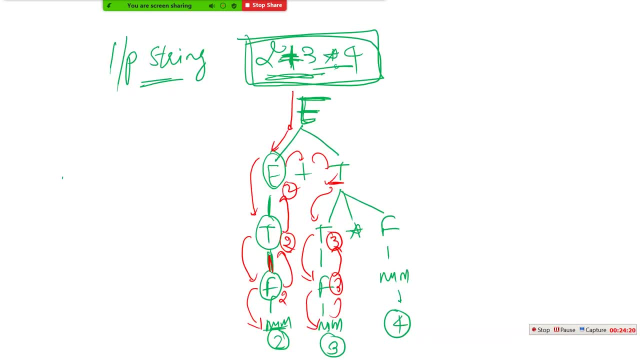 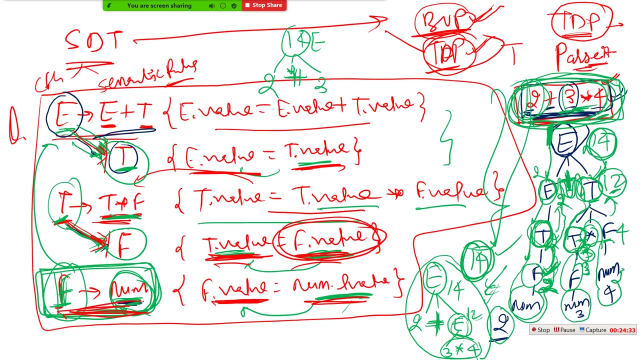 so this t derives f would be passed here, and now i need to multiply this three with this f. but i don't have the f value now, so i will traverse it again back. i will get num value. what is my num value? four. so this num value is passed to this f. that is four. this is my f derived num value. so this transition. 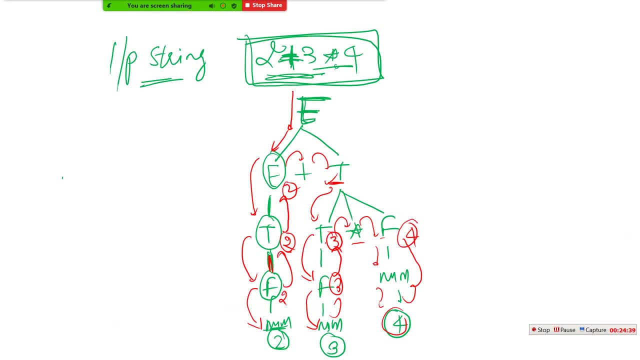 will do this and this four. now i have t. it is waiting as of now. so three into four will be done and result 12 will be passed to this t. using, using, using, using this transition, using this transition, we have done this. so, guys, if you will observe here: first multiplication is first the. 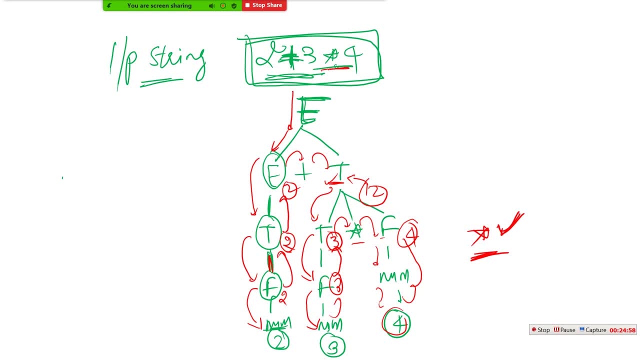 result of multiplication is done because the precedence of this multiplication is higher. after that i got the value two already waited here. now 12 plus 2 will be generated and it will pass the value 14 to this e and this e will generate 14 as answer. so our first multiplication. 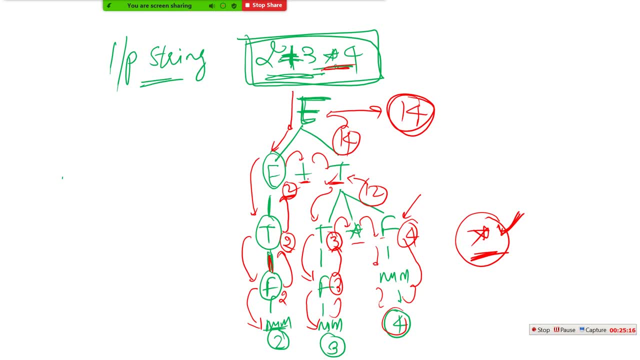 would be done by compiler, by our computer, and then this addition operator will be done by our computer. so, finally, the 14 results will be passed as output for this. so, guys, is it clear now? so may, is it clear to you now? very good, is it clear now. so semantic tree is generated. generate meaningful 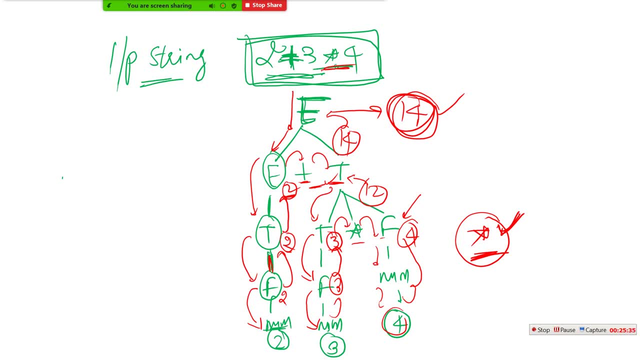 pass tree right. then how can say passed is meaningful or not, how we can say pass trees meaningful or not? semantic tree is generating meaningful pass tree, right? yes, so guys, here we are doing it. arun kumar, here we have generated this semantic tree manually, but compiler- only compiler- by default- have such programs so that 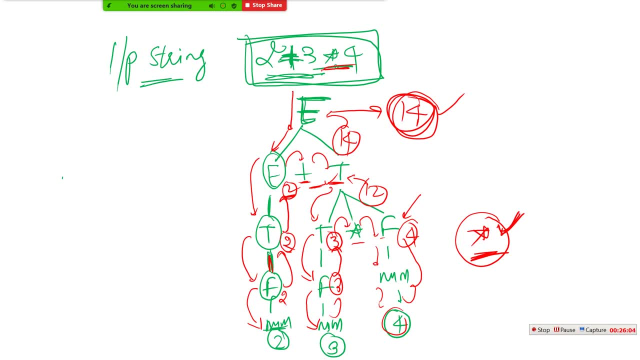 it will check whether our constructors are valid or not, whether our syntax are click syntax are valid or not, whether our identifiers are valid or not. so it is a part of compiler. compiler or by default will have such program by which it will, it will itself itself it. 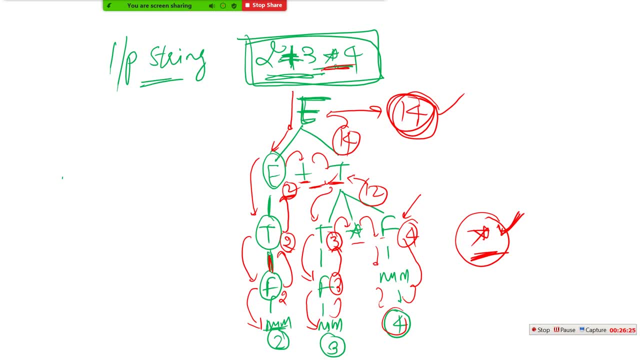 will clarify that, whether the token which is passed from upper pages present in our library files or not, suppose we have passed only printf on the place of printf. we only only have printf. we don't include any here. so this, this keyword doesn't existed in the library files of compiler, so 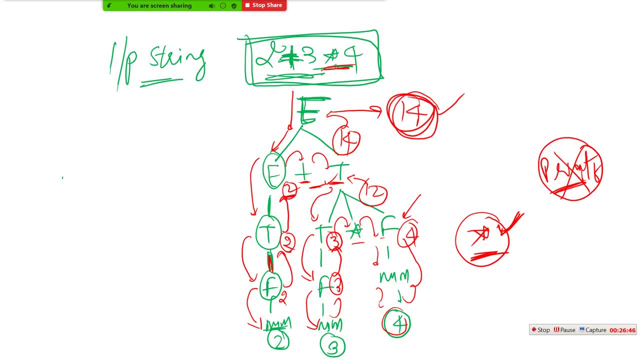 compiler itself treat this as a non-valid talking and it will not be putted in our syntax tree, in our semantic tree, so semantic error may be generated at that time. so we need to correct this semantic error while writing the program. is it clear, arun? is it clear, please? answer is: 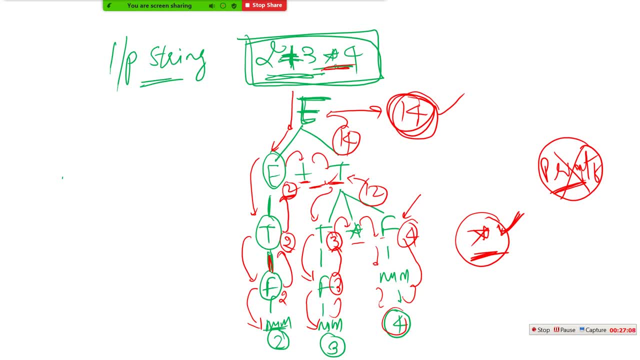 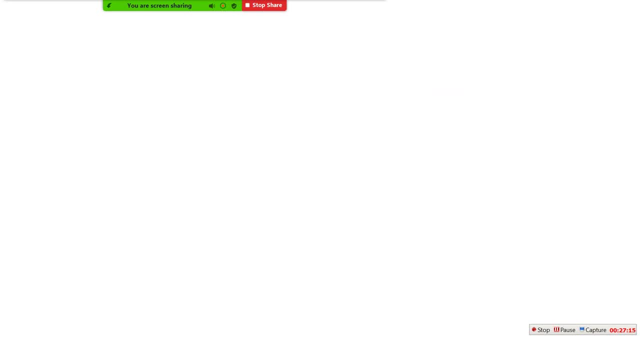 it clear, arun, please answer me. okay, guys, am giving next question to you. now i am giving next question to you. it is very, very important question. it is a gate question, guys, it is a gate question on semantic tree. it is a gate question. we all need to answer this question. so i am writing my sdt in front of you. e derives. 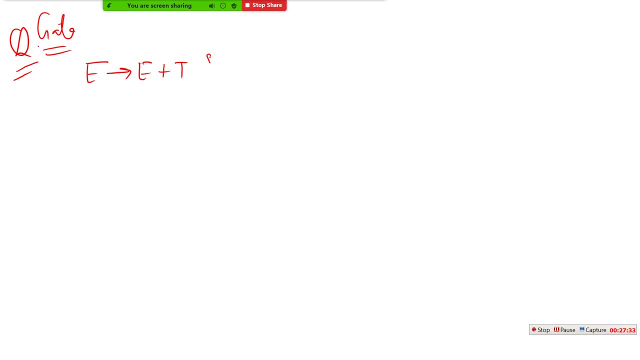 e plus t and semantic rules for that. this is print f, print f plus, so it will print f. the first, first, first transition will generate print f, and next transition is t, so it will print two. it will print two. it will print two. okay, it will print two, and next transition is t. the transition is t. 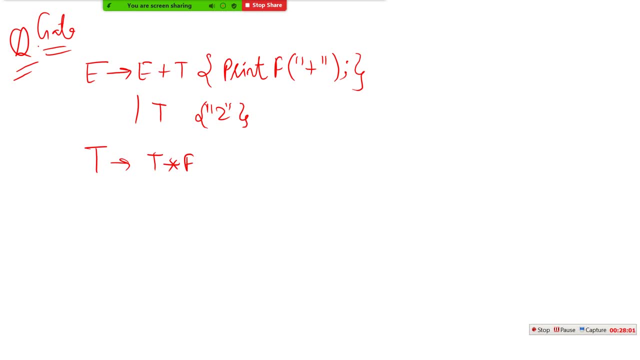 into f, okay, t into f. and semantic rule is: it will print. it will print multiplication symbol here. it will print multiplication symbol here and t also derives f, and it will print. it will print four, suppose it. it will print four. okay, it will print four. and next i have f derives num. 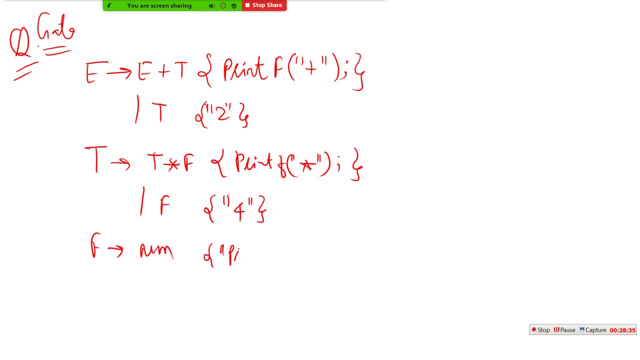 and semantic rule of this num is: it will print, it will print. suppose print f is given to us, then it will print num value. whatever num value we will have, we we have- it will be printed with this statement. right, it will be printed with this statement, so you can assume it like it is a first statement. 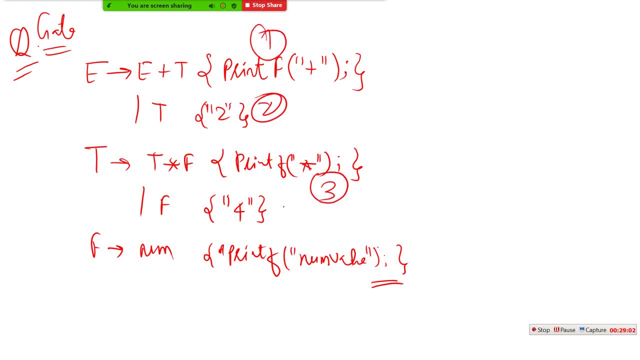 it is a second statement, it is third statement, it is fourth statement and it is five statements. these are the five statements. okay, how many statements? we have five statements. we have three things to write down. these three things must be represented by th. still right string apple. no change thisignon. 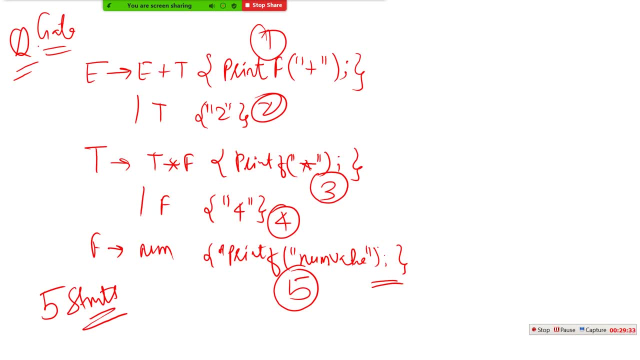 regular trajectory: three four, three, three four. 36, 13, 17, 28, 30, 21. after this problem is okay, after this problem, we will take break, okay. so, guys, we have five statements in that and my question in front of you that: what is the execution order of? what is the execution order of? what is the? 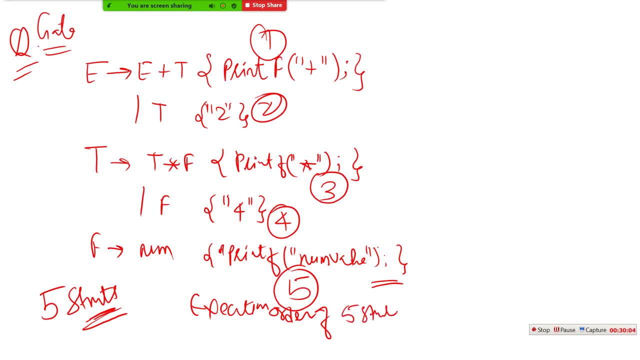 execution order of this is five statements. what is the execution order of this? five statements according to semantic tree. according to semantic tree, what is the execution order of this statement? please answer me. what is the execution order of these statements, these statements? what is the execution order of these statements? means you just need to draw semantic tree. i am also. 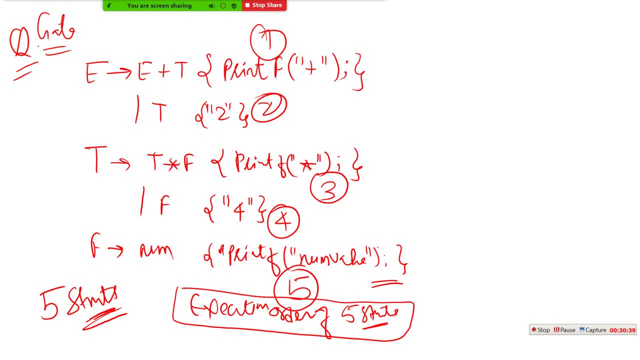 giving you a hint: execution order simply means that, or a Execution order simply means that, what, what statements are executing at the place? You just need to answer. that means which statement is executing, and after that, which statement is executing. You just need to answer the destasy. She will execute first, after that. 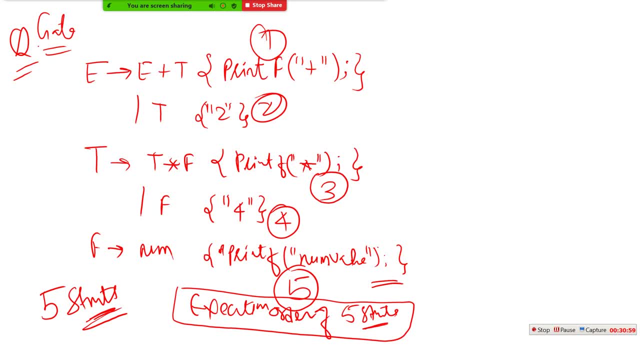 This transition will execute and after that, this transition will execute. So simplest question is that: what is the execution order of this statements? You can answer me using semantic tree. you can answer me using semantic tree. so, guys, I am giving you three minutes. I am giving you three minutes to solve this problem. you will 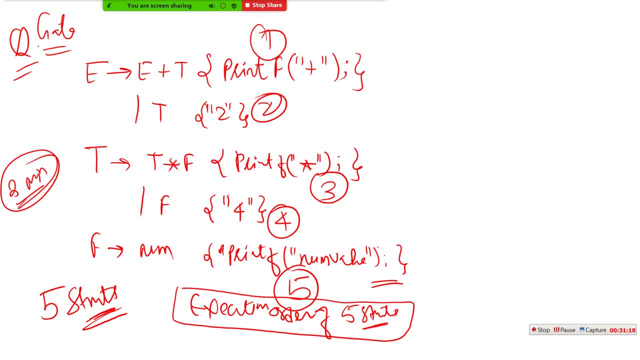 need to. you will need to draw a, okay. so, okay, guys, just focus here, focus here. after this we will take a question. okay, focus here now. focus here. let me tell you something more about it. let me tell you something more about this semantic tree, and after that we will take a problem and after that we will. 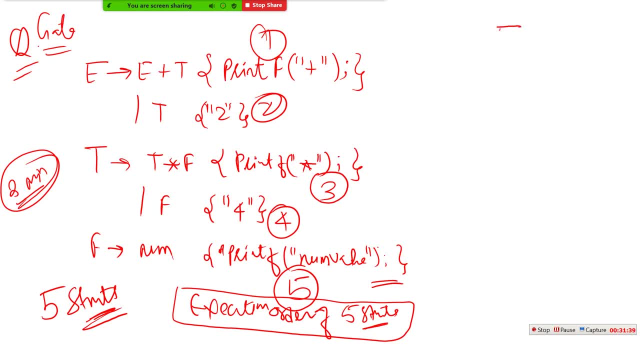 take a problem. so let me start it from here. suppose I am starting here. I am starting it from here. suppose my input string is again the same. suppose my input string is again the same, that is, 2 plus 3 into 4. again my input string is there: 2 plus 3 into 4. so what I will do? what? 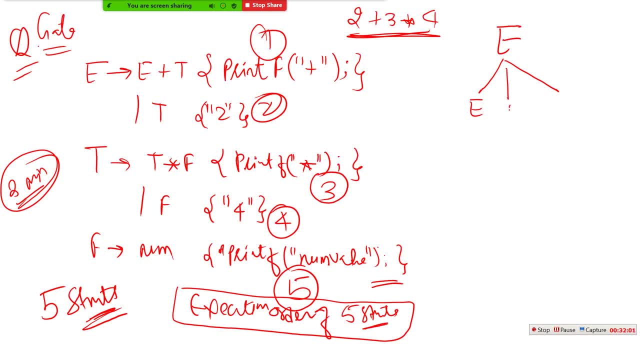 I will do. I will just generate it like that: e plus P and this is my. you can simply say that this is my first statement execution. if I will execute the value of this T, I will say that it is my first statement execute right, and this e will further generate T. 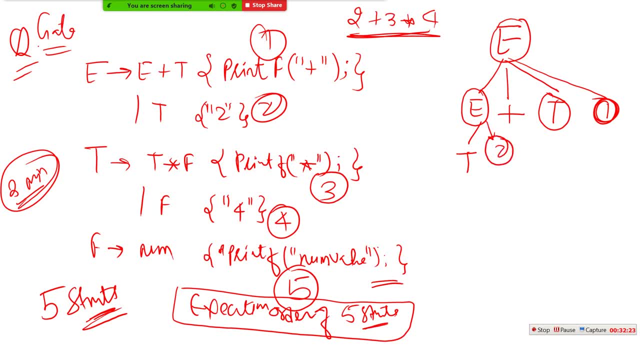 so if I will execute this, I will say: it is my second statement execution and this T will generate. this T will generate P into F. so if I will generate, I will execute that. I will say that my- Let me say that my- third statement is executed. this T will further generate F and. 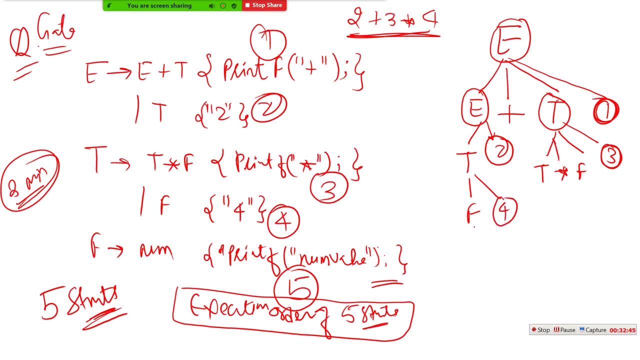 if I will execute that, I will say that my fourth statement is executed and after F, I will generate numValue. if my numValue will be generated, I will say fifth statement is executed. similarly, here, F would be here. if I will get value of this T, I will say my fourth statement. 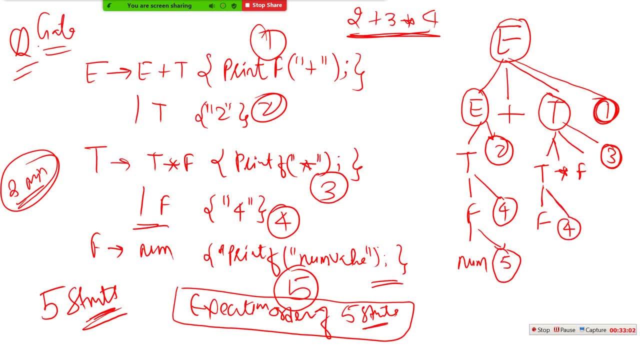 is executed because T generates F is a fourth statement, you can see. and if this F will generate further num, so Почему nENg도了? i will generate the f value. i will say: fifth statement is executed similarly here. if i will generate the f value, that is num. so i will simply say that my fifth statement executed because f. 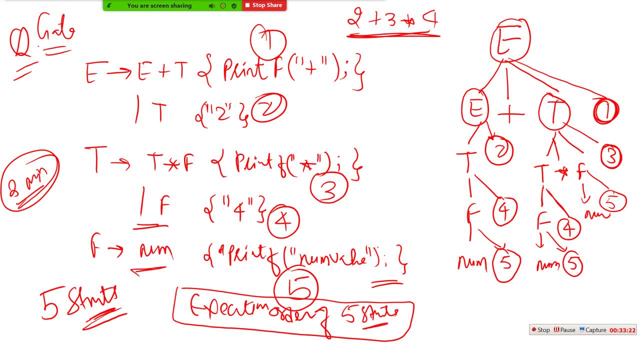 derives. num is the fifth statement, right? so it is my syntax, it is my semantic tree. so, guys, let me traverse it now. you already know- because we have already solved it, but still i am solving it- that we will start from e we. we go here e, but we don't have e value of e as of now. as of now, we don't have. 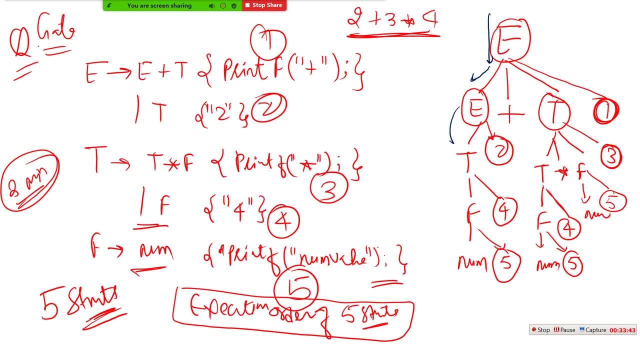 any value of e. so what we will do, we will further traverse from this e to t and this t will get value of this f. now this f is still don't have value, but this f will get value directly from num. so this f is generated first. so execution order would be like this: transition is generated first. 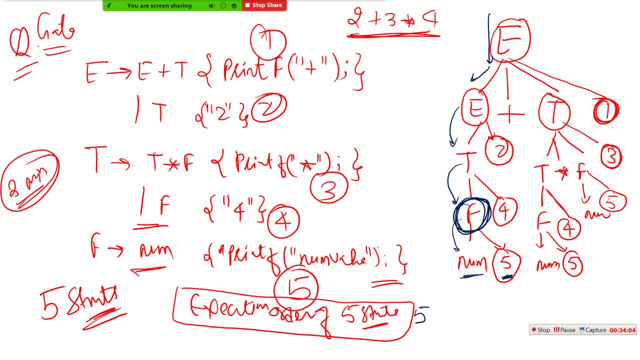 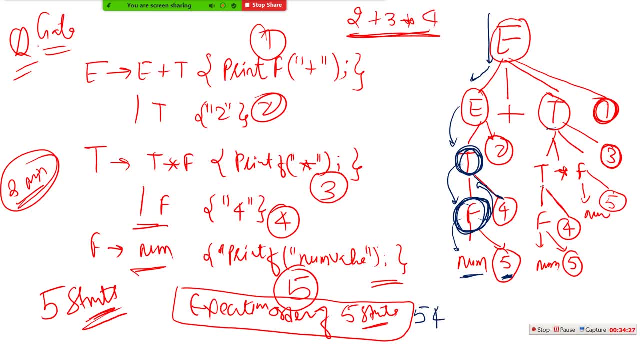 fourth statement is now executed, and after that the value that is passed here, that is the two. two is passed here. two is passed here. this two is passed to here. this two is passed to here now. so now statement two is executed because e derives t. e derives t is a statement two. two is generated here now. this two is holding here. 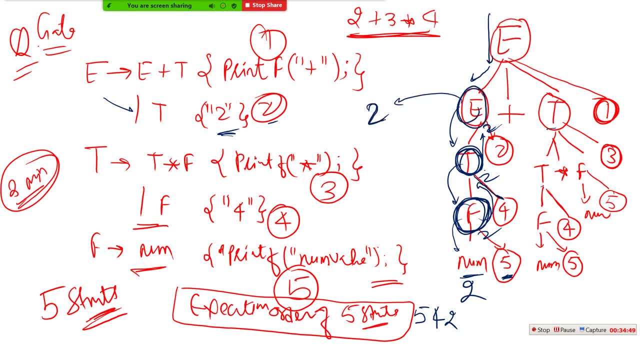 two is passed to e. this e here two, so two. this two is waiting. this two is now waiting. waiting for whom? this two is waiting for value of t, so that it can add the value of t in it right now. after this, if you will see, i need to. 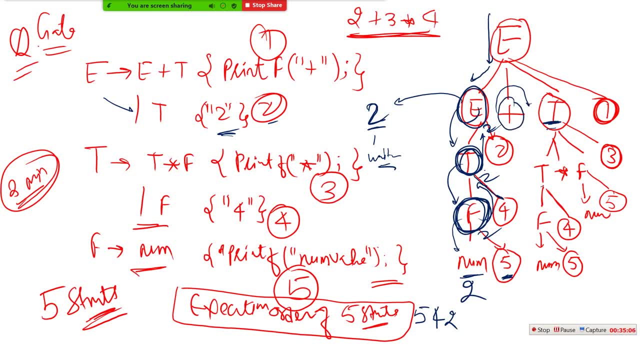 execute this plus. but. but i don't have any value plus as of now. so what i will do, what i will do, i will go to this t. i don't have any of this t. i will go to here if i don't have value of this f. 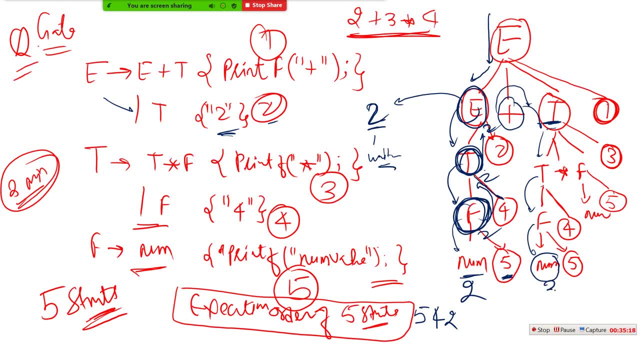 now this f will generate value of num. what is value of norm here? 3. so now statement 5 is again generated, this statement five is again generated and value three is passed to this f. now, now this value of 3 will be passed to this t. 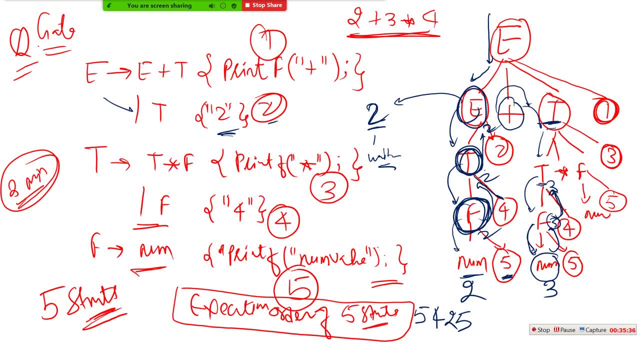 will execute in order to pass this t to this, this 3 to this t. statement 4 will execute in order to pass the value this t 3 to this t now further. this t will hold here now this 3 is holding here. why it is holding here? because it is waiting for multiplication item and after that we will pass. 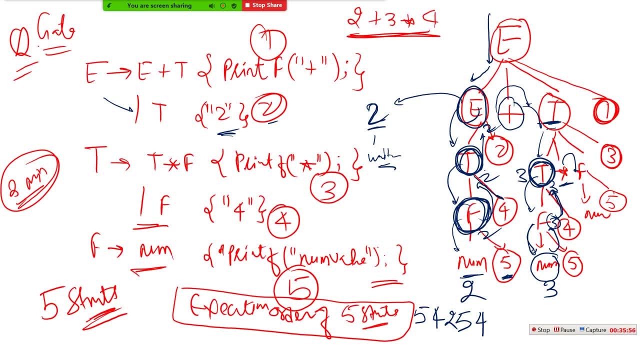 to f and after that we we only got this statement 4 until now, and after that we will pass to this f. this f will generate the value of num, that is, 4, and now this 4 will be passed to this f using fifth transition. so again, fifth transition will be: would be executed and after execution, this: 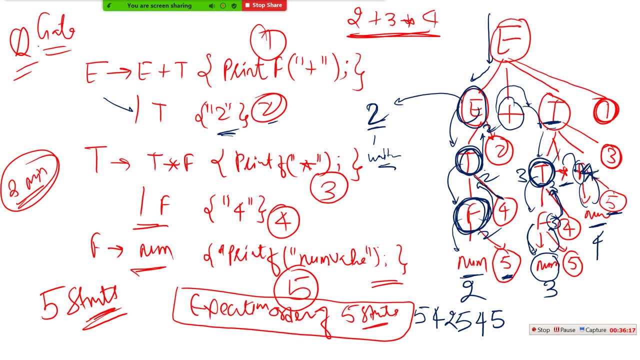 fifth statement. what it? what value it do have now? it have 4. so now 3 into 4 will be multiplied and 12 will be passed to this t. the multiplication of 3 and 4 will be passed to 12. using third statement. using this third statement. using this third statement. 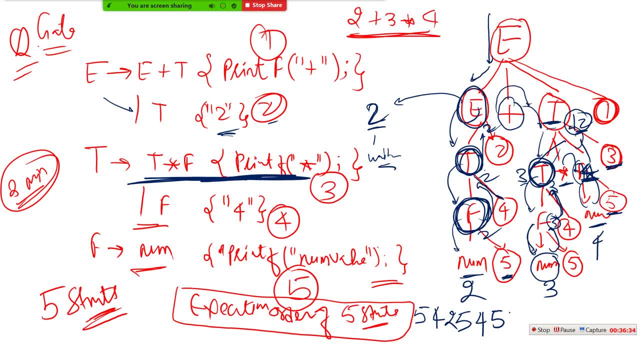 this 12 will be passed to this t. so now we have performed third statement. after this third statement, this 2 is already waiting. this 2 is already waiting. so this 2 and 12 will be added as a 14 using statement 1. using statement 1. using statement 1, we will add the value. 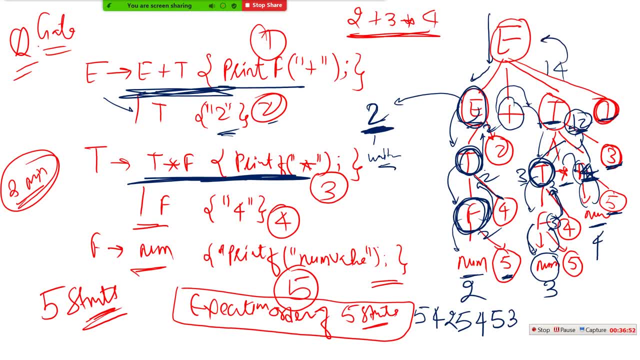 of this 2, with this 12 and this 14 will be passed, and now statement 1 is executed. now, statement 1 is executed. so, after execution of such statement, i am getting my final value as a 14. i am getting my final value as a 14. so how many executions are there? 1, 2, 3, 4, 5. 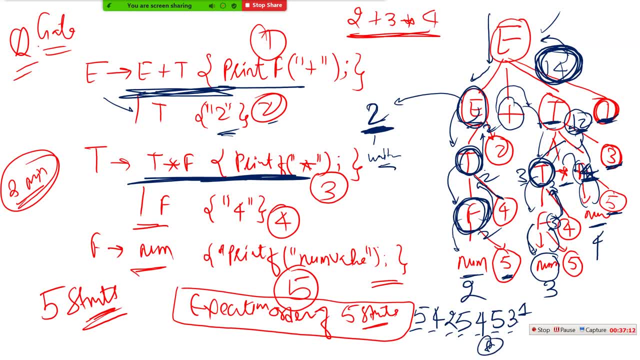 6, 7, 8, 8. executions are there means whatever value we are getting, whatever value we are getting, whatever value we are getting, we are saying that it is the execution. so the execution order of the statement is 5, 4, 2, 5, 4, 5, 3, 1. it is the execution order of the statement. 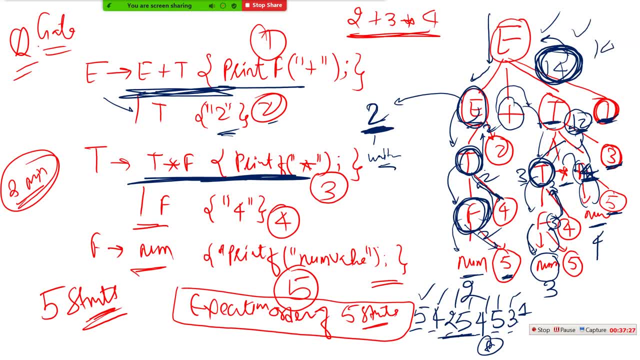 and the value of this is 14. so, guys, is it clear to you or not? now, yes, yes, yes, it is executing just like recursion tree. it is executing just like recursion tree, is it clear to you or not, guys? because it is cfg and cfg uses stake as a data structure. so, until basically, 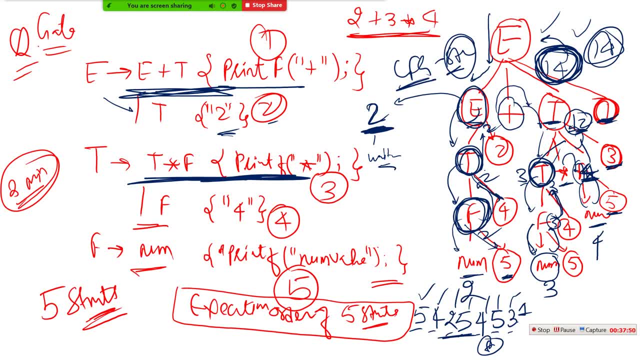 all the concepts are same. is it clear to every candidate, or not, that? what are the execution statements of the execution order of the statement? and the value of this is 14. so, guys, this grammar is it clear? guys, is it clear? please respond me. the execution order of. 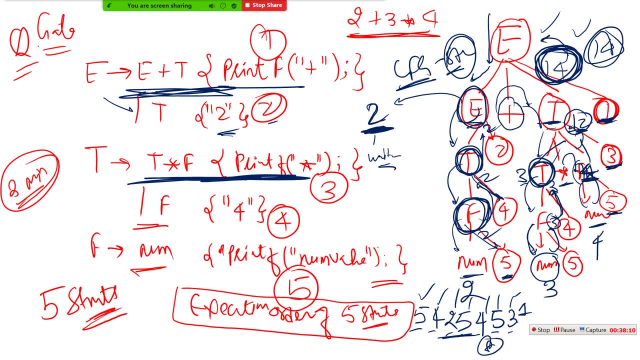 statements are clear to every candidate or not? if it is clear, please tell me in the chat box. okay, it is clear, it is clear, okay, guys. so before discussing the real problem of get, before discussing the real problem of get, are you guys read this grammar? is it clear? 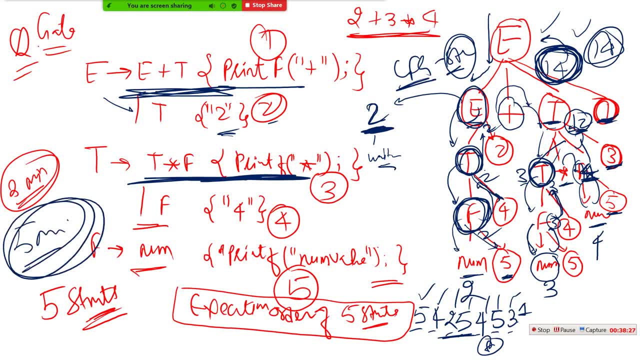 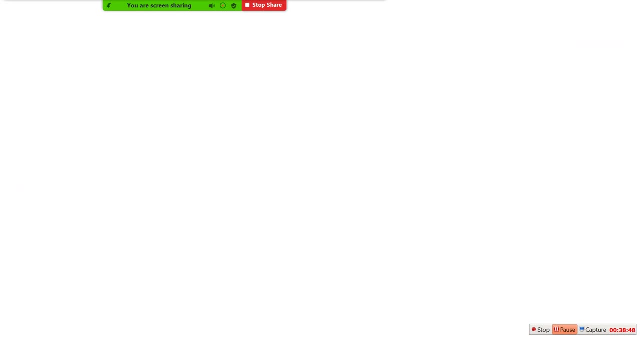 are you guys read this grammar? is it clear? okay, guys, are you ready to take five minute break? after five minutes, we will resume our session. okay guys, after five minute break. after five minute break, we will resume our session. okay guys, is it okay? okay sir, okay sir. hello students. are you ready for the next problem? please comment. 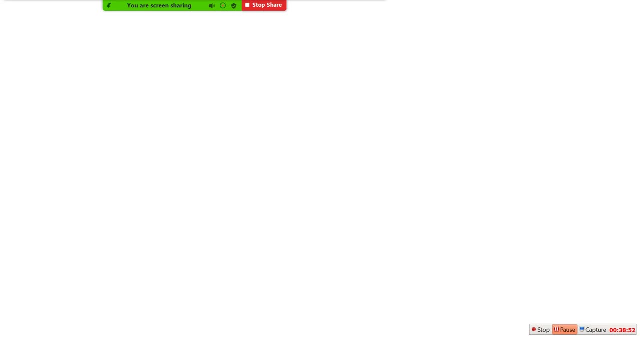 me in the chat box. are you ready, guys, do comment. are you ready? should i discuss next problem with you? okay, so, guys. next question is: it is a gate question. gate question for two marks. guys from sdt. question is: grammar is given to you like s derives double x and w. w is a non-terminal here and semantic rule in front of. 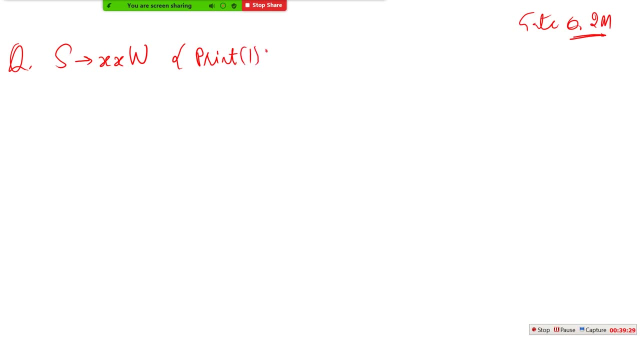 it. front of it is a print one. it is a semantic rule which is given in front of it. and one more transition we have from s, that is, s derives y, and semantic rule is print print two. it is a semantic rule for this. and one more transition we have from: 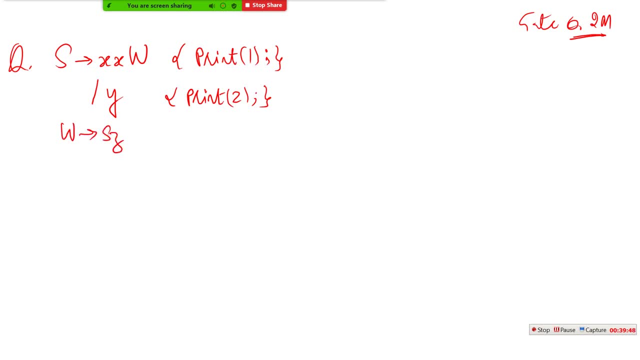 not non-terminal w. that is s z. okay and uh. semantic rule of this is print three. is print three. now the question which was asked in the gate. the question which was asked in the gate is that the following string is passed as a input, the following string: that is double x, double x. 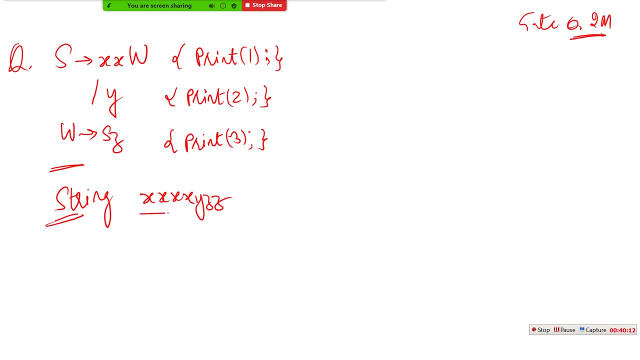 y and double z. this string is passed as a input. this is a input string. it is a input string. it is passed as a input. it is passed as an input. you need to answer me: what is the output? what is the output semantic tree will generate? what is the output? this semantic? 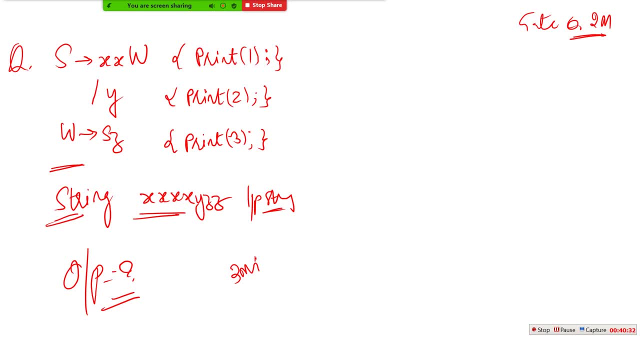 tree will generate. guys, i am giving you three minutes to answer this question because it is very, very important. gate two marks question. if you are able to solve this question as of now, you can sure that you are getting the complete concept of sdt and we can move forward for the. 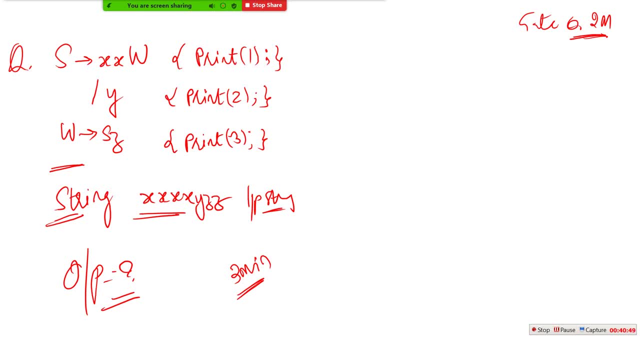 next gate and isro and bark problems, right? so guys do answer me. i am giving you three minute and requesting every candidate to answer this question. it is very, very interesting question and you need to answer me that: what is the output? what is the output this semantic tree will generate while? 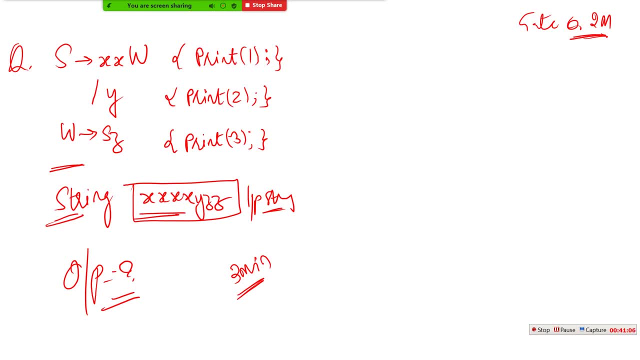 traversing this string as a input string: double x, double x, y and double z. so, guys, i am giving you three minute. i am expecting every candidate to answer. after that i will discuss the solution. input string is in front of you, sdt is in front of you. you just need to apply the concept of 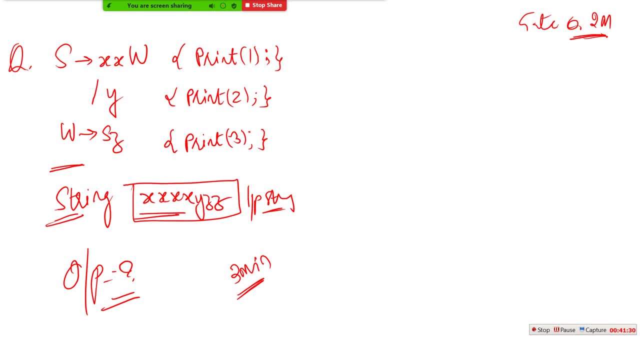 semantic tree after applying concept of semantic tree. answer me. if you are facing any problem while solving the question, don't worry. while i will discuss the solution of this problem, you can focus at that time as well, but before that, please apply the approach which i have discussed with you. apply the approach. 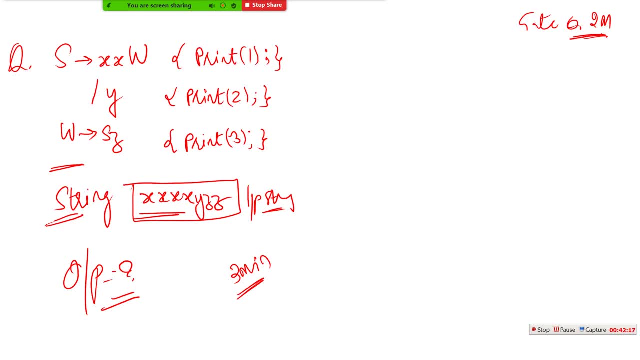 which i have discussed with you apply the approach which i have discussed with you. yes, sir, is the one problem. sir, is there any other browser to access this session other than puffin? please ask this problem from admin. i don't know about it. please ask this problem from admin. sign. 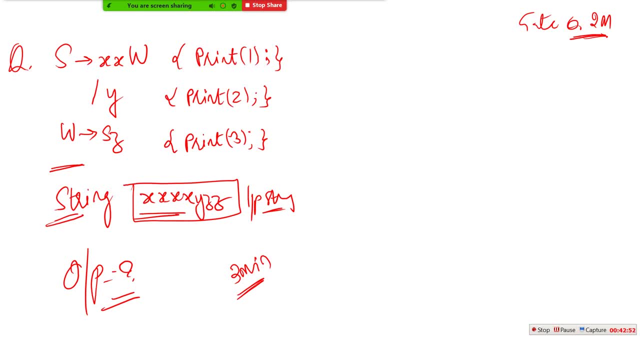 that what you can do it for that. please ask this question from admin. i don't know anything about it, right? please ask from admin. so, guys, are you trying this problem? are you trying this problem? is anybody got the answer? what is the output of this program? what is the output of this sdt while traversing this string? 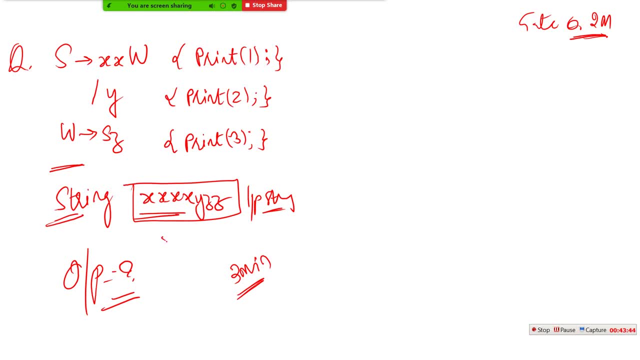 you can apply top down parsing, guys. you can apply top down parsing, no problem. you can apply top down parsing, no problem. so maya is saying: sir double z is not generating, so it will generate. so, maya, please try the semantic tree. we need to make semantic tree manually in order that it will generate all. 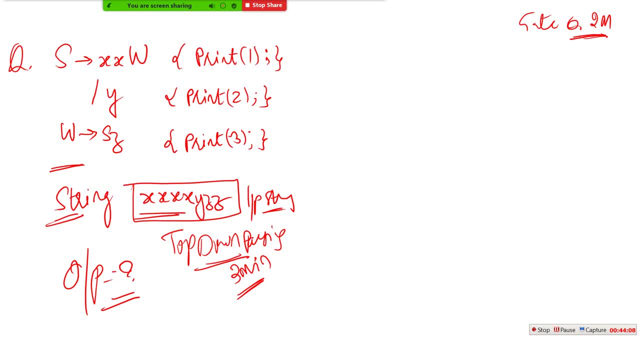 our input string and this input string is a part of this grammar. so don't worry, there is a need. there is a need to make semantic tree such like that. this string will be generated right, so try it on once more by your own. after that i will discuss the solution, because it is very important problem and you need to solve this. 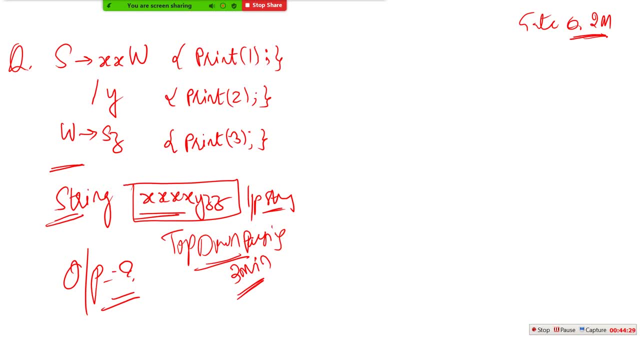 right, because we need to do manually in order to make this string as a part of this grammar and this string is 100 part of this grammar. we have already discussed this grammar while discussing lexical analysis, a lexical analysis. in lexical analysis, we have applied uh in a syntax. 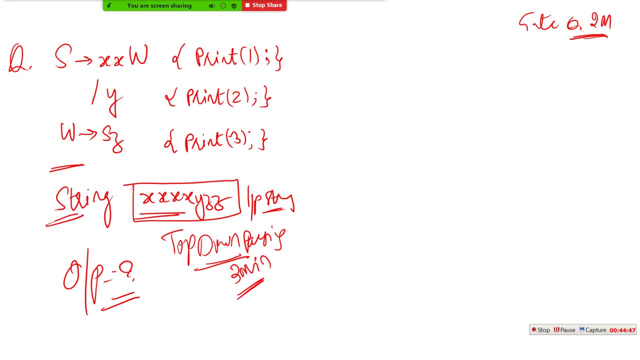 analyzer we have. we have applied a shift and reduce parser in it and in sr parsing this string has get accepted without any conflicts, right in the basics of shift reduce parsing. we have discussed this grammar, so again i am discussing this as a part of get cs question for two marks. 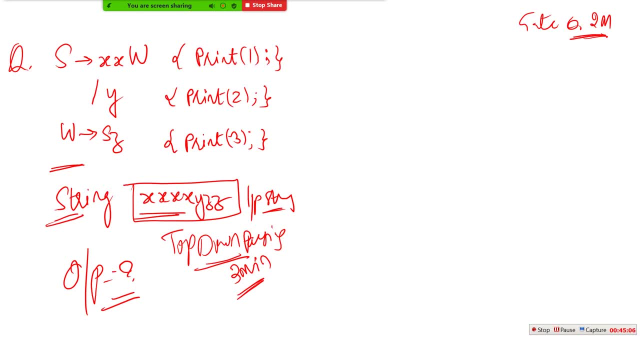 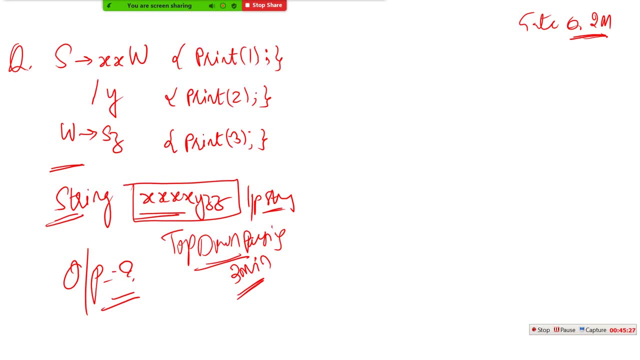 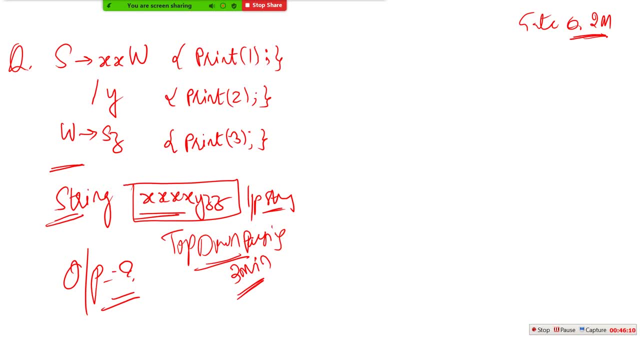 trying this problem. okay, so now I am solving this problem, guys. focus on the screen now. focus on the screen now, guys. we need to generate our string. we need to generate what string I need to generate double X, double X, Y, double Z. so I will start from the initial symbol, that is, s, and I will generate double X. 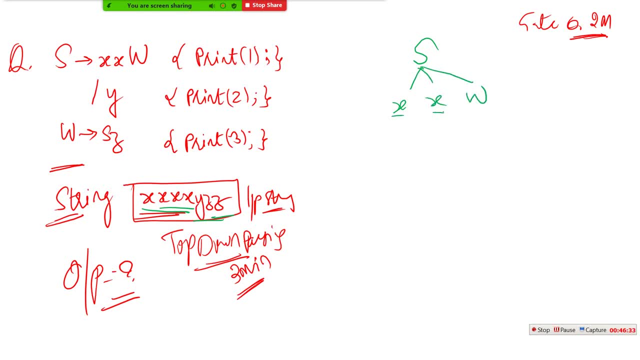 W. now I have two X, but I again need two more X. but from W I can generate s and j and this s can give me two more X and one more W. so I use 4x now and this W will further generate s and jet for me and this s will end with Y. right this? so if you 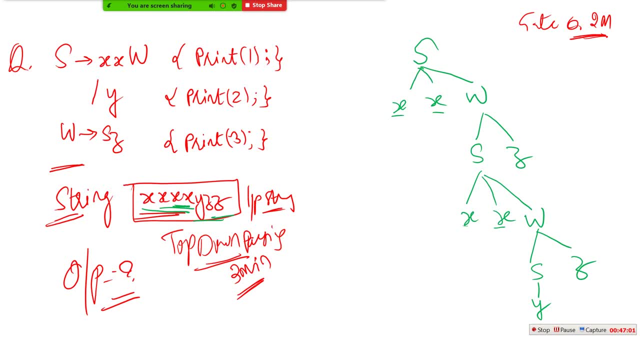 will. if you will do this is derives why this is my second transition. a double x W is the first transition and is read as my third translation is the second and since I am from means 167, I will " transition. so it is a semantic tree structure and while, while traversing this tree, while traversing 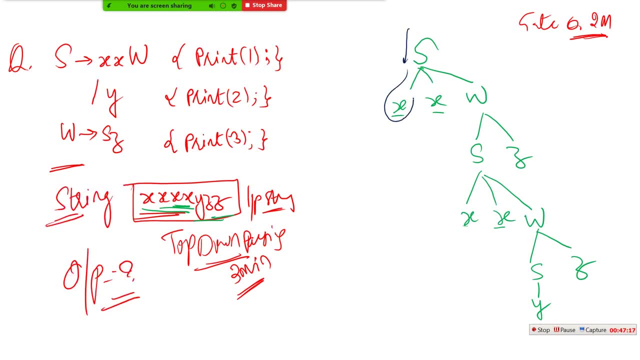 this tree. you can start s from here. you will take y, x, but we don't take x as of now x. we need to traverse it in this manner. in this manner, we will again traverse nx, but double x is not a part of anything, right? double x is not a part of anything and this w is a non-terminal. this is is generating. 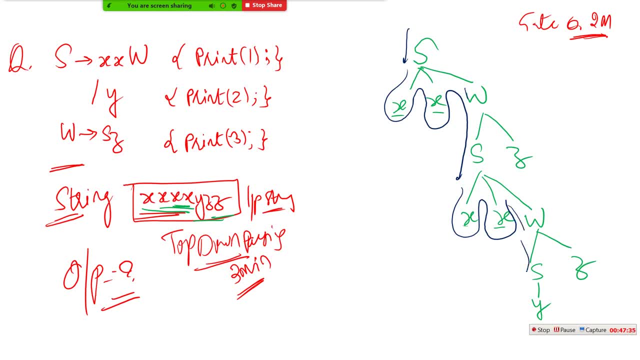 double x, but we don't have value of w as of now. but this s derives y, this s derives y. that is, this s derives y. that is second transition is generating. so this transition will print two first, because this is executed first, at the first position. this s is generated, this s is executed first. 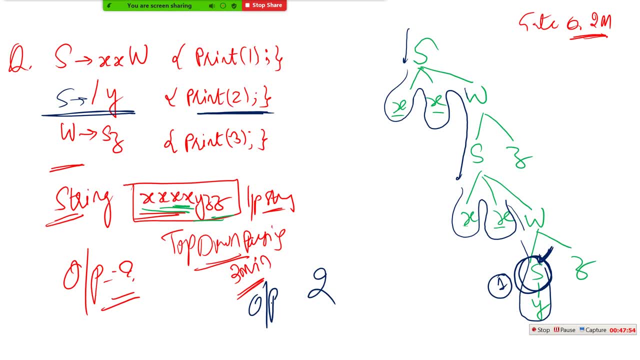 so this will print two as a output. i am writing output here. two will be a part of output. after that i will take z. but z is not not a single part of any right hand side production. so this s and z combinedly will give the value to this w. so this w is generating s and z means 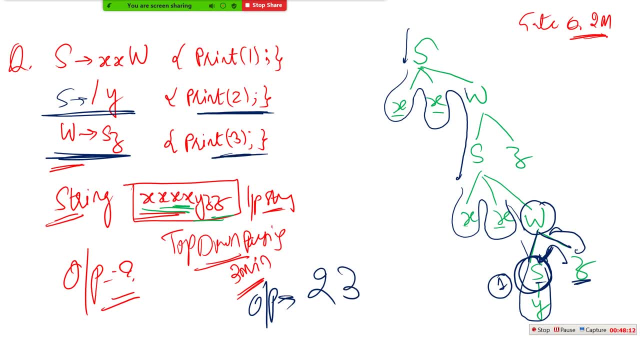 third statement is executing, so it will print three. because this s and z combinedly give the value to this w and now we have value of x, x and w because, after execution of this w, we have value of this w. so now this x, x and w will provide the value to this s and this s is x, x, w. that 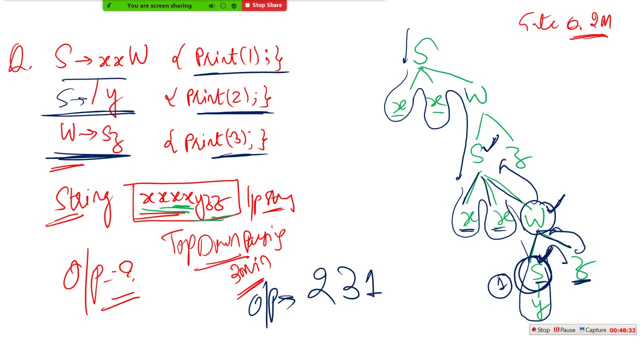 is transition one, that is, one will be printed now. now, after getting value of s, we will take z from third transition and this w will now again generate the s and z right. so again three will get printed and again we have value of w. now, that is we. 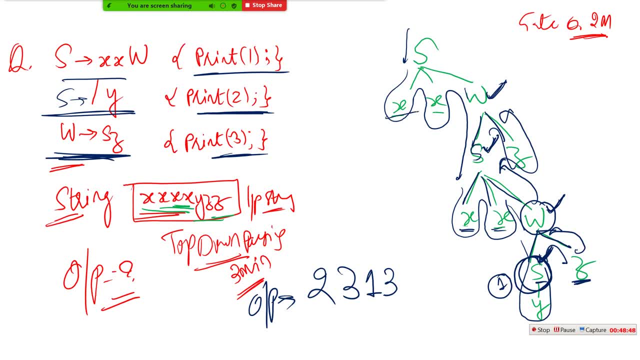 have derived from s and z by using top down parsing and now again we have x, x, w. so it will again generated by s and it will give one as output, because it is the statement one that is x, x, w. so two, three, one, three, one. it is the output of this. 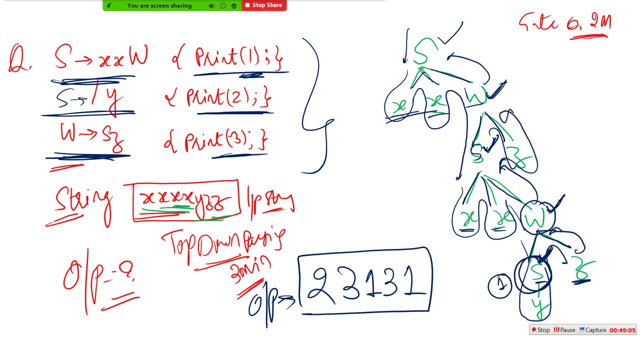 one will stay. is the error of this s? when this w is created from this, we will two, three, one plus zero. there is no issue, because we will have this вопрос. is this question이라고 statement? ciao, now we haveetten t Moiv문. 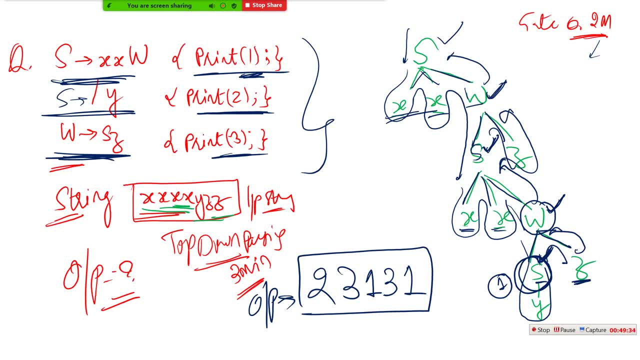 and now it is still here, and now it is three point parabola. now it is three point parabola. very good, very good. so if you are, if you have solved this question, okay, it is clear to everyone, very good guys, it is clear to everyone, very good. so now i am moving to. now i am moving to next. 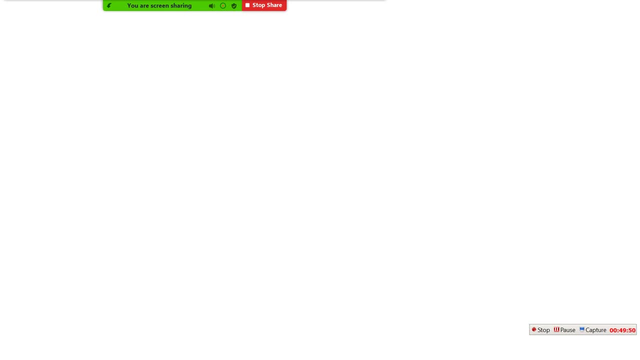 problem. it is also asked in gate and the problem is again, as it is given to you, that is syntax, directed translation is given to you. it is like: e derives e multiplied t and semantic rule is: e value equals to t value into t, e value into t value. okay, 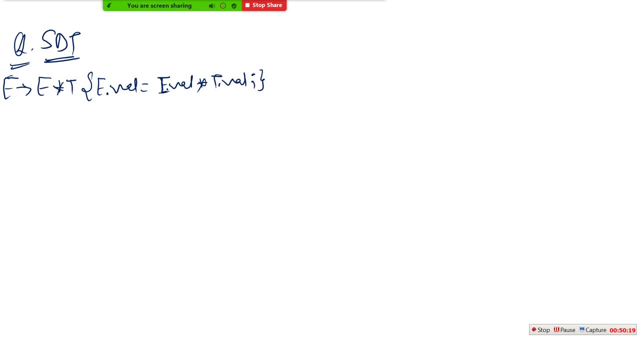 okay, and e derives t would be there, and okay, and e derives t would be there, and okay, and e derives t would be there, and e value equals to t value. now, okay, and again we have t derived f subtraction t and it here. t value equals to f value subtraction. 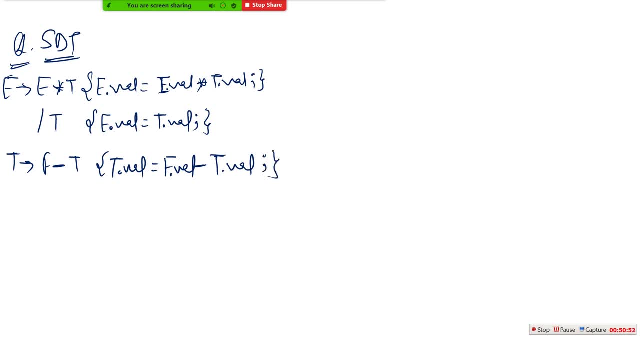 t value and we have have F and it will generate T value equals to F value. it is a question which I am given give giving to you. and F is generating 2 and it is also generating 4. it simply means that F- will you help 2 and it simply means that F value equals. 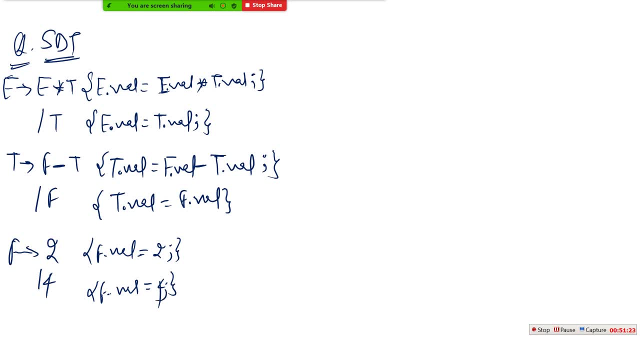 to 4. okay, so it is a SDT, that is, syntax directed translation. I have given to you now a string: is 4 minus 2 minus 4 multiplied 2. it is the input string. guys, it is the input string. now, while solving it, while in, while traversing this input, 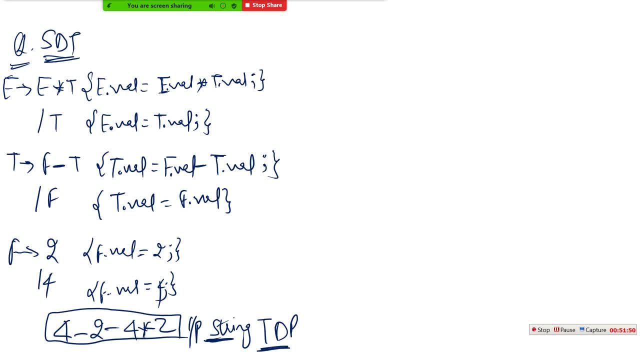 string using top-down parser. using top-down parser, what would be the answer? using top-down parser, if we will traverse this string, what would be the output? you need to answer me. what would be the output if I will traverse this input string. that is 4 minus 2, minus 4 multiplied with 2, if I. 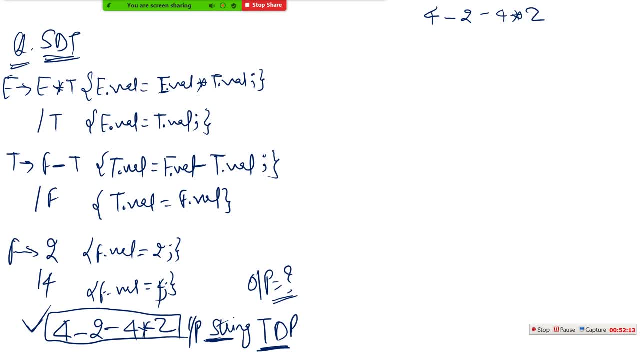 will traverse it using top-down parser technique. what would be the output of this? I am giving you guys four minutes to solve this problem. it will you guys four minutes to solve this problem. it will make you may feel somewhat lengthier, but it is not that much lengthier. 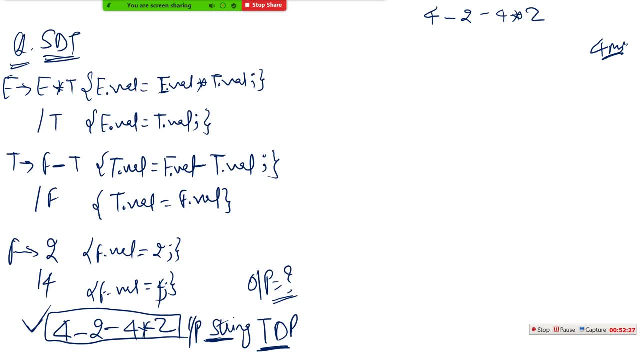 make you may feel somewhat lengthier, but it is not that much lengthier. you just need to answer right. you always need to start from starting symbol and check manually that whether we are able to generating this is thing or not. if you are able to generate this string means you are correct, so we need to. 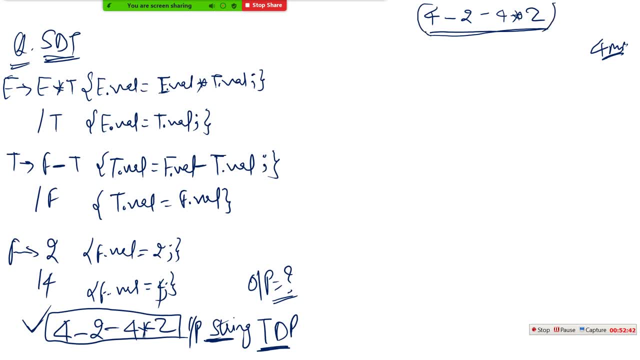 answer this using- we need to answer this using this asating, using this sdT, we need to generate semantic tree and by semantic tree needs to be white on the orich Verm trail right. while pronouncing that way and marque, I will the penguin form the laatis three and we willALLEN. 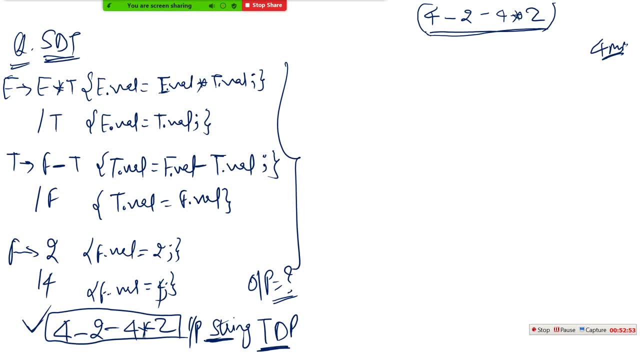 you will give me the output and yesterday's some important concept will always- all will always- be clear with this example, because it is very, very important problem, and you will understand all the compiler design concepts from this, from this problem, you will get understand all important concepts of compiler design and SDT. so please solve this. I am giving you four. 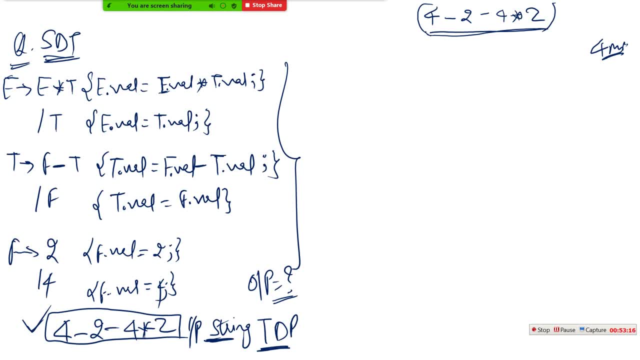 minute to answer that. what will be? the output will be generated in respective of four minus two minus four into two. you need to answer me, okay? Piyush has answered it. good, I am expecting other candidates as well. please answer it as early as possible and then we can move to next problem. then we can move to next. 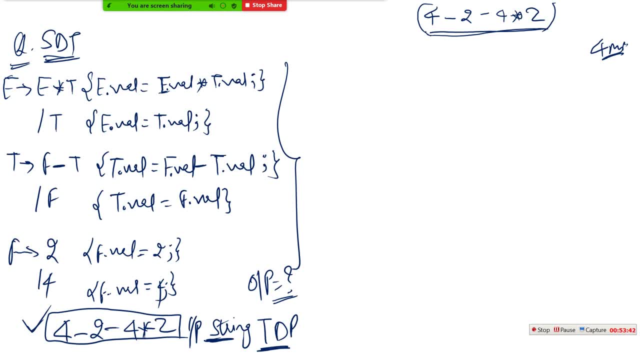 problem because it is very important. problem guys, very, very important and it's interesting, problems which I am discussing it with you. you, gate problems is row problems and bar problems, this all are part of this. problems, right? so one by one, place all this and after that we can take some. 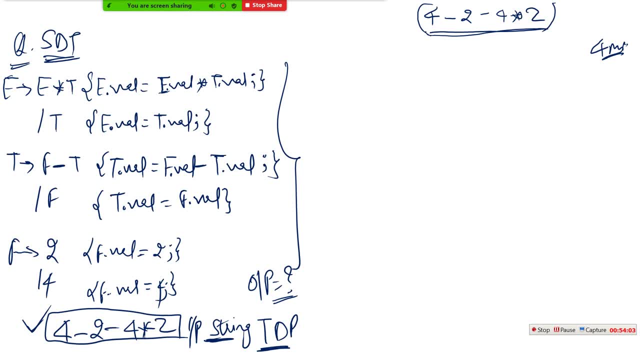 more problems of gate and previous year CS exams. only Piyush has answered it. I am requesting other candidates as well that please be interactive with us. please apply your approach of the SDT concepts and answer this question. students have asked you if the question is correct. if the question is accurate. 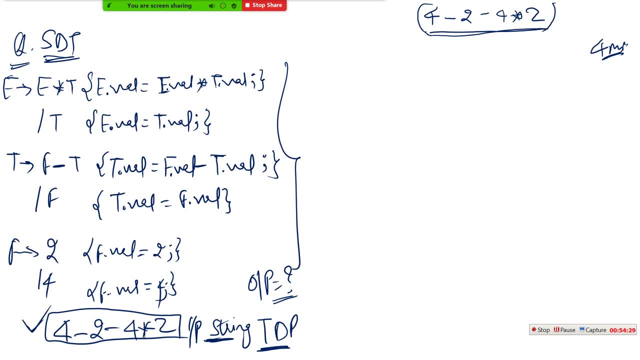 should not be the question you can express in your effectivement. answer is very clear. use that question, Piyush. please answer all the points. 그러니까, if you got correct answer, you can quickly have the start with the answer one by one. please reply down haciendo. 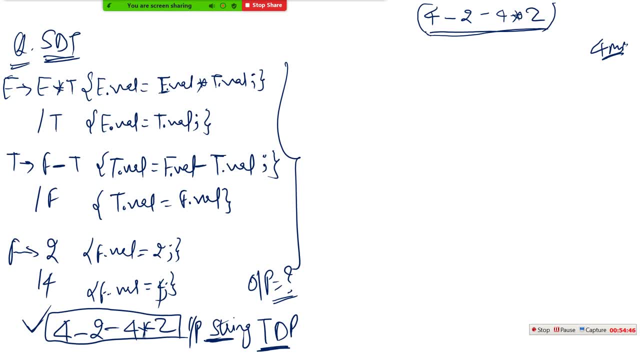 an kind or an expected answer, but if you need an answer, you can ask question. it is saying: if you have not answered the question, do not tell me the first of your questions due to this, and you will answer it simply like the ones, which are very well. 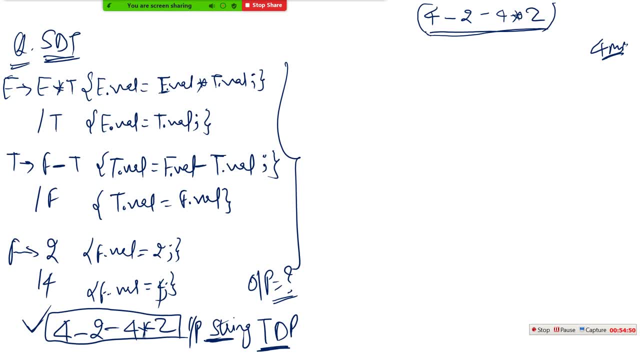 answered. very good, Piyush. if you have not answered the question answer, choose the following: what about other candidates? are other candidates also trying? please respond me. very good, manjit. i am giving one more minute for other candidates. please solve. answer it in the chat box, so. 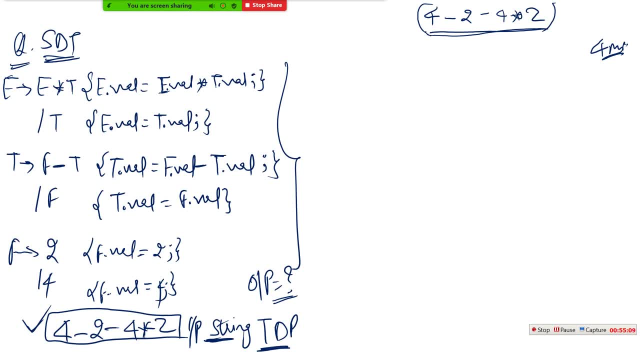 that i can understand that you are practicing it, because until and unless you are practicing it, it will, it is, it will be only beneficial for you. only if you are participating in the chat box, if you will be interactive with us, you will ask your doubts and queries as much. 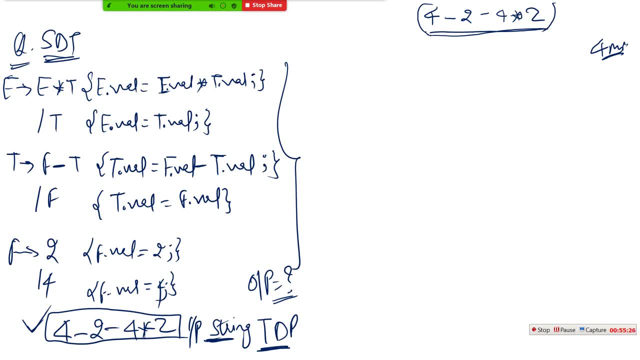 as you will be interactive and ask your queries, it will gonna beneficial for you. so solve all the problems which i am discussing with you. discussing with you because from previous four to five years, if you will solve such problems and assignment papers which i will share with the admin of. 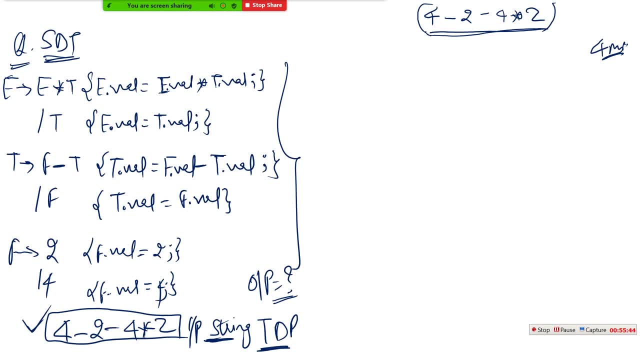 this schedule, so you will hundred percent gonna score in this subject. so i am requesting other candidate as well. please answer. this is other candidates trying. yes, just twenty more seconds, guys. after that i will discuss the solution in detail. after that i will solution in the detail. i will discuss the solution. 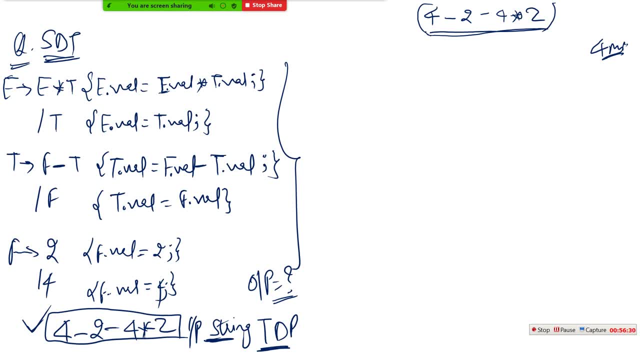 in detail. so please answer it, guys. please answer it. vipak, yes, vipak, yes, you okay guys, okay guys. it's enough time that i have given to you. now i am solving the problem, guys. what we need to do now, we need to start from the initial, initial starting symbol, whatever our 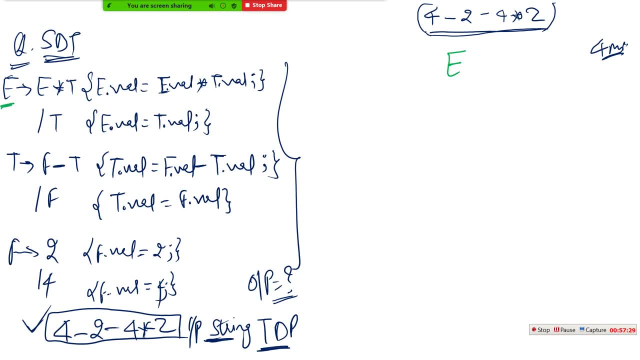 starting symbol. it is the rule one. rule one is that we always need to start from. we always need to start, we always need to start from starting symbol, and our starting symbol is e. so i have started from here. now. next one: is that what i need to do? i need a subtraction here, but 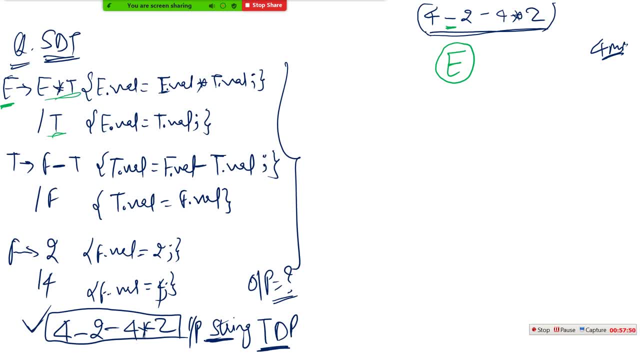 i don't find any direct transition from e, which consists of subtraction. i only have e multiply with t or t. so what i would take, i would rather take e multiply with t because i don't have any subtraction. so what i will do? this t, this t or we. i can generate e from this t if i will generate. 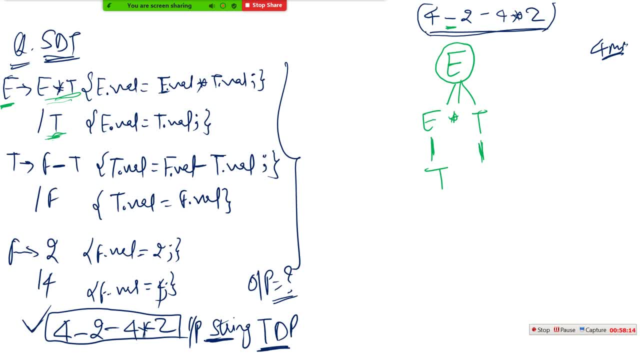 this: uh, this t from this e. this t will further give me this transition that is f minus t, so f minus t. i have generated from this t using this transition and after that, if you will observe what i need, two minus four means i need. i need one more transition. 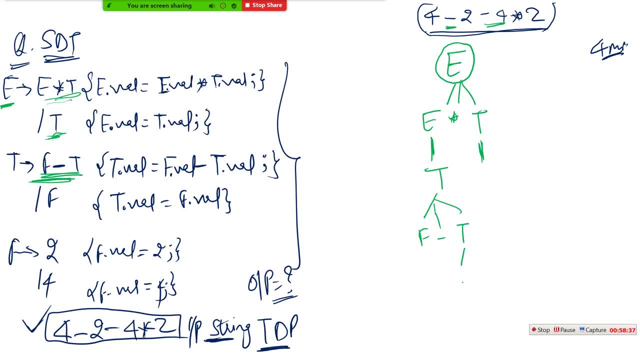 so this t, this t, will fetch me the value of this t will fetch me the value of f minus t, again, f minus t, again i took it from here- and this t will take value f and it will generate value. so what i need? i initially need four, so i will take four from here, then two, then four and then i i will fetch value. 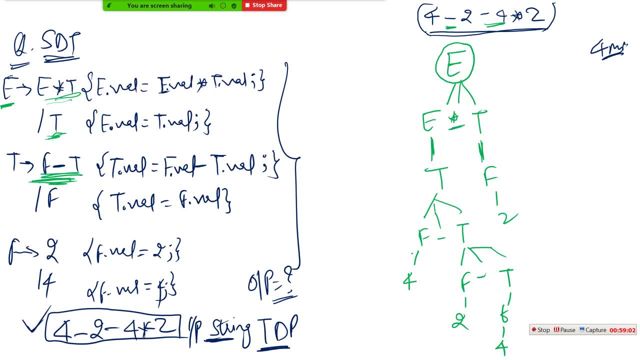 of two from here, because i need just multiply. i use multiplication here, so the remaining part would be done from the left hand side, and then this multiplication would be done on this basis, guys. okay, now i am traversing it after making semantic tree. i am traversing it, guys. 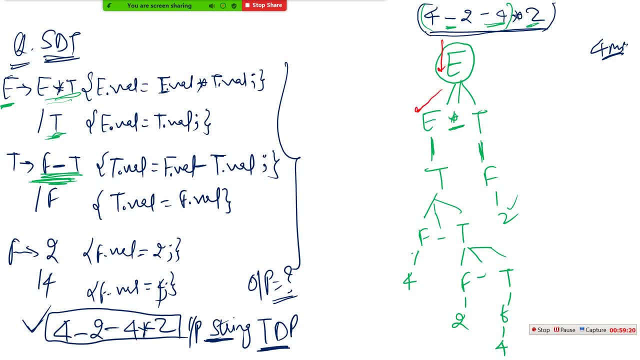 So I will start from here E. I will traverse to this E. I don't get any value. I am traversing to this T. I don't get any value yet. I am traversing to this F. I don't get any value yet From this 4, from this F, I got value. that is 4, which is passed to here. That is 4.. I got 4 here. 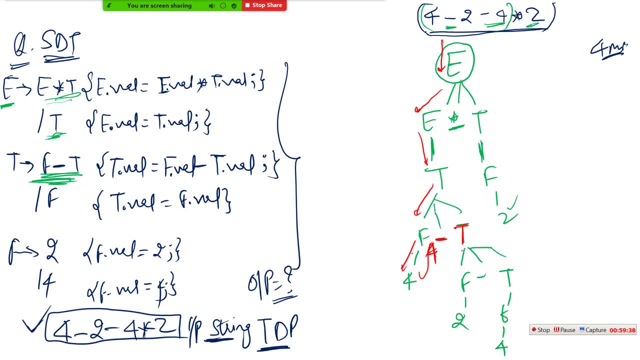 But I need to subtract here from the value of T. What is the value of T? T is deriving F minus T. Now I need F minus T. Whatever the value of F minus T would be there. we would take the value of this transition here. Right Now this F is generating value 2. This will be passed here And this T is now I need to subtract it from the value of T. What is the value of T? It is the value of F. That is value of T is value of F. So this value of F is 4.. 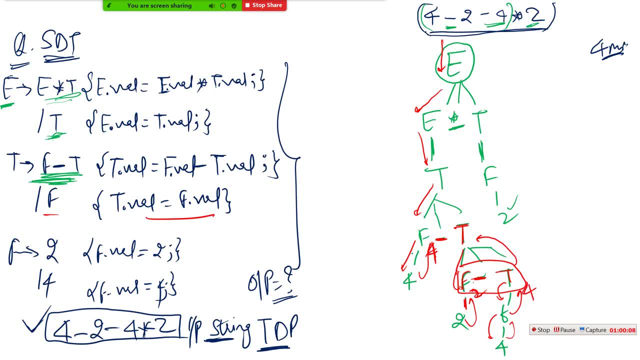 4 is passed here, 4 is passed here And 2 minus 4.. 2 minus 4.. That is minus 2, will be passed to this T. So this 2 consists of value minus 2.. So if you will observe here, If you will observe here: 2 minus 4.. That is this transition: 2 minus 4.. It is generated first. This is: This is generated first: 2 minus 4.. That is minus 2.. This transition is generated first. I will also tell you that why it is generated first. Now, 4 minus minus 2.. 4 minus minus 2.. 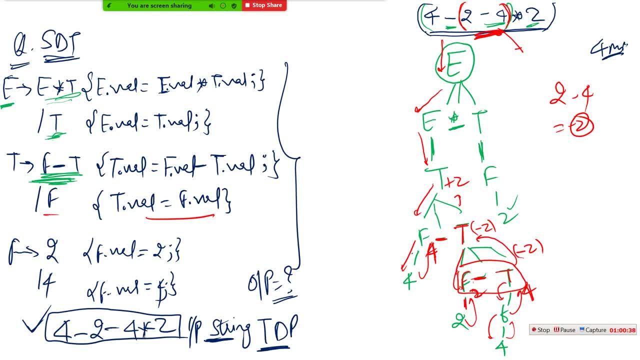 That is plus 2 is given to it. 4 minus minus 2.. That is plus 2 is given to it. So this T now have plus 2.. Right Now, the value of minus 2 here Now next one is 4 minus minus 2.. 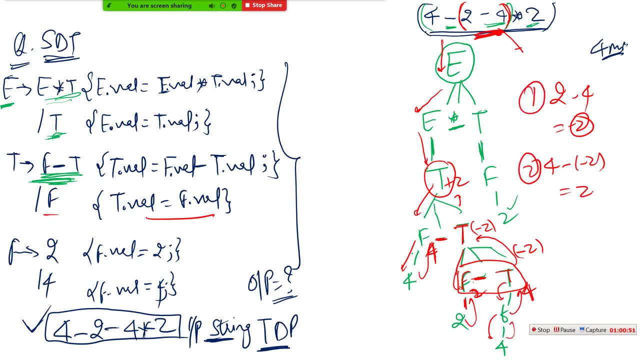 So in first step I got that. In second step, what I got, I got plus 2.. And after that the value of this 2 is passed to this E. That is, 2 is passed to E. That is E equals to value of T. from this transition. 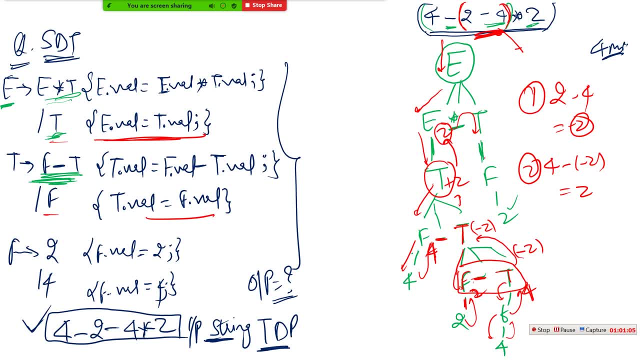 Now I will traverse from the right hand side part of this semantic tree And I will get the value of F as a 2. And this value of F will be passed. T will be equals to F value. So this 2 is passed to here. 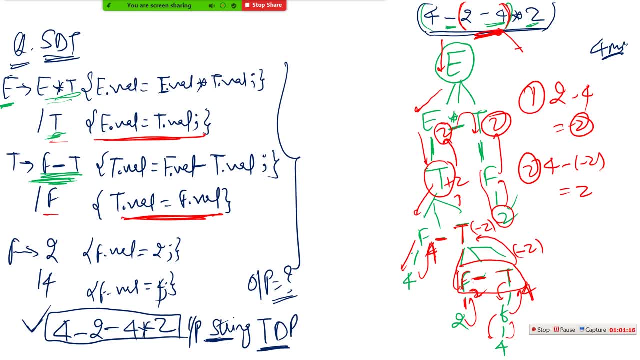 And this 2.. 2 will be passed to here. Okay, guys, This 2 is passed to here. And if this 2 is passed to here, You can simply say: This 2 is passed to here. And now what I need to do? 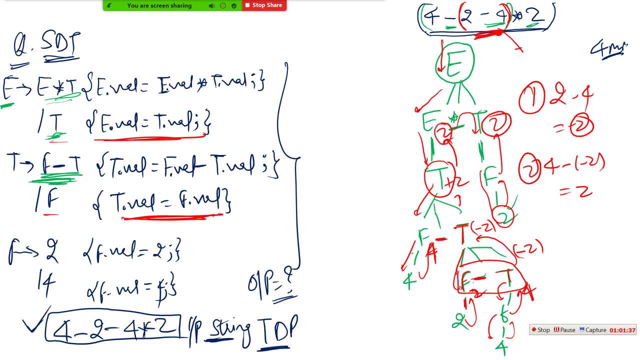 I need to. I need to multiply this 2 with this 2.. So 4 will be resulted And this E will generate value 4.. This E will be generated value 4.. So what is value 4?? What is the value 4?? 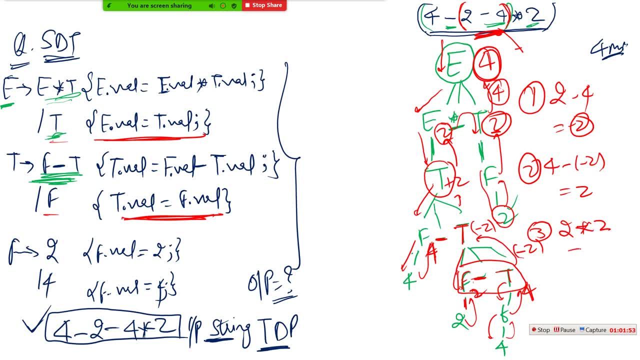 So at last, in third transition I got 2 into 2.. That is 4.. So output of this transition would be 4.. Now, most of you candidates, what you done, You generally done. You just multiplied. 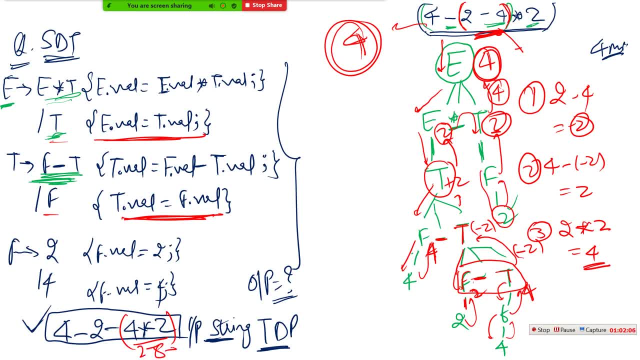 You got 8.. Then 2 minus 8.. 2 minus 8.. You got 6.. What you done? I don't know That what you have done and how you done Right, How you got 12, guys. 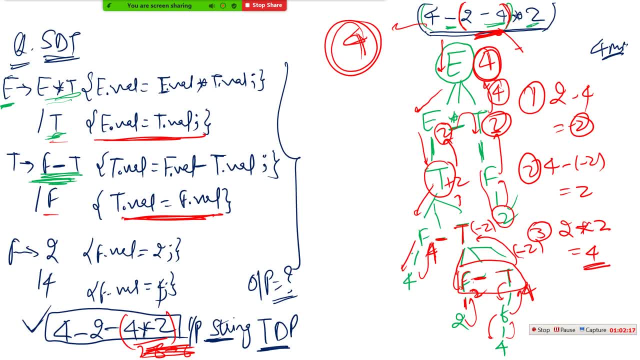 Okay, Nikhil is saying: sir, 12 is the answer. Let me do it. Let me do it guys. Let me do it. 2 minus 4 minus 2 is there, And minus plus minus. Okay, guys. 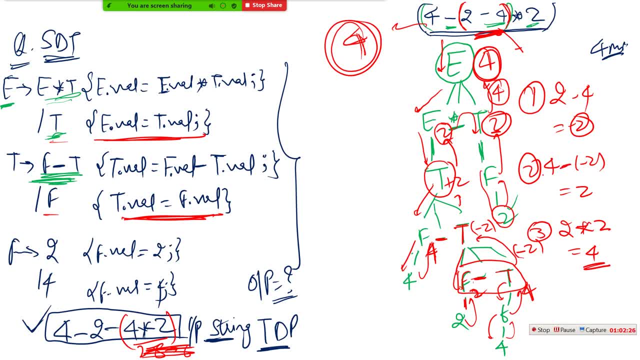 Here minus plus minus. What then? 4. Here 2 was there, So 4 minus minus 2. 6 would be there. So this 6 would be passed to here. So E consists 6 as a value. 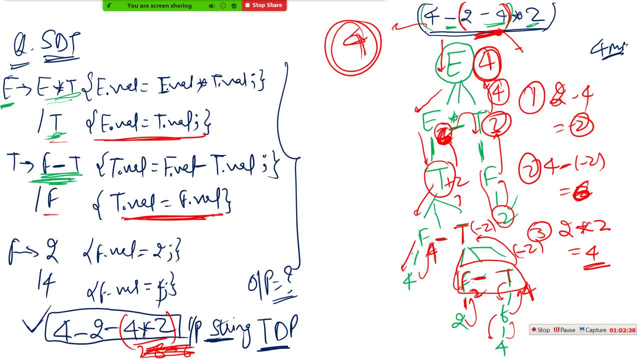 And 6 multiplied with this, 2 will be passed here. So 6 multiplied to 12 will be passed. 12 will be passed. So this E will generate 12. as answer Why? Because here we take plus 2.. 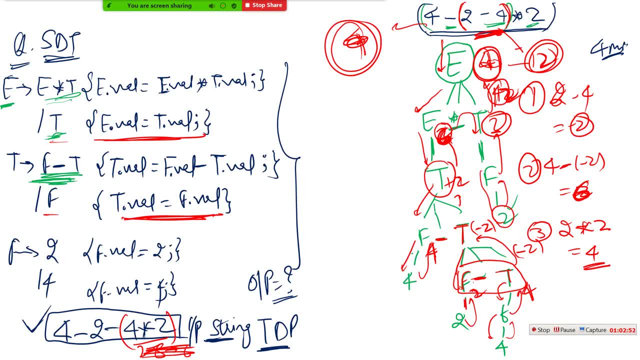 But here, if you will observe, we have gone minus 2. And here we already have minus. So 4 minus minus 2.. So 4 minus minus 2, that is 4 plus 2.. It is nothing but 4 plus 2.. 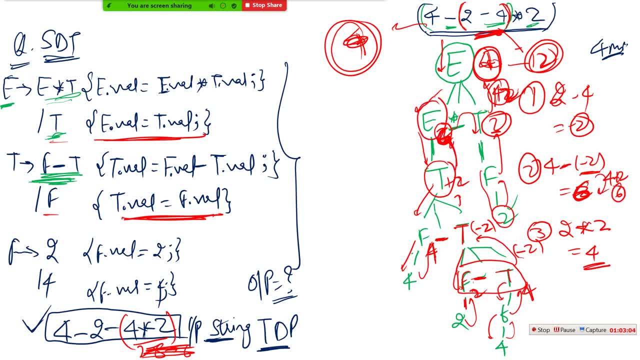 So we got 6.. And this 6 has passed as a value. So we got 2 from the value of this TN. 6 and 2 multiplied So we got value 12.. So we got 12 as answer. 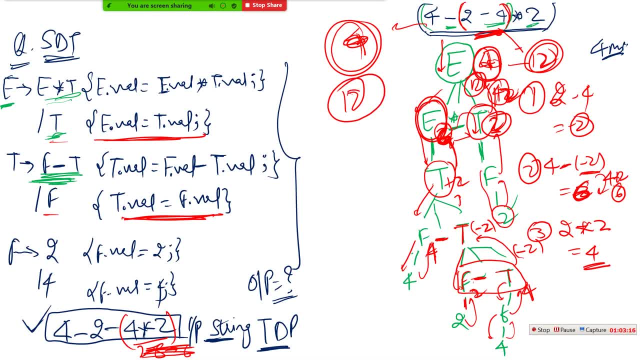 Now, guys, one more problem I want to discuss. in it That you can simply observe that first we have generated the transition, First we have generated the transition 2 minus 4.. That is, this transition has generated 2 minus 4.. 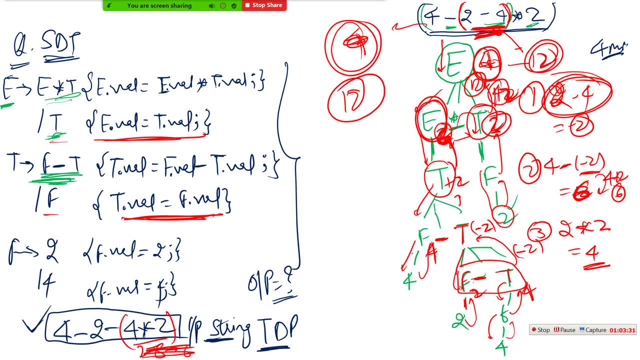 Why it is done? Because, if you will observe this negative sign, that is this subtraction sign, this subtraction symbol is in the bottom most place of the sequence. So I told you earlier that whatever symbol we are finding in the bottom most side of the grammar will be given to the higher precedence. 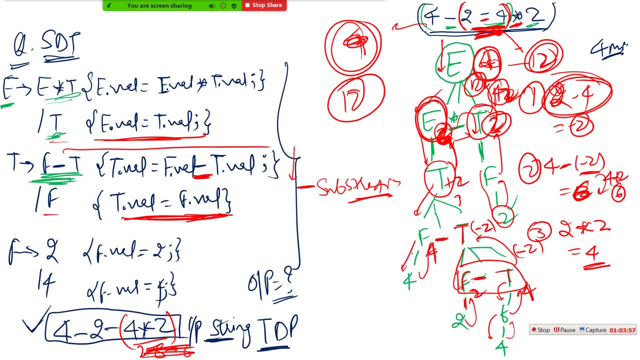 So, among multiplication, in this subtraction, we have given higher precedence to this subtraction symbol. Why? Because it is placed in the bottom, most side In this semantic tree. you can observe it. Whatever we have discussed yesterday, it is the proof of that. 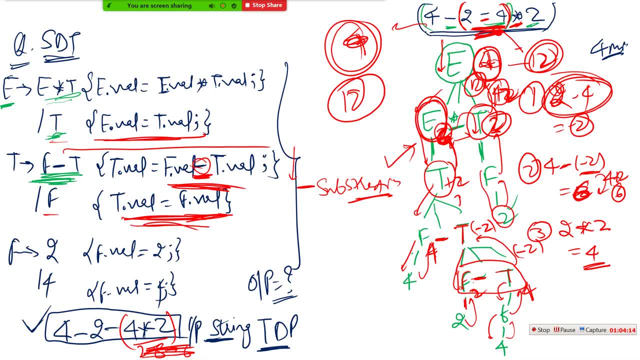 That whatever placed in the bottom most side of grammar will be given highest precedence. This is the part of ID. ID will be given highest precedence in operator precedence parsing table. Why? Because it existed in the bottom most side. So if it existed in the bottom most side, we have executed this one first. 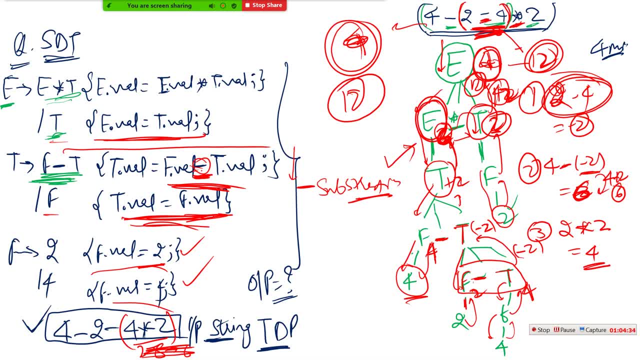 But among multiplication and subtraction. you will observe here, this subtraction is existed downside this multiplication symbol. That is why the precedence of this subtraction symbol is higher. The precedence of this subtraction symbol is higher. Now, why we solve this subtraction first? Why didn't we solve this subtraction first? 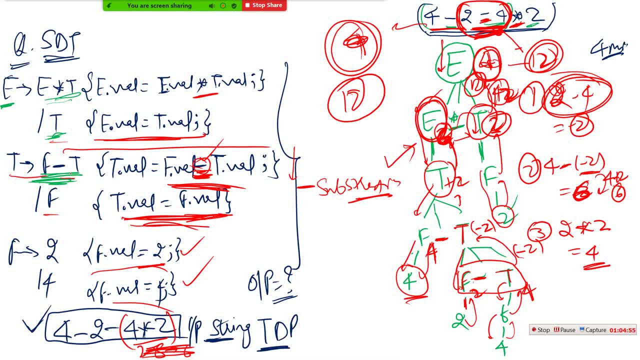 Because you will observe, here t derives f, dot, t. So this t, that is the left, most symbol of this t, existed on the right side, Right side of this t, this subtraction here, this left factoring on the right side of this t. 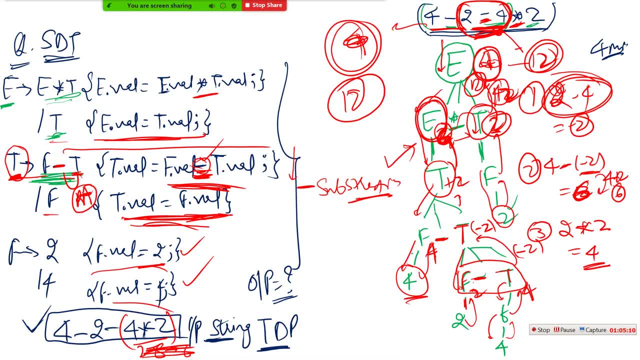 that is why you can say that we have right associativity. There is right associativity relation with the subtraction. So we have did right side subtraction first, After that we have performed this subtraction And after that we multiply. So, guys, we find 12 as the output of this problem. 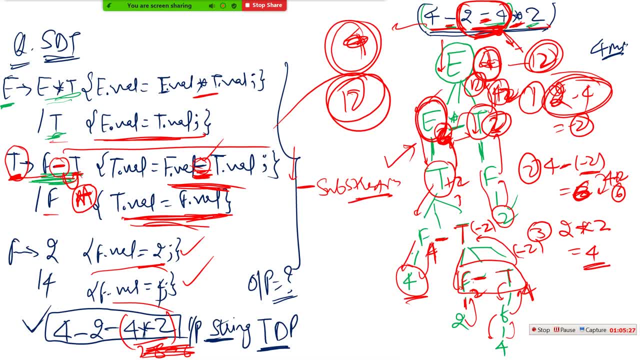 Is it clear to every candidate guys? Please answer me, Please respond me. Is it clear to every candidate? Is this problem clear to every candidate? Please answer me, guys. Is it clear to every candidate, guys? Is it clear to every candidate, guys? 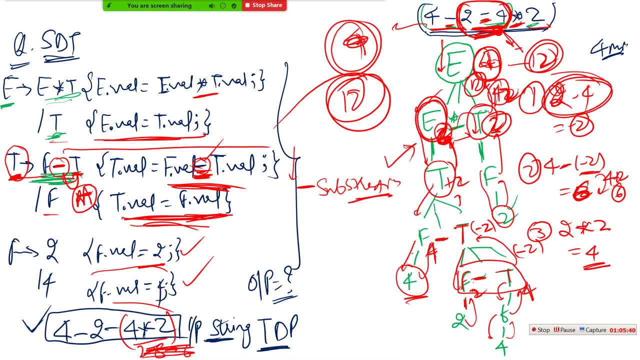 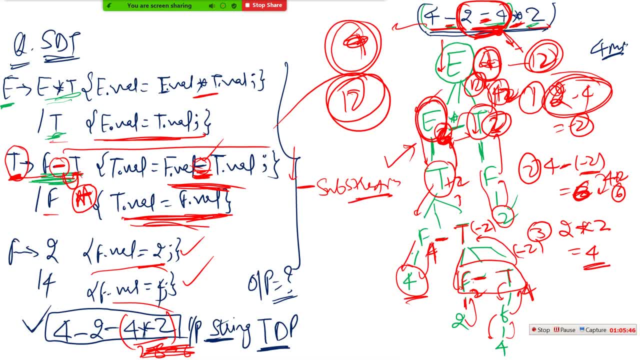 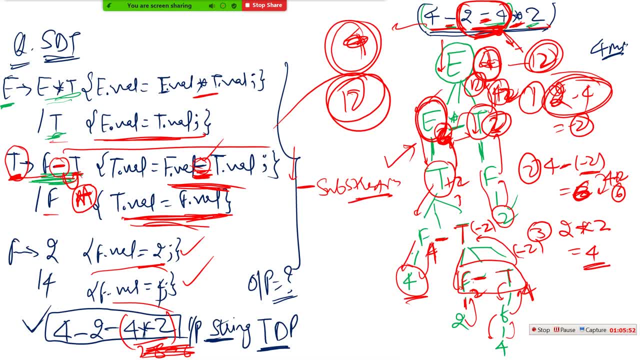 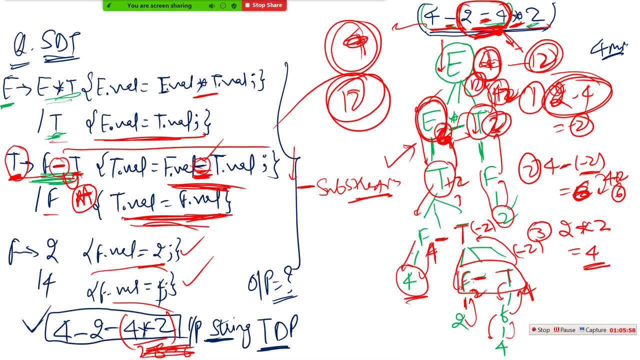 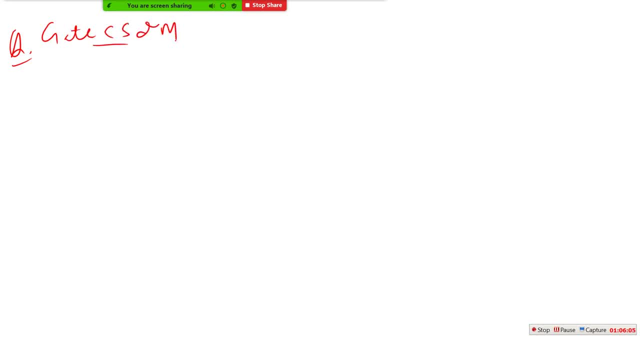 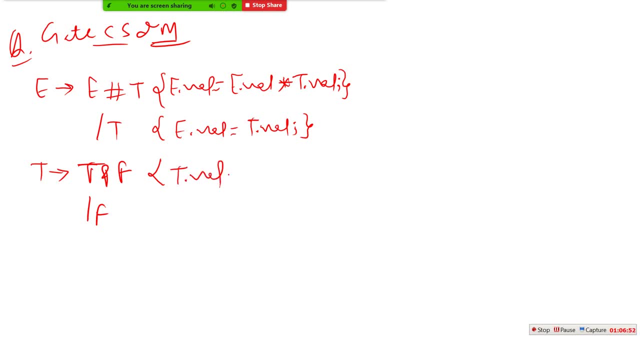 in a semantic rule of this is t value equals to t value plus f value, and semantic rule for this is t value equals to f value. after that i have generated, f derives num and it have f value equals to num dot l value. okay, guys, now question in front of you is that you need to find the output for. 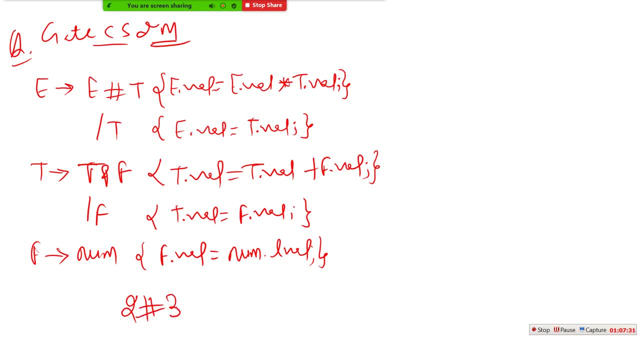 the respective string. the string is 2- hash 3 m percent 5. hash 6 m percent 4. this is the input string. guys, this is the input string and you need to answer me. what is the output for the following string? it is the gate, two marks. 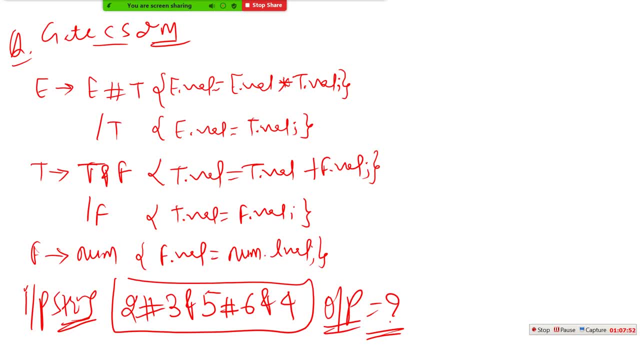 problem asked in numerical section. in numeral section they have asked in two marks. the question is: this string, that is, 2 hash 3 m percent 5 hash 6 m percent 4, it is passed as a input string and we need to answer. we need to answer that. what is the output of this string? what is the output of? 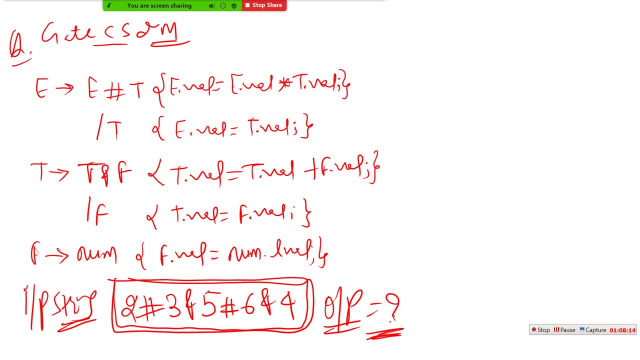 this string. i am giving you guys three minutes. i am giving you three minutes to answer. after that i will discuss the solution. i am expecting every candidate to answer it. very simple problem for two marks under gate computer science. please answer me, guys. so very important problem of gate computer science. please solve it. 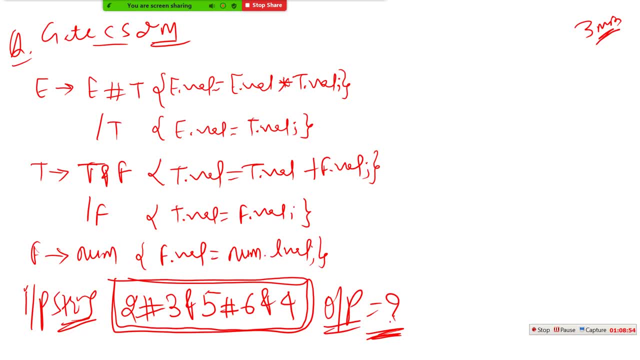 and answer me that what is the output you are getting in respect of this input as a string? so, so, so, so, so, O, so, so, so, so very easiest problem, just you can add. you can solve it earlier as well. okay, here she is getting answer. good, i will verify the answer while solving the. 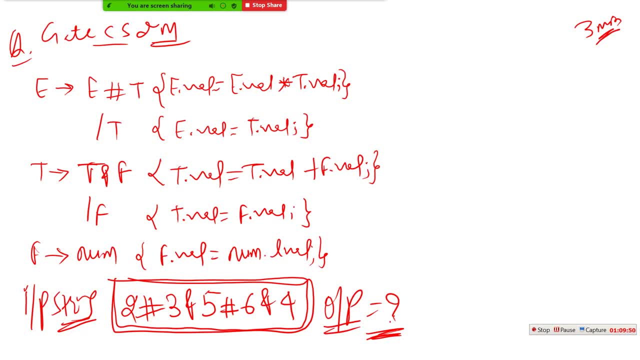 answer is very easy as well. okay, here she is getting answer. good, i will verify the answer while solving the question. i am getting answer very easy, so the question don't worry what I need to generate. I need to generate 2 hash, 3 M percent 5 where 6 M percent 4. okay, and it has also answered. okay, I am expecting. 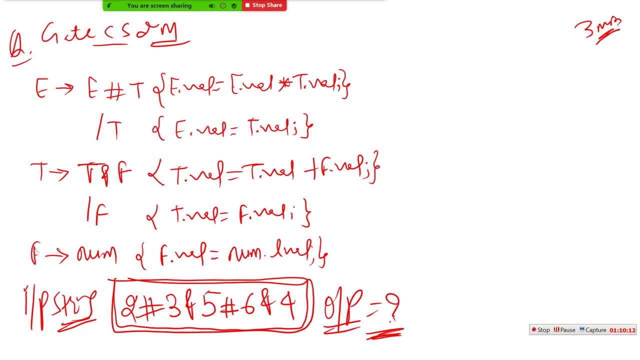 other candidates to answer it as well. after that I will discuss the solution. you you, Piyush has also answered it. okay, I got an answer from 3 candidates, who total 3 questions that I have gotten I don't know for which形. Hey, outside the same curve, don't know how to do that. very better, who lost? if I don't see more, then I'll answer needed. okay, I got my answer from 3 candidates. 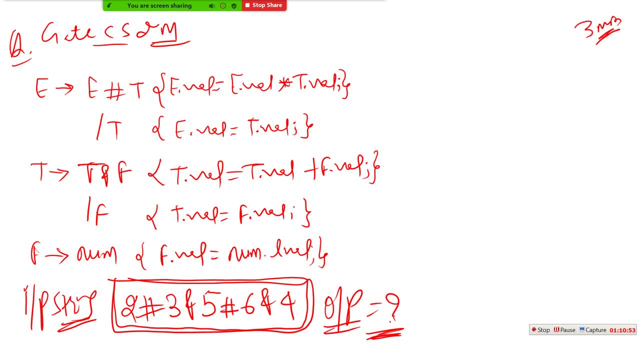 Yash, Ankit and Piyush. and Poshali has answered it. okay, for four answers I got till. I am expecting other candidates as well. please answer it, then I will discuss the solution. you, my name, is Ankit, and I am expecting other candidates as well. please answer it, then I will discuss the solution. 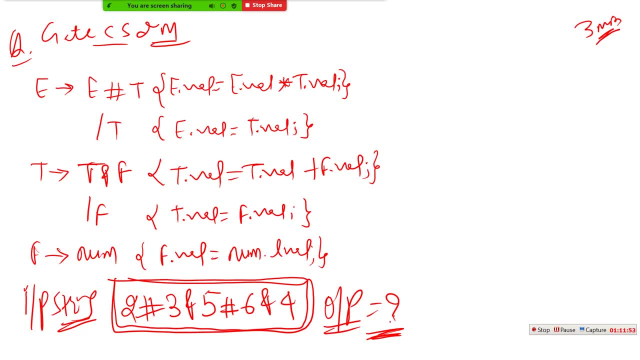 Ankit has also answered it. okay, Somya has also answered. okay, guys, now I am discussing the solution because almost all the candidates answered according to them, but still I am facing that many students has answered differently, so I am discussing the solution once again. so, guy's, the problem was same problem was very easier. I need to answer. 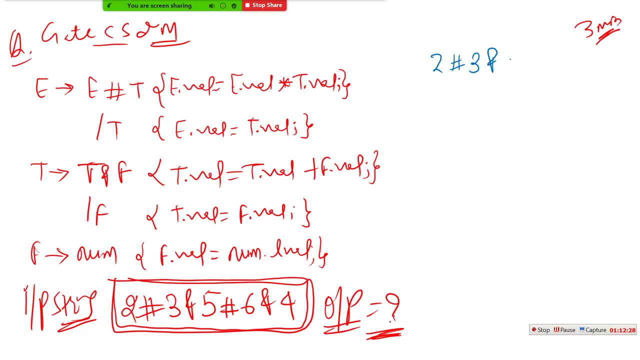 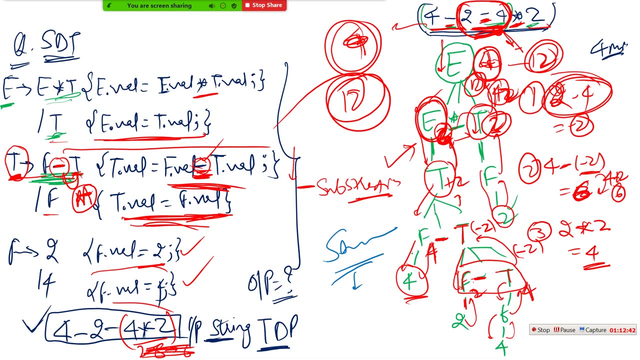 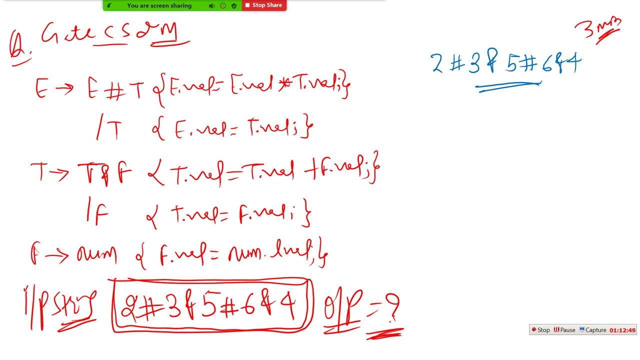 two hashe, three M percent, 5 hashe, 6 appetizers and four. so we have discussed complete procedure here in previous problem, how to make semantics tree and then solve: i levar keôm, but now you can answer it using shortcuts, using shortcuts, using shortcuts, you can answer. 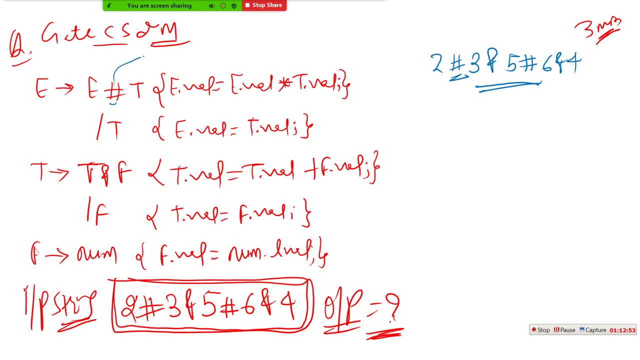 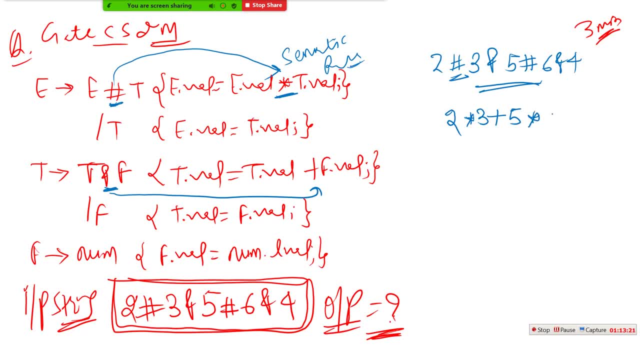 three plus five, again h means multiplication and six and again m percent means plus right, and six m percent is plus, so four. so ultimately, this s symbol is representing multiplication symbol and this m percent symbol is representing addition operation. so i hope you are getting this. so we just need to answer this now. now, no need to make semantic tree, because in 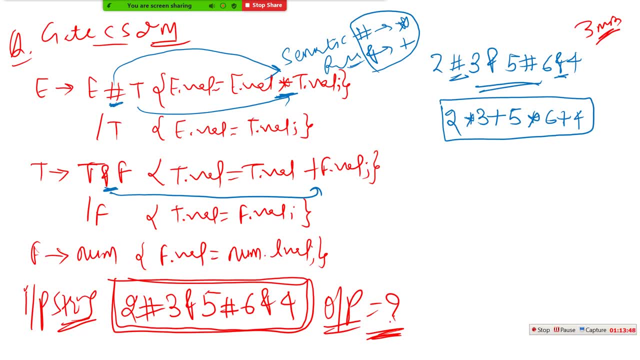 gate exam. if you will apply shortcuts, if you know the concepts of compiler design, that how compiler is processing with this, it will gonna very useful for you. so we first need to answer that among, among, among multiplication operation and addition operation, whose precedence is greater? whose precedence is greater. so you will say that this plus symbol help, greater precedence because 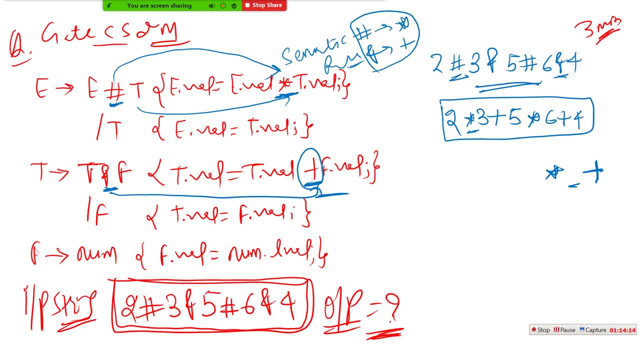 it is existed in the bottom side of that star. the star is a greater precedence of the previous upper side in the transition level and plus is existed in the bottom side. that is why the precedence of addition operator is greater. the precedence of addition operator is given. it is. 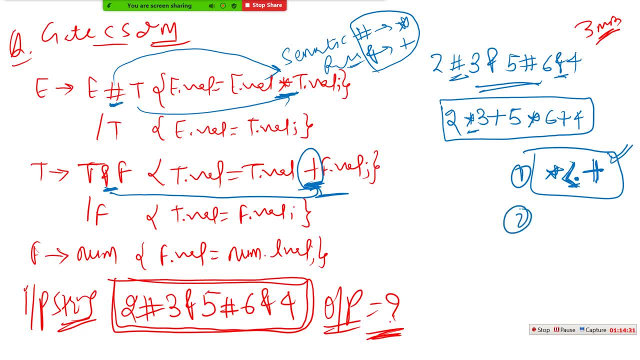 first deduction which i have derived. now, second deduction is that plus is left associative or right associative. so if you will see, t value equals to t value dot plus. so my whatever i am having in as a non-terminal in the left hand side, i am having it on the left side of the plus. 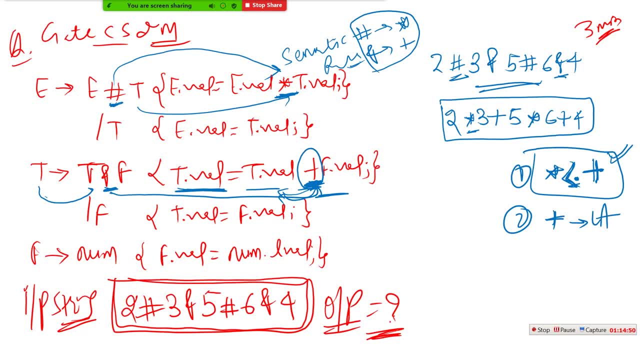 operator. so plus is my left associative, this plus is left associative. and third is: what is my multiplication operator? so this uh multiplication operator, i am having e value equals to e value, dot, t value, that is. i also have this multiplication as a, as a left associative, so my both 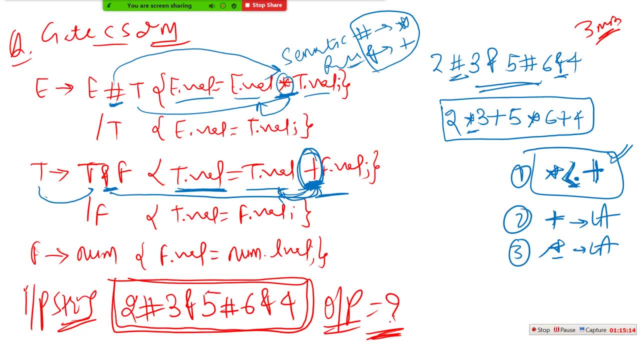 addition operation and multiplication operation are left associative. now plus will be evaluated first, but left plus will be evaluated first. so 3 plus 5, that is 8. now i have my equation like: 2 multiply with 8 into this 8, this operation will be added again because this is plus but left. 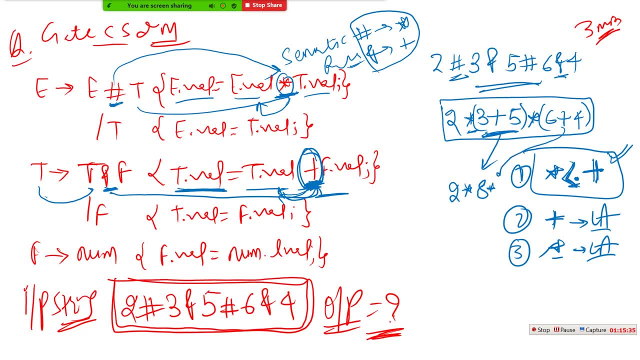 associative. so i have calculated it first. after that i will calculate: 6 plus 4, that is, 10 would be there. now there is no need to apply associative between multiplication because whatever the associativity of multiplication, it will not impact. so simply you can say 8 into 2, 16 into 10, that is you are getting 160 as a output. we didn't make any. 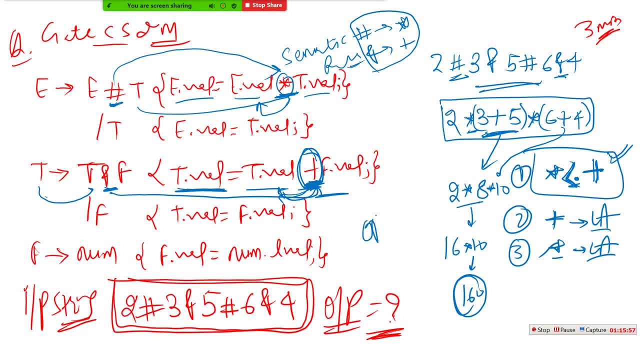 semantic tree. we just answered it using the rule of operator precedence table and the associativity of the operators in using simple concepts of sdt. so 160 would be the output of this problem. this is the gate to max problem. guys, this problem is clear to everybody. please answer me. 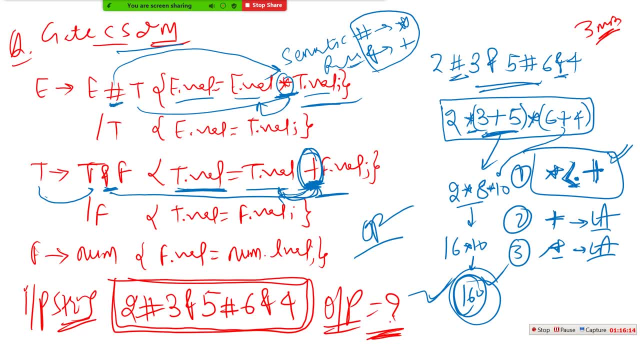 is this problem is clear to everybody? please answer me. okay, guys, it is clear to everybody. very good, very good guys, it is the shortcuts you can follow. this is this was the shortcut you can follow. right, it will save your time. but the role of the semantic trees if you are getting some problem in. 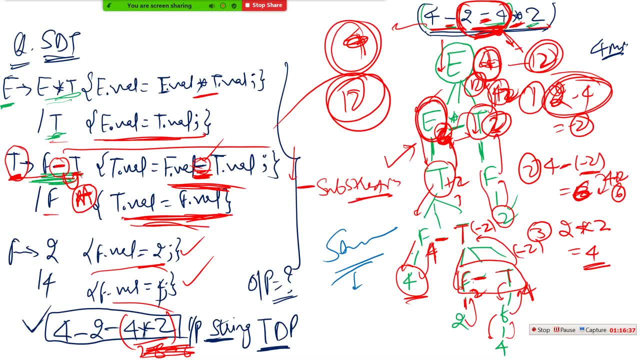 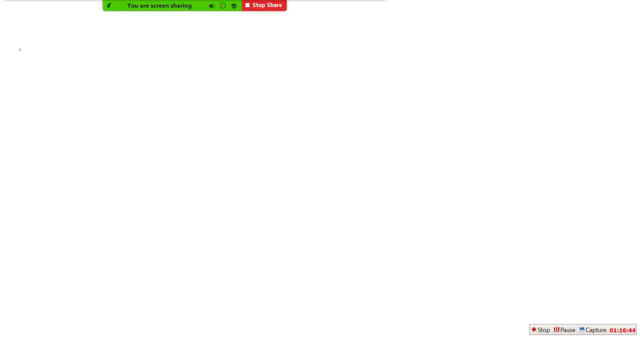 which you are getting stuck. you can try with semantic. so we have discussed it with the procedure as well and we have also discussed it with the shortcuts. okay, okay. now the next problem is isro's problem. i am discussing isro cs problem with you. from sdt, my grammar is it is derived a s. again, s derives a, b, a derives a small a. 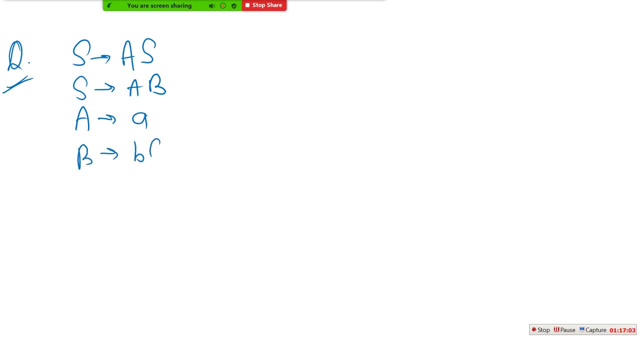 b derives b and c. this is a non-terminal. and further, my b once more derives d and b and my c derives a small c. it is a terminal. now, this is terminal, this is non-terminal. okay, don't get confused on that. now the semantic rules is: it will print one, it will print two. 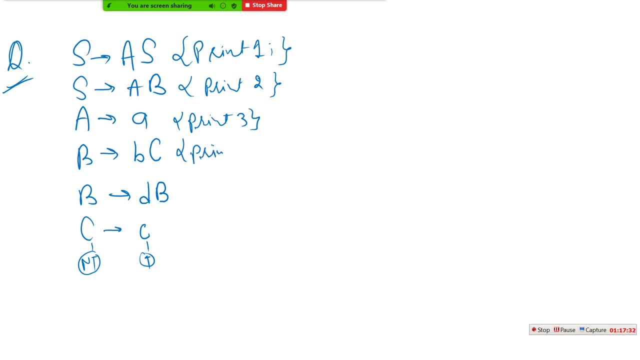 it will print three, it will print four, it will print five and this transition will print six. the input string- the input string is input string- is triple: a, d, b, c. this is the input string. guys, this is the input string. answer me, answer me what will be the output. answer me what will be the output. answer me. 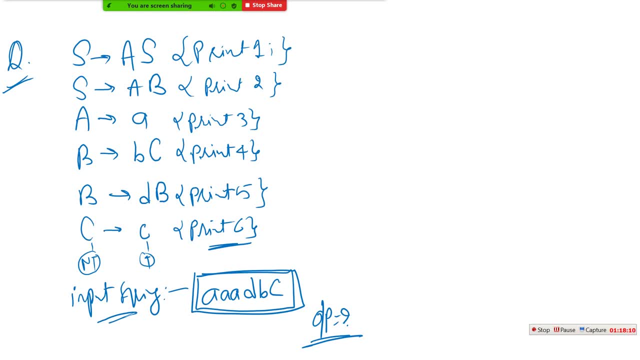 what will be the output? and also, to answer me, it will revise your concepts. how many handles, how many handles you are getting while parsing this string on this grammar, parsing this string on this grammar, what is the output and how many handles you are getting while solving this? 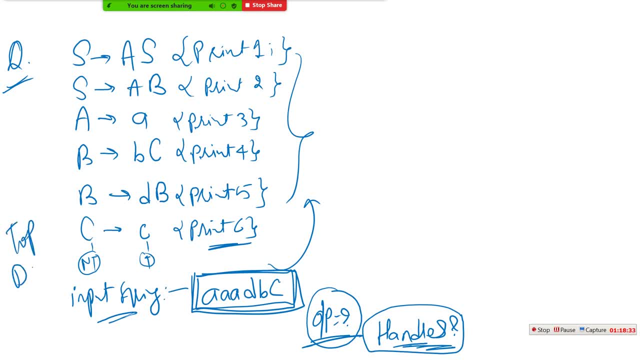 using top down parser using top down parser. guys using top down parser using top down parser, what is the output and how many handles you are getting in semantic tree? please answer me. i am again giving three minutes so that you can answer it. it is very easiest question of. 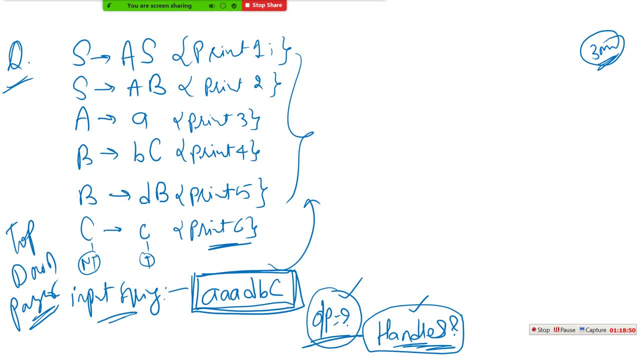 isro, please answer me. no, yes, it seems lengthy, but it is easier. it seems lengthy, but it is easier. please answer me. you can solve it in two to three minutes. it will not take that much linear. please solve it. you just need to answer that. what would be the output using top-down? 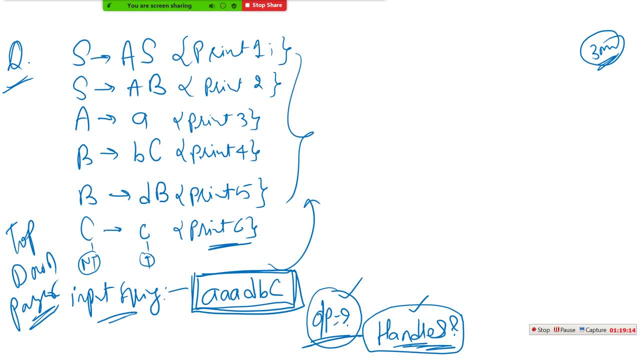 parsing you. okay, if you have made parse tree, then answer me what is the execution order of output? what would be the print? what would be the output of this SDT? what would be the output of this SDT after drawing parsing tree, just parse from top down, from top to down, pass and answer me that. what statement you are getting? what? 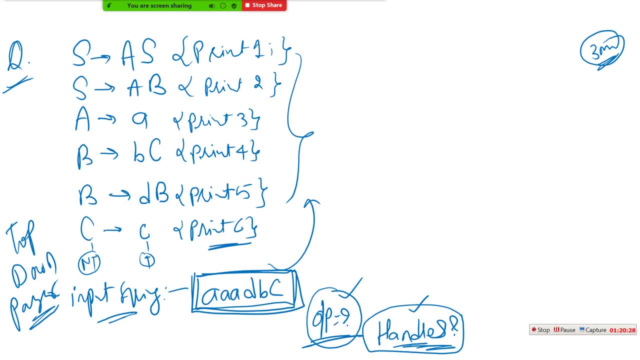 output you are getting one by one from top to down. this one is so computer science paper question from previous year and very, very important concept: you, after parsing, after making parsing tree, or semantic tree, after making semantic tree, after making semantic tree, just applied top-to-down passing and in that 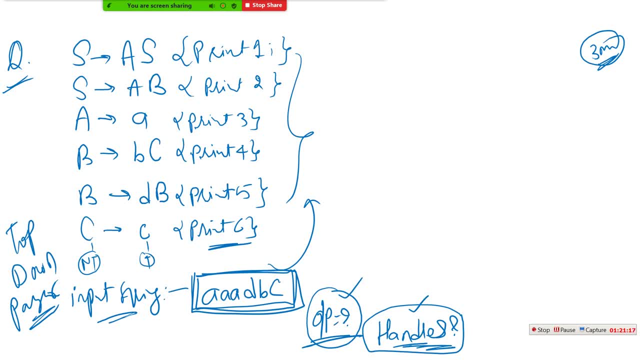 top-to-down passing. answer me that, what statements you are executing at first, after that what you are executing, and by that you can answer me the answer. it is QA answer. it is also automatic min central dot 0.1 abord is 84.7. 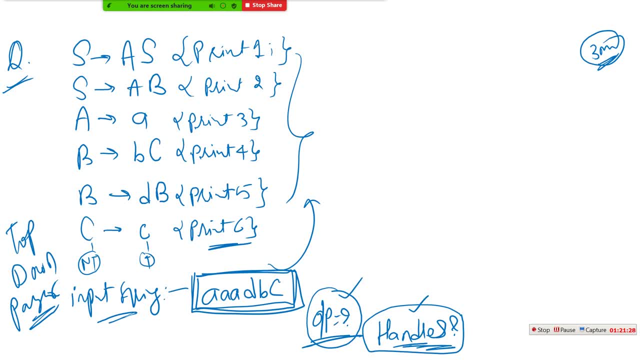 that this is the output i am getting. okay, somya has answered me four, five, two, one one while generating this. okay, i will check it out. don't worry why, when i will solve this question now, completely focus on my screen. i will solve it in detail and will answer it that why it is so and why it is so. so i am still giving one more minute to 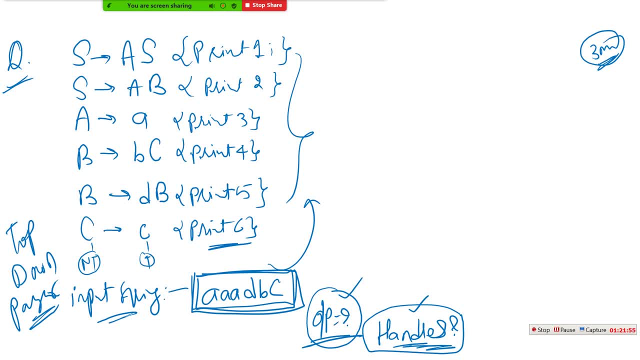 other candidates because i got only one answer. okay, yasir answered it again. okay, i got two answers. till now. both answers are different. i am still giving you time, guys. please solve it. piyush is getting answer. ankit has also answered me. actually, we need to apply top-down parsing, guys. we need to apply top-down parsing, okay. 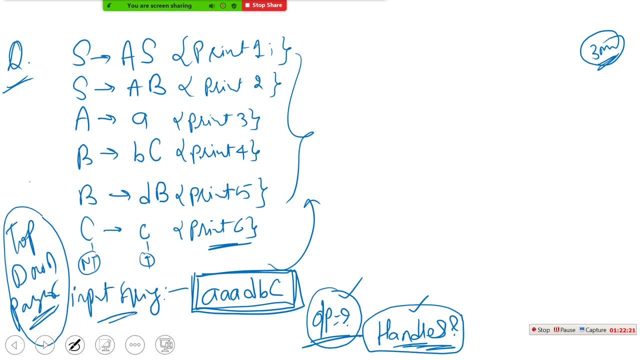 okay, okay, now let us focus here. now focus here. i am drawing this: what i need to generate? a, a, a, d, b, c. so my complete focus would be on this input string. my complete focus will be on this string because i need to generate this string using top-down parsing, as it is mentioned in the question. 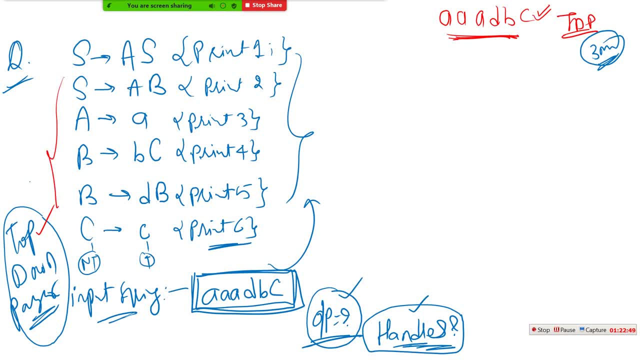 using this sdt that is combination of context-free grammar and semantic rules. so the rule number one is: always start from the starting symbol, always start from the starting symbol. so i have started it from s. so what i need is, initially i need a and i only, i can only get a from capital a. so what i will 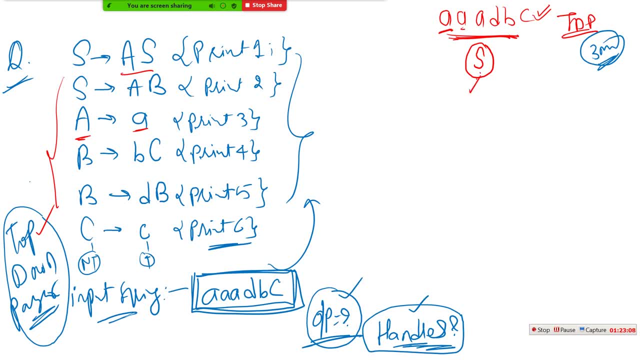 generate. i will generate a s, because i again need a, so i will. i will generate a and s here, because i again need one more a, so i will again. and after that i also again need a, so i will generate a and s here. now, after this a, i need b, i need b, so i will get this d from only b, so what i? 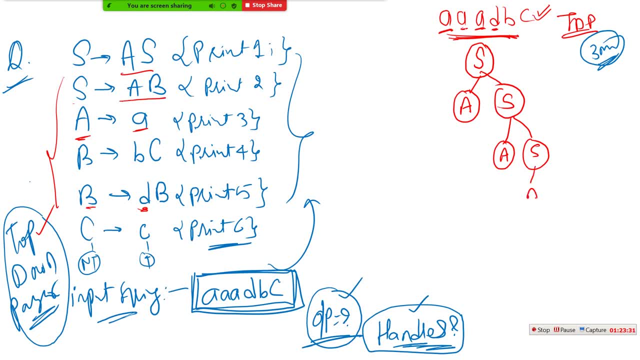 will generate. i will generate a, b now. so this s would generate a and b now, because this a will lead to me: this is small a, this a will lead to me, this is small a, and this a will lead to me. this is small a. so i got triple a. now i need d. so from this b, from with this b, i can generate b, b, because after 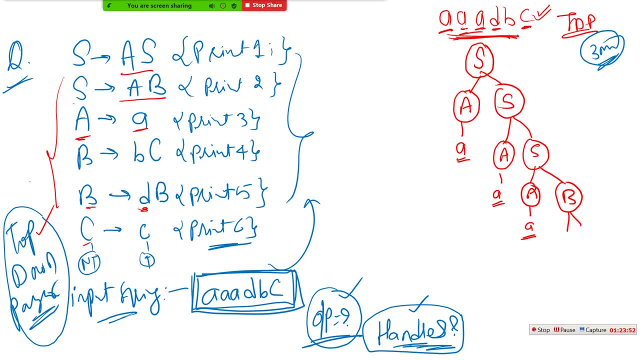 that i need c and i can get c from c, so i can generate db from that. right from this b i can get db, and that is this d and b. now i got d as well. now from this b i need bc, so is there bc directly? 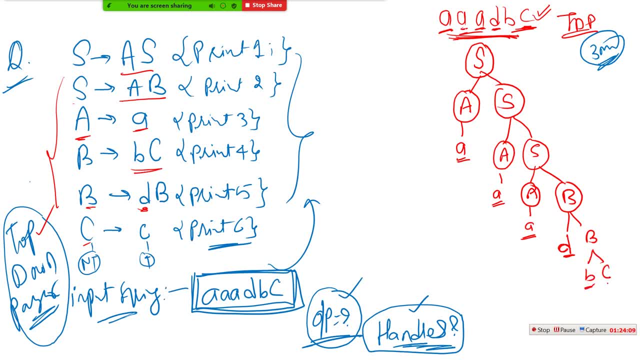 yes, i need bc. so here i have get b and this is terminal, non-terminal c, and from this c i will got this c. so triple a dbc. this is my semantic tree, this is my semantic tree, this is my semantic which i am getting, which i am getting as a top down parsing. now, if you will observe here, guys, 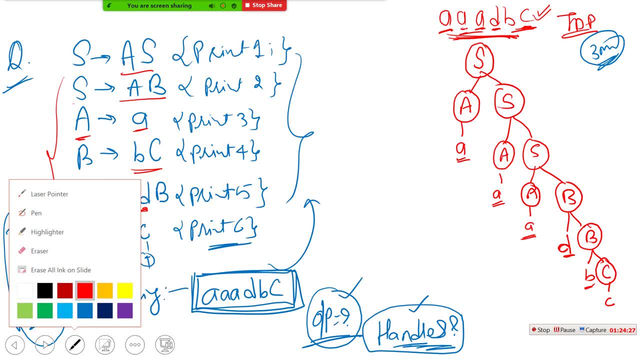 now, if you will observe here, focus on the screen now, completely focus on the screen, guys. initially i have generated this a and the value of this a is generated using this a. so what is this a? this a will generate print three. why? because this a is a. this is the transition third which is executed. 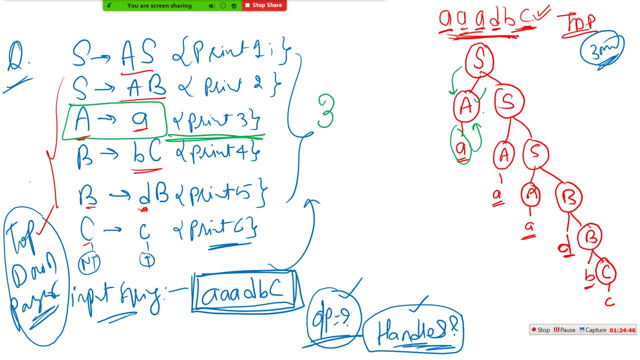 first, so it will generate three as a output. after that, if i will move, if this s is generated as, but it is not executing completely, this a is only executed and this generated three, so i have write my output three here after that. after that, after that, this s is generating this a. 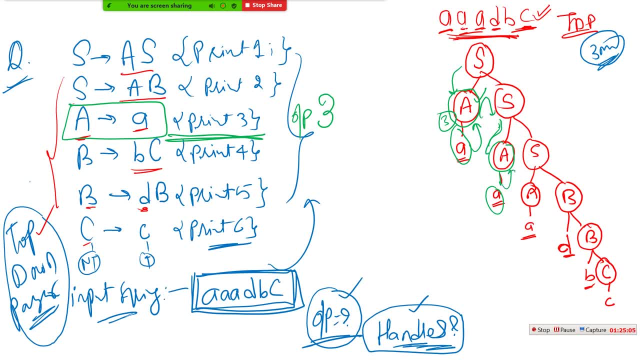 and this a is generating a. so this a is getting value of a here. so again, this is a generating a. so again i am getting capital three, that is, three, as a output. so this three is now executed. now. after that, this is: this: s is generating a and b. this a is again getting a. 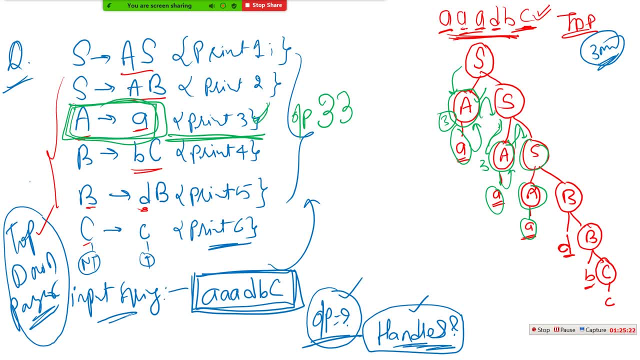 so this is a is generating a. again it will generate print 3, because whenever this s statement executed, whenever a derives, a executed, 3 will got printed on the screen. so here again, 3 got printed. so i have again write 3 here now. after that i will go to this b. this b is generating b. 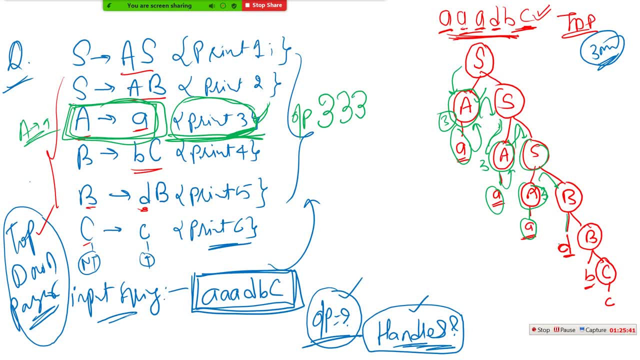 but this b is generating db. this b is generating db, but this b is not executed completely. now, this b is not executed completely because this d will B along with this B, but these bi generating BC. This C is not again completed, So this C is now generating C. 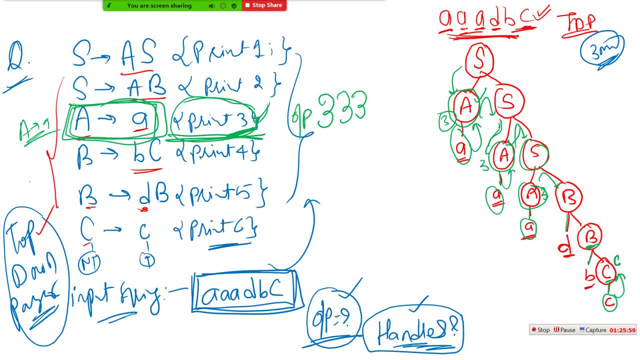 So first, when I got the values small c here, when I got value small c here, when I got value small c from this B, I can say, I can say that this C is holding value of this C, this WC is holding value of C. 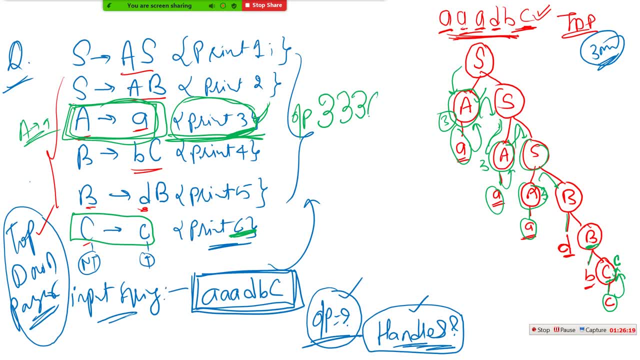 so this c is holding value of c. so now 6 will got printed on the screen. now this b will got the bc, because this capital c is holding value of this c. so this b is now holding value of c. so first this capital c will executed. after this this non-terminal b will executed. so this b derives. 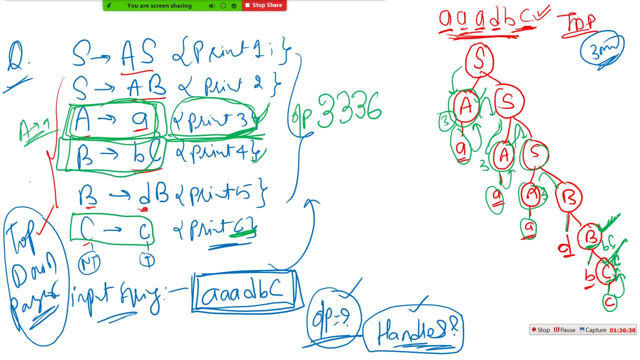 bc. this b derives bc means 4 is there, 4 is there, so now this 4 will be executed. so 4 will got print on the screen because of this b. now this b is generating value db completely, so now b derives db, that is, 5 will not. 5 will got printed because the b derives db and now 5 will got printed. 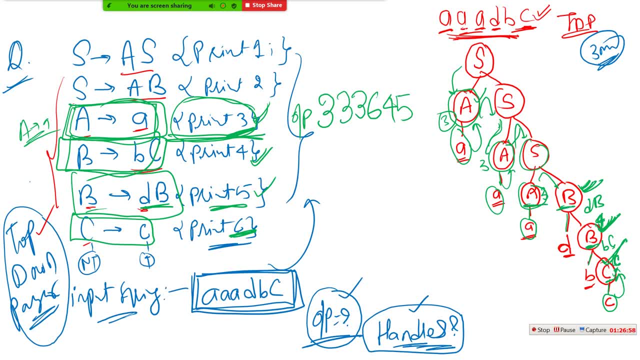 because of this b now, because of this a b, because i have value of a that is a smaller here, and i have value of this b that is db here. so, completely, with a and b, i will generate value of s. so what else is generating s is executing a b. 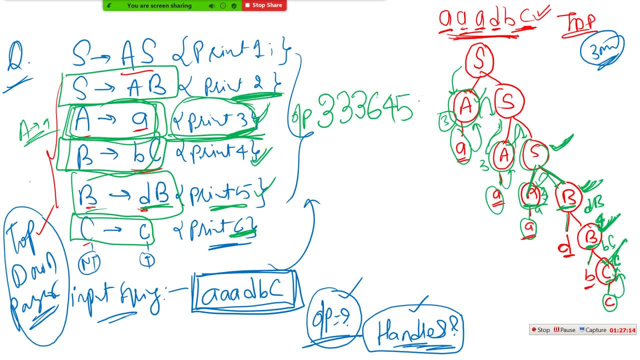 b. a, yes, is executing a- b, so print two. 2 will got printed on the screen and now i have value of a and s. so this a and s both will got printed because of this a. so a is generating as s is generating a, that is one. one will got print on the screen and after this, a is generating as this: i: 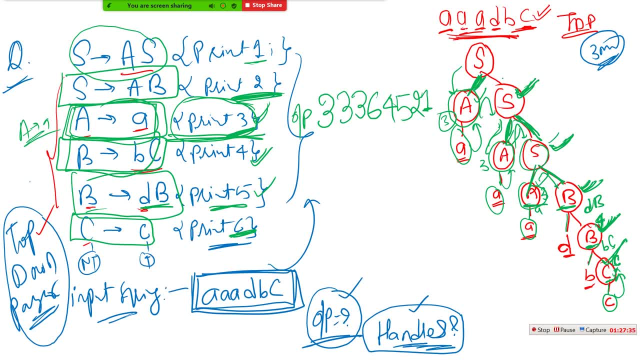 have got value of this a and further. this s have value of this a and s. so after generating this s, that is one again generated, as that is one will got printed. so output that will gonna print on the screen is triple, three, six, four, five, two, one, one. it is the output. guys, it is the exact output. 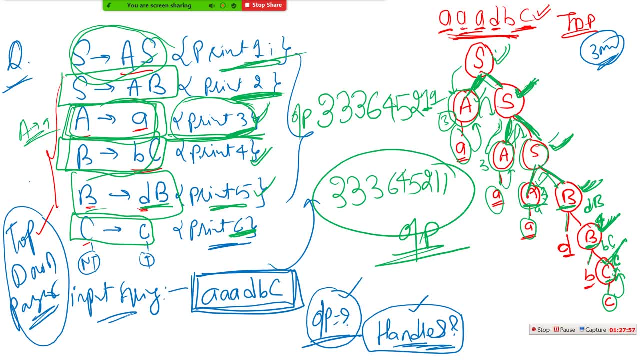 according to isros solution. so, guys, is it clear to everybody that how this output come, how this output come, is it clear to everybody? is it clear to everybody that how this output come? please answer me, because this is very important concept and if you have got that means now you 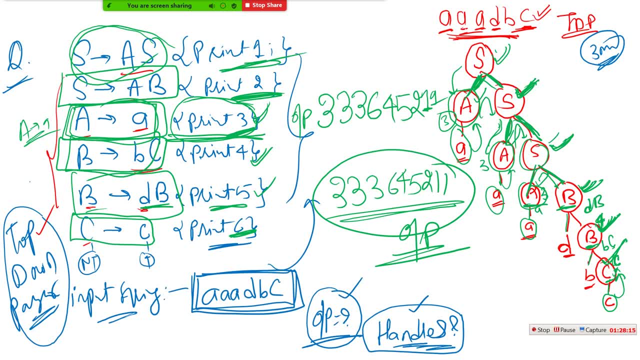 are getting pesa 4 sdt in its problems. clear now, guys, that white triple three, six, four, five, two, double one is answer. very good guys, very good, clear to everybody. very good now, if i talk about handles, if i talk about handles now, if i talk about handles, then observe here: first i have 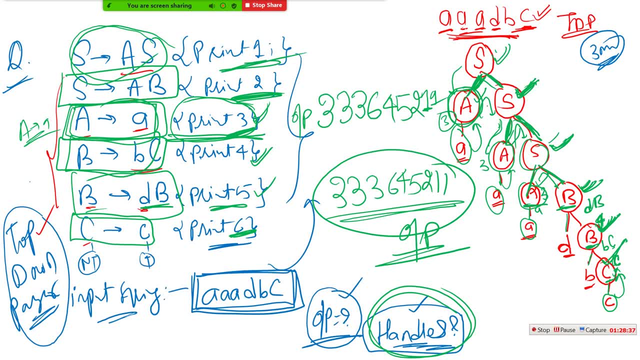 executed is. this is so how many handles? basically, i am getting a derives a one handle here. okay, i am changing my color so that you can got the answer. okay, sorry, i am making it highlighter. this is the one of the handle. guys, just two seconds. this is one of the handle. this is second handle. okay, this is third. 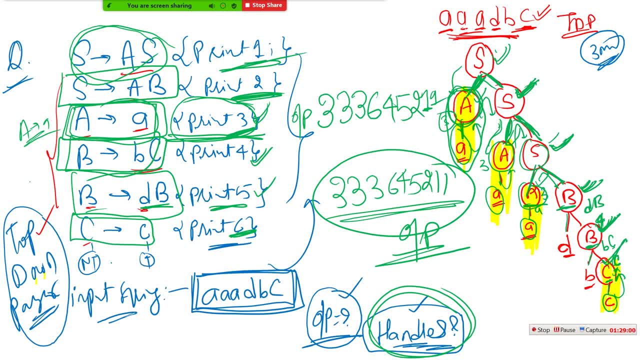 handle. this is fourth handle, this is fifth handle, that is this one, this is sixth handle, this is seventh handle, this is eighth handle and this is ninth handle. so, guys, you can verify it. you can verify it now, when we have sold, when we have sold earlier, as 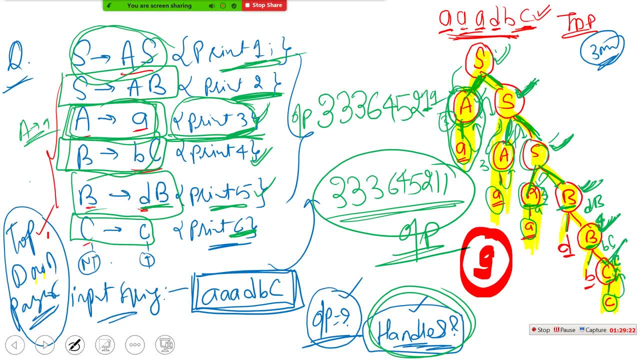 well, when we have sold it earlier as well, when i give you problem in before syntax analyzer now, at that time we also answered it that nine handles we are facing, we are getting nine handles. so i hope now it is clear that why my nine handles are there. this is the process of compiler design. i. 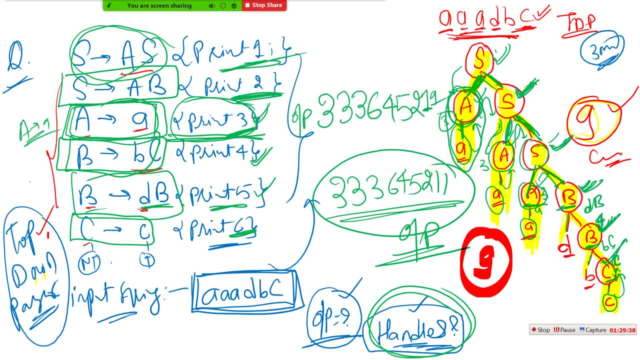 you are getting compiler design in detail. nine handles are the right. yes, handles will not gonna change. whether you do top-down parsing or bottom-up parsing, handle will remain same, dear. yes, handle will remain same whether you do top-down parsing or bottom-up parsing. in bottom-up parsing, there will always be. 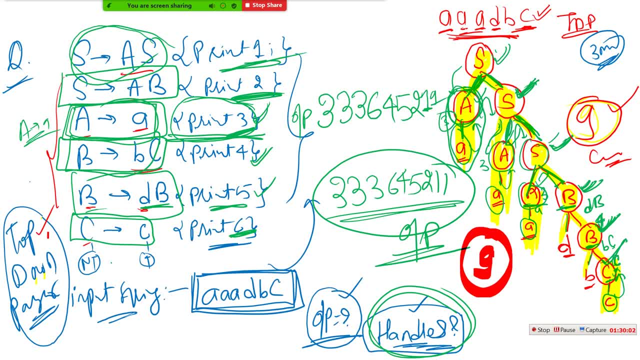 nine handles in top-down parsing. it will go nothing. it will not gonna change. okay, guys, is it clear. is it clear? okay guys, break yes. what you are answered, yes, yes is saying oh, yes, if you will do bottom-up parsing, definitely output gonna change. if I said that bottom-up parser, then in bottom-up parser, this is. 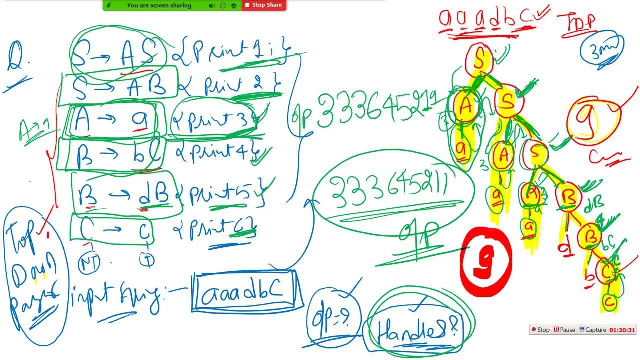 executed first or whatever is executing according to that handle. with respect to that handle, you can answer that didn't change this printer is the answer. okay? so okay, don't worry. don't worry guys, don't worry, this is the answer that this is. the answer which I am getting is a top-down. 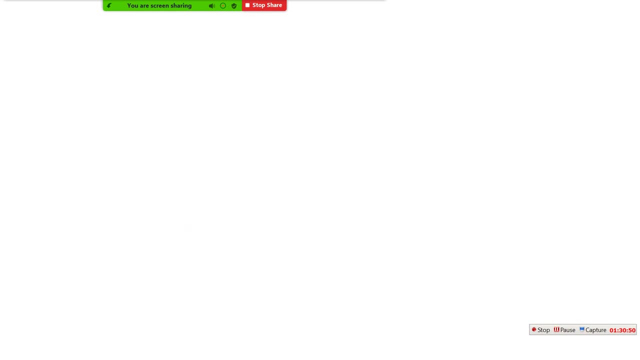 parser now, because of yes problem, I, yes, prop, yes- has asked one more problem: that what if we do bottom-up parsing in the same handle? my string will remain same: triple a DBC. okay guys, do you need break? do you need break? after 5 minute we can discuss the bottom of parsing on this in. 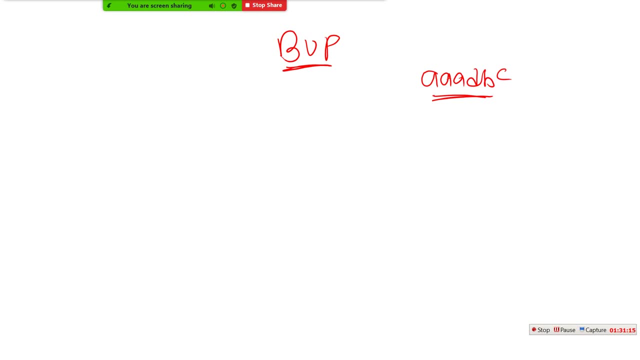 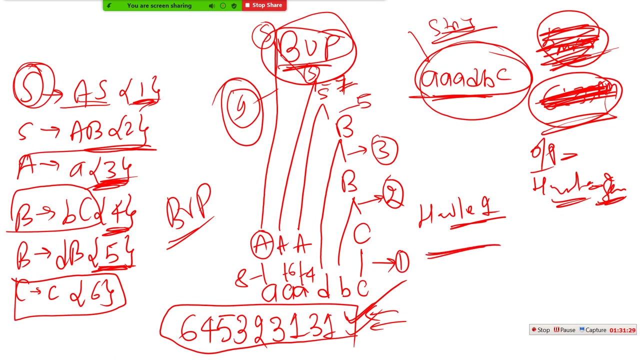 do you need break or should I continue with that? after that, we can take break. after discussing this bottom of parsing, we can take break this, or you need break now. please answer me. you need break now. okay, so it is my answer. it is my answer. it is my answer while traversing the bottom of parsing for the same same. 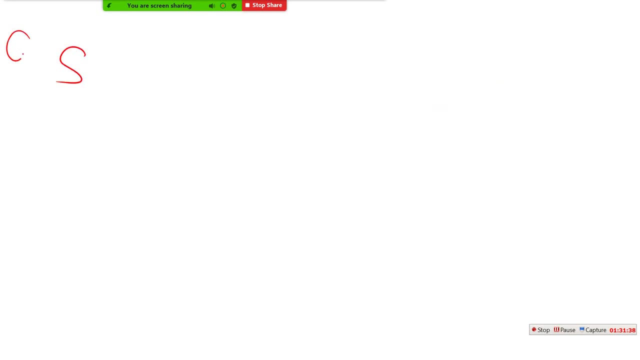 problem right now. next question in front of you is the question is asked in bark exam and the question is: as derives a, a as derives a and as derives, what is there as derives? okay, a is deriving, a is deriving sb and input is here. is it will print one in semantic rule? it will print one. 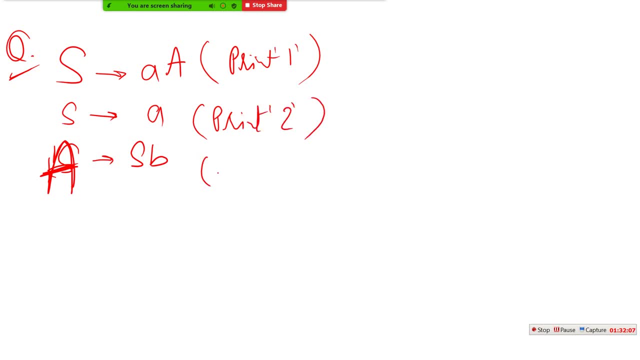 it will print two. it will print three. my input string is a, a, b. you need to apply bottom-up parsing. question is: you need to apply bottom-up parsing using bottom-up parsing. what will be the output, guys? what would be the output applying bottom-up parsing? please answer me just one minute question. it is very. 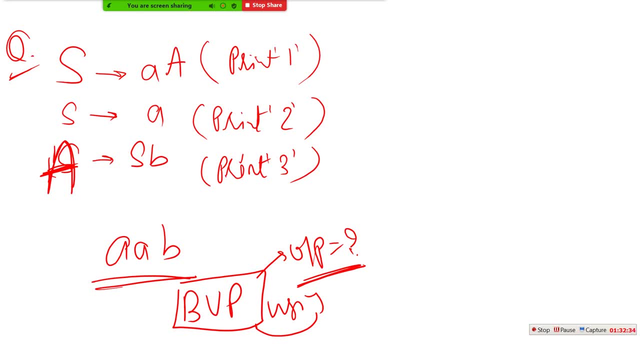 simplest question. one minute question. what would be the output of the following program pro program using bottom-up parsing? simplest program in gate any bark exam, it is the gate problem which is later asked by bark master. if a problem is solved which is later in, out your or Parts unitclock, what is it called? answer me this problem 2311. ok, I will check it out. 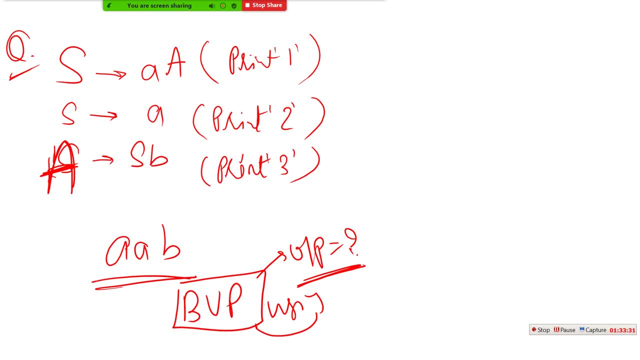 while doing: while doing bottom-up parsing unit to answer. while doing Instagram of parsing unit to answer. please answer other candidate. I am requesting from other candidates as well. please answer other candidate. I am requesting from other candidates as well: them two, three, one one. I got answer from two candidates expecting other candidates as well. 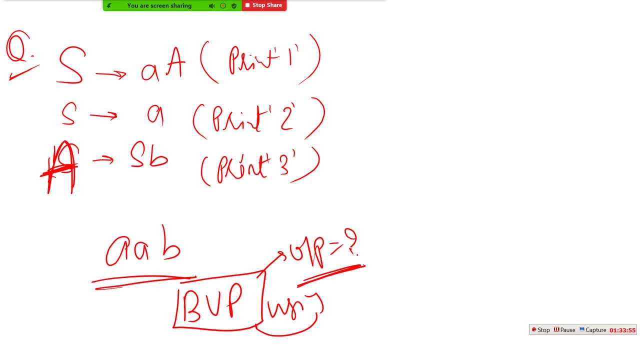 please answer. I only have my input string as a a a B. a a B is my input string, guys. Walsh, Ali is getting 2, 1, 3, so may is getting 2, 3, 2, 1. Oh, many answers are there, guys? I am. 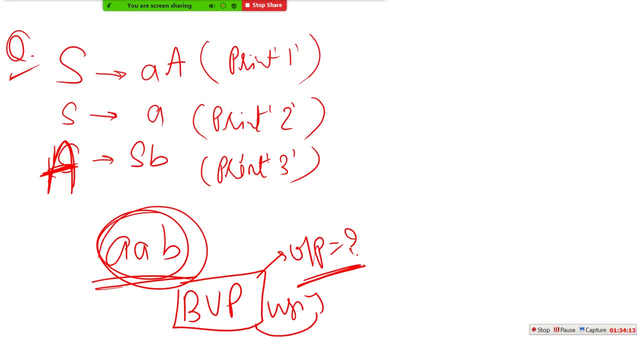 getting much answers. where it is of unfair, I am getting. why don't you forget? why don't all of you are giving me unique answer? I got many answers. I got many answers. okay, let it check it. now. I'm discussing the solutions a, b guys. it is my string. it is my string, guys. now let let focus here. i need to apply bottom-up. 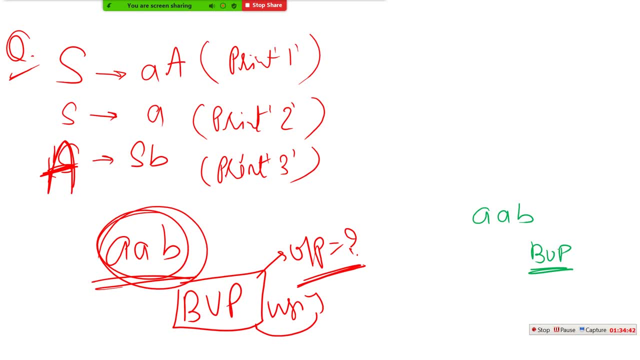 parsing, i need to apply bottom-up parsing. using bottom-up parsing, can i generate alone b? this alone b cannot be generated from anyone, from anyone. this alone a cannot be generated, cannot be generated. that is why i will go further, one step ahead. in that case, i can generate this a. 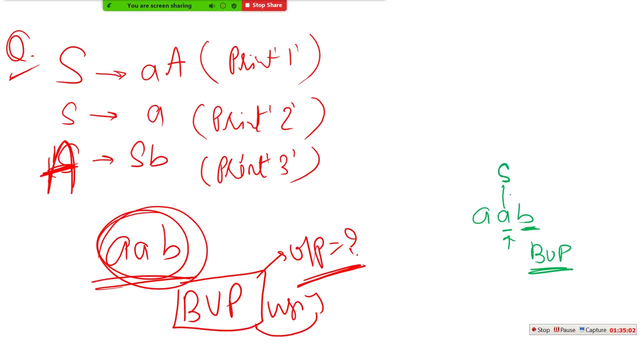 i can generate this a with this a. so this a i am generating with the second transition is so what i will get output. my output will look like: two is on my screen. my two is now on my screen as a output because of this transition, because of this transition after that, after that, after that. 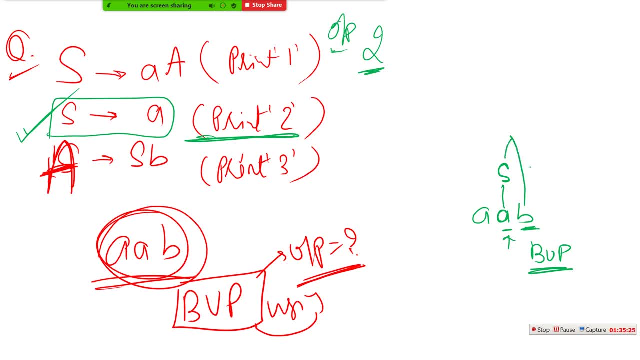 what i am getting. this s and b will be lead to a. this s and b- that is, a- is leading to this a and b because again i need to start from rightmost side now. so again i am getting a and b and it will gonna print three for me. it will gonna print three for me because it is. 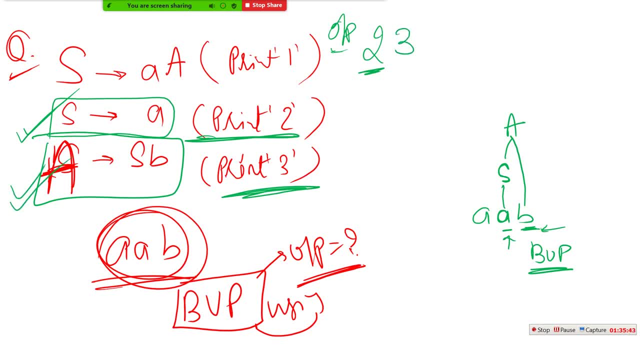 third transition, so it is gonna print three for me what i am left with. i am left with a and a. now, this a and a i will got from this s, so this s is generating this a and a. so what transition it is? it is first transition, so it will gonna print one, so i got my starting symbol. 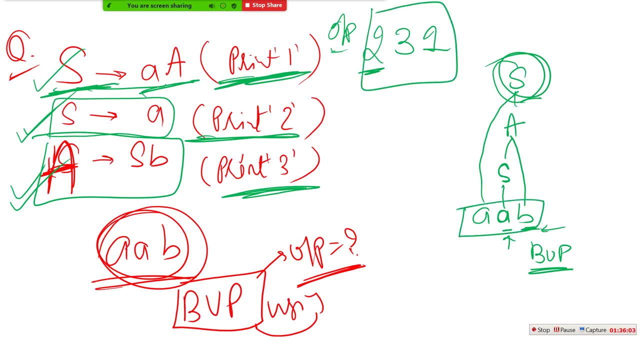 and i traversed completely my input string so i got output two, three, one. now i am asking that whether double one you are getting guys, where extra one you are getting nikhil and manjit and yash, where do you get one extra one? because i only got two, three, one and it is the correct answer. 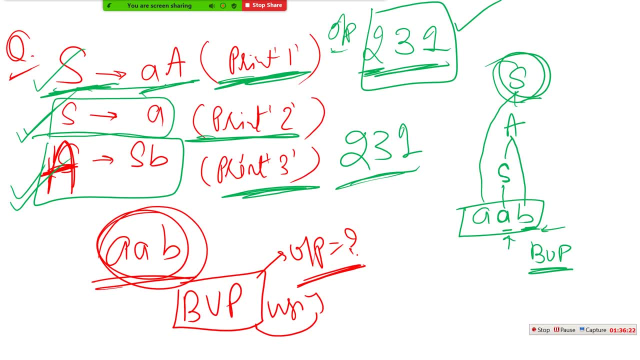 according to the gate keys: two, three, one is the correct answer using bottom up parsing: guys. okay, two, three, one is the right answer. is it? is it clear to every candidate? is it clear to every candidate? guys, this problem is clear to every candidate. please answer me. please answer me. is it clear to every candidate? okay, it is clear to every candidate. very good guys. 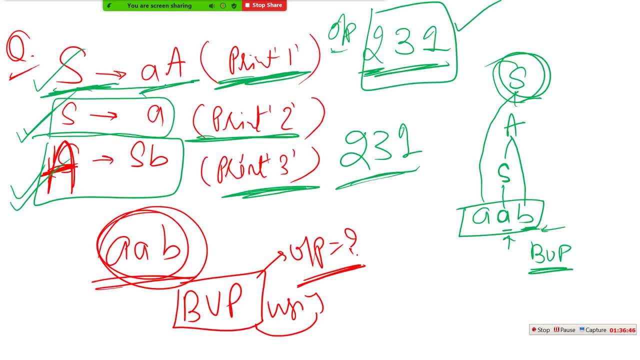 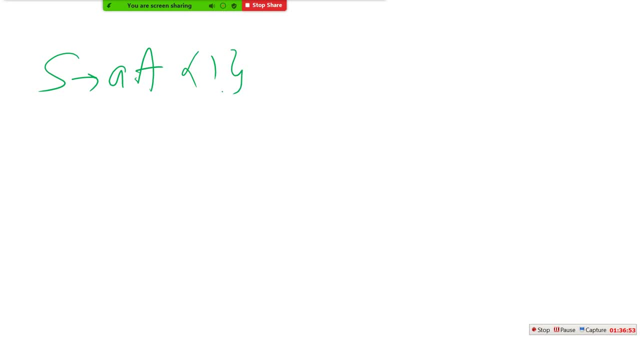 okay, no problem. now, what guys? what guys, if i say i, if i say the same problem, if i say the same problem, a, a, it will gonna print one, and s derives a, it will gonna print two, and a s, b, it will gonna print three? what if i will say again: you need to traverse the screen. a, a, b. 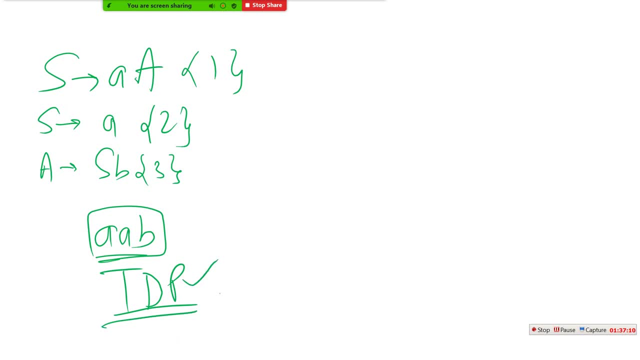 using top down parsing now. using top down parsing now. what will be output? now, answer me now. what would what would be the output? answer me, guys. answer me what would be the output. i am giving you one more minute. please answer me what would be the output using top down passing. 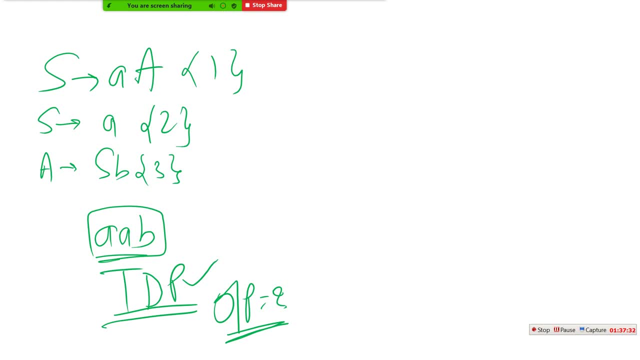 so, so, so. so what would be the answer, guys, if you will parse this tree using top-down parsing? top-down parsing, if I will apply top-down parsing, what would be my answer, guys, for the same problem? I am asking to all candidates. only two answers I got, yet I am asking all candidates: please answer it. 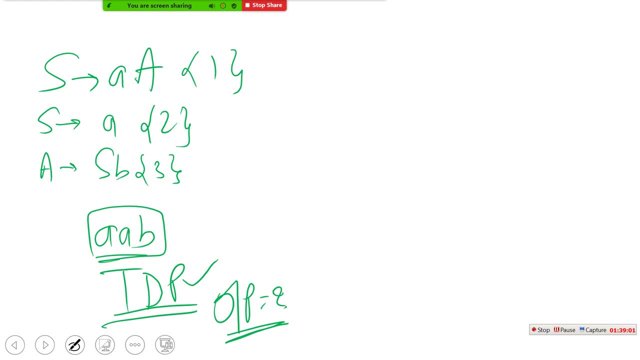 fast only two answer. I got what would be my output. let's please answer it fast way. okay, age, it is also on special, ok. so, guys, let us see here: my string is a, a, B, now what my target is. I need to generate a first, after that a in, then B. so I will always start from a starting symbol. 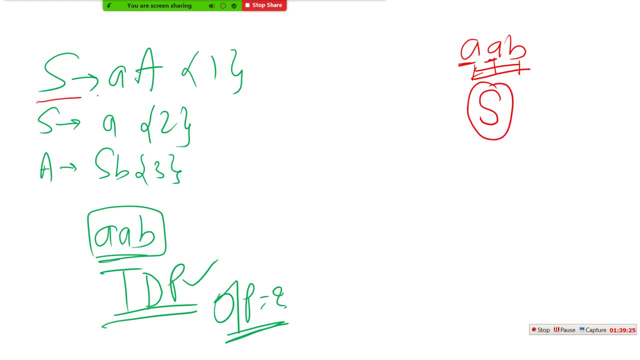 atop down parser I am doing after that I need a, so I will do this transition. so I will tell you the solutions today. you just press A, then press next two buttons and press: take this a and this a as a part of syntax tree and this a will further generate as b, because i 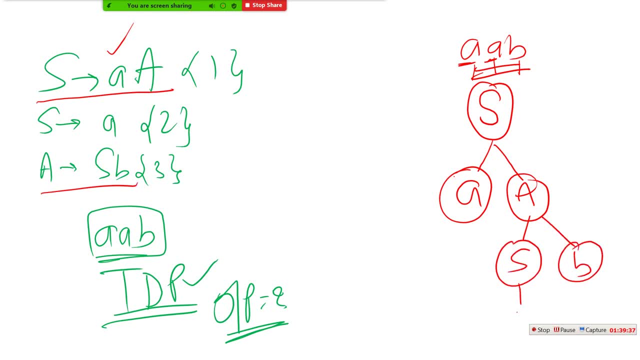 need one more s. so this hv is there and this a will generate a. so i will go to a, a and b. right, but when i will traverse this? now, when i will gonna traverse this, i will start it from here and i go directly as derive a transition. so you will say, say, sir, two is the output. but no guys. 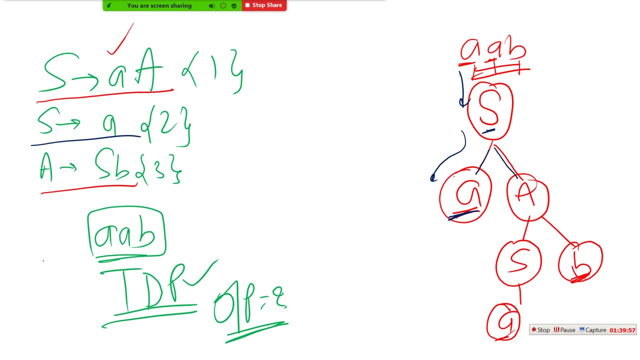 this s is generating this a and a combinedly. this is not generating this a in as a lonely right. this is not a complete transition. the complete transition of this a is when it will get complete output of a. so you need to traverse it from here to here, from a to. you are getting s.